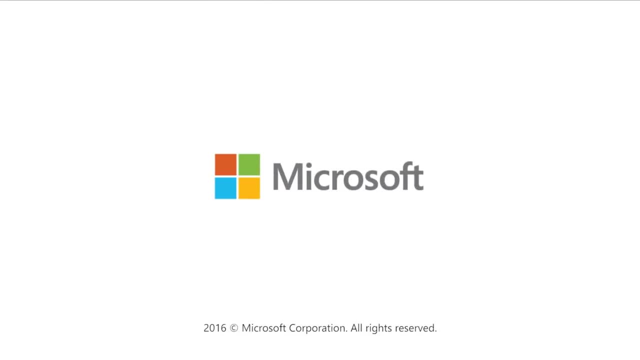 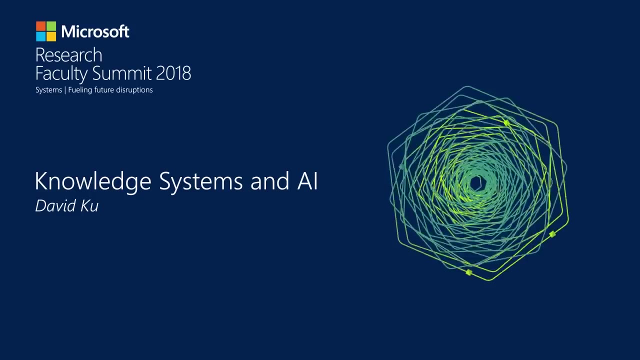 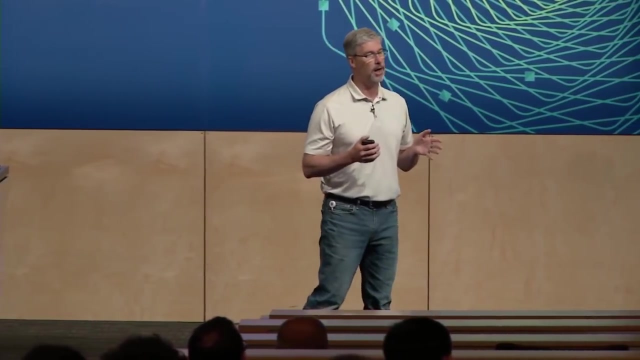 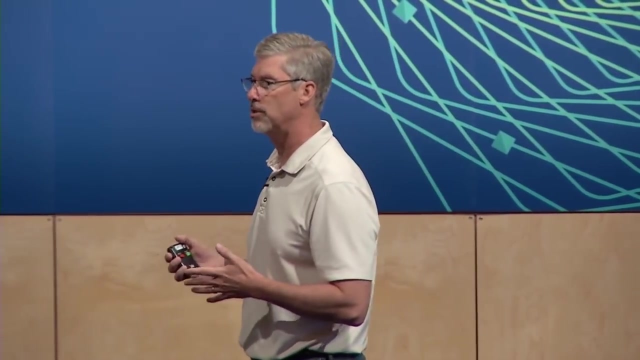 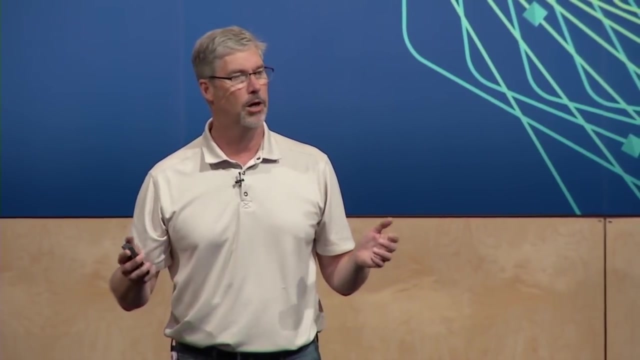 I am excited to introduce our next speaker. Our theme has been how systems are fueling future disruptions. Yesterday we had Mark Russinovich come in as the CTO of our Azure business to give you a view of how systems is impacting our cloud business. Today we 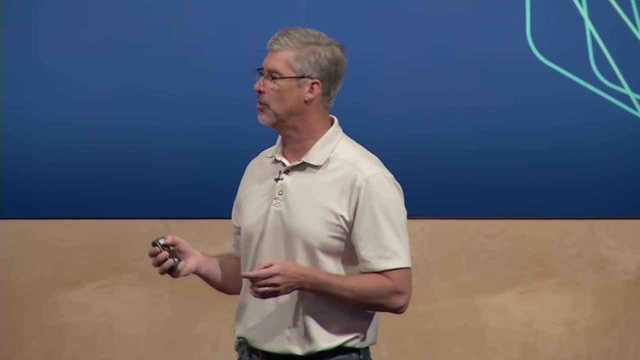 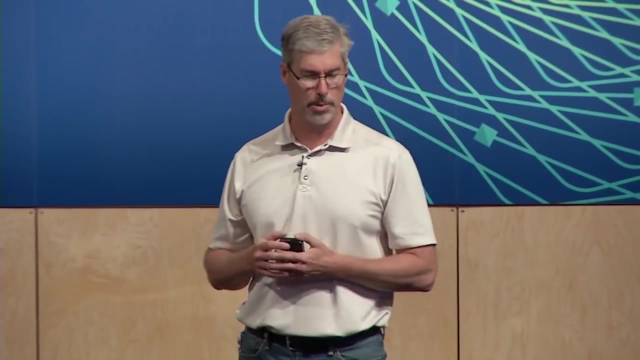 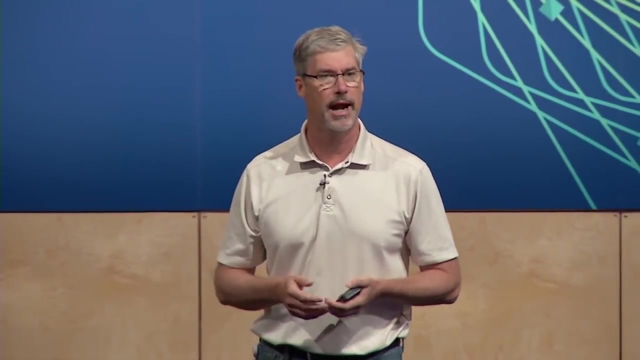 have the CTO from our AI and research group coming in, David Koo. David is also the corporate vice president for our AI core business. This is the group that powers the AI capabilities behind Bing, Cortana, Office and Azure. It's the group that designs, develops and deploys. 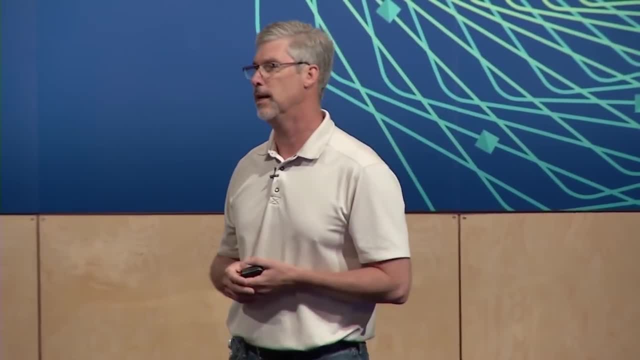 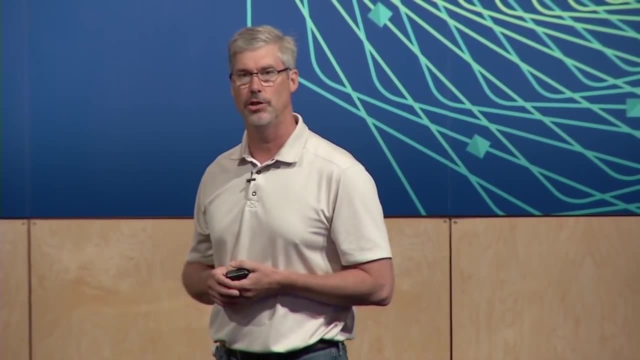 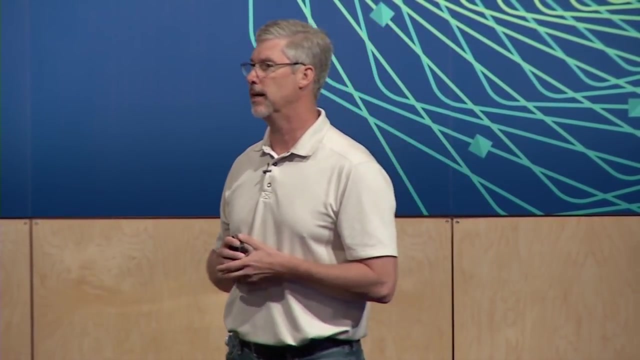 the Bing Graph, the Bing Ads Marketplace, the Office Knowledge Graph and Substrate. David's always been a big supporter of research as well and our engagement with academia. He's the executive sponsor for our relationship with Stanford and is very engaged with a number 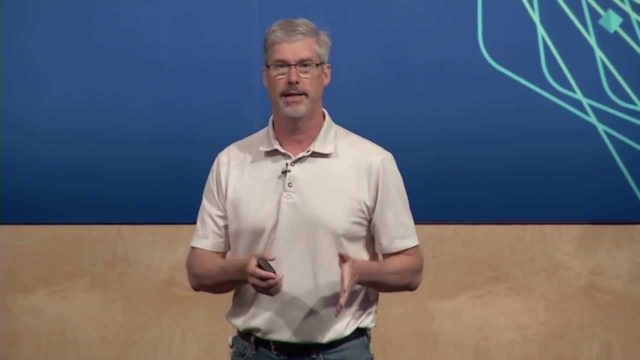 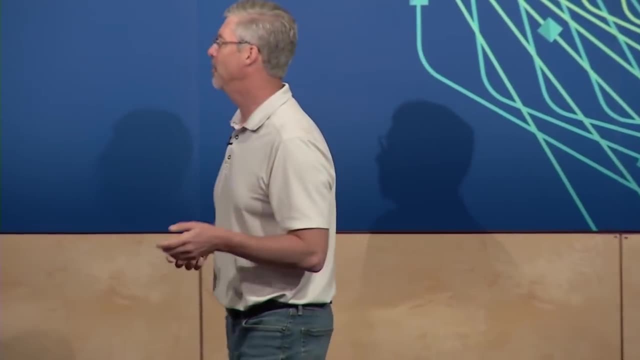 of communities from an entrepreneurship standpoint, in connecting high-tech communities into the Silicon Valley, And he's an all-around good guy. So with that, let me introduce David Koo. All right, thank you, I'm an all-around good guy. Well, good morning, I'm very excited. 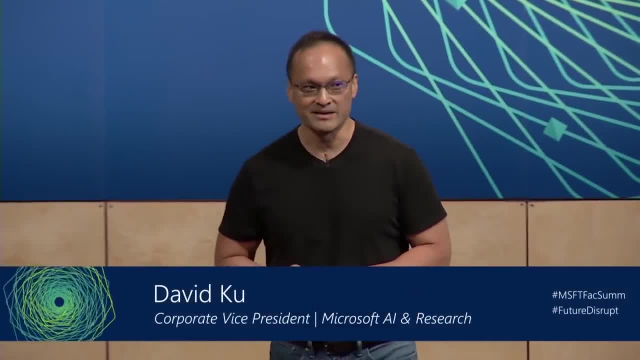 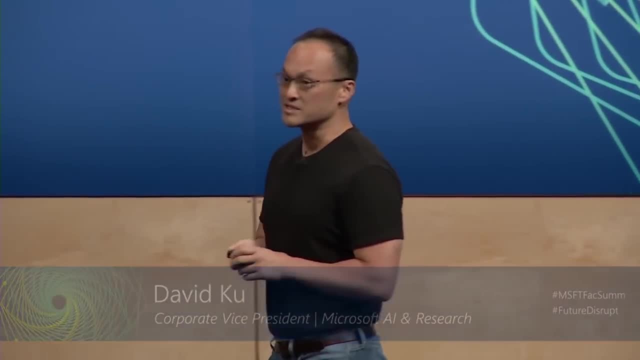 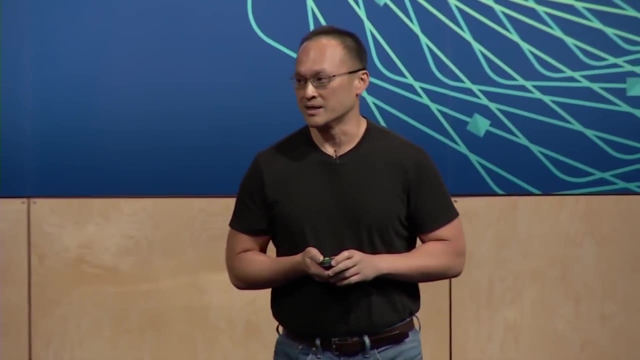 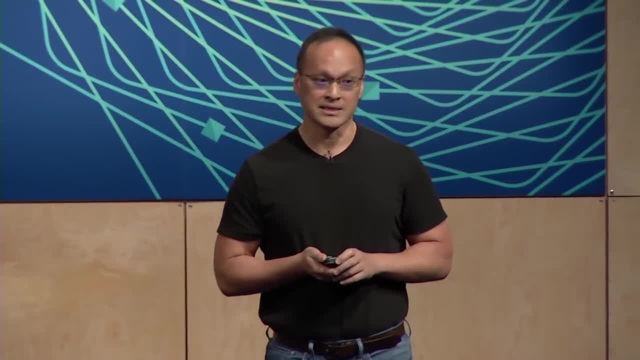 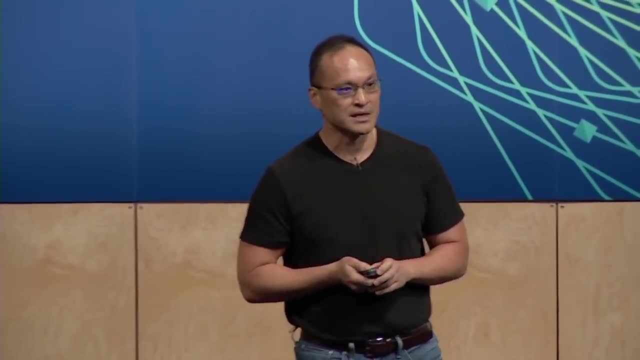 a great experience for us, And I think it's going to be a great experience for us to be invested in research in academia. I think it's a blessing And I'm certainly honored to be here, And what I want to do is I want to focus the theme on knowledge Now. this is from: 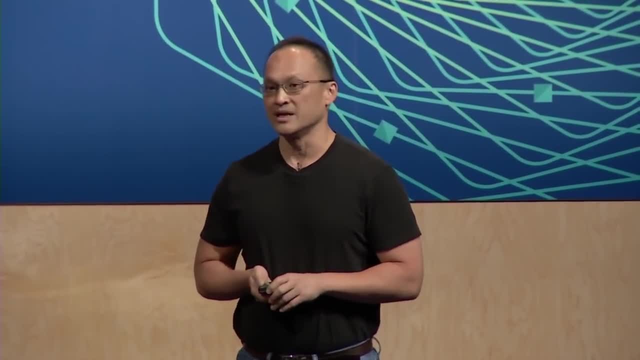 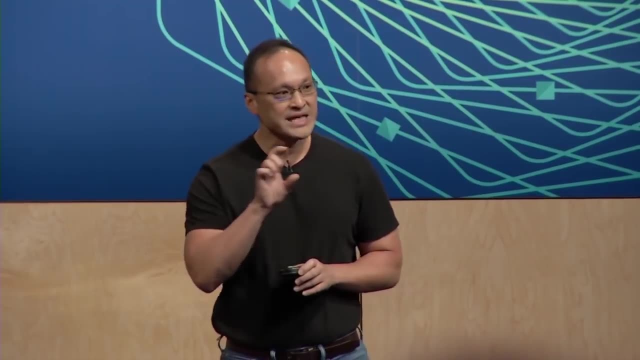 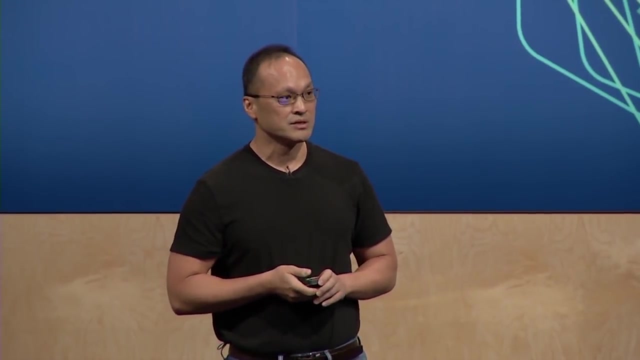 my experience in working in search in advertising. as Sandy said, in Office productivity Azure, There's a theme which is around the ability to semantically model, and we just call that broad lead knowledge, And I want to share a little bit of the journey, But also 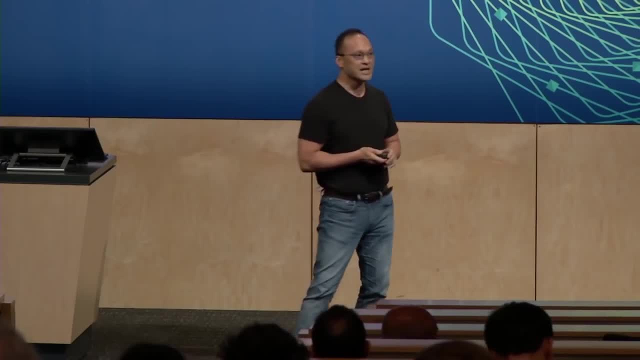 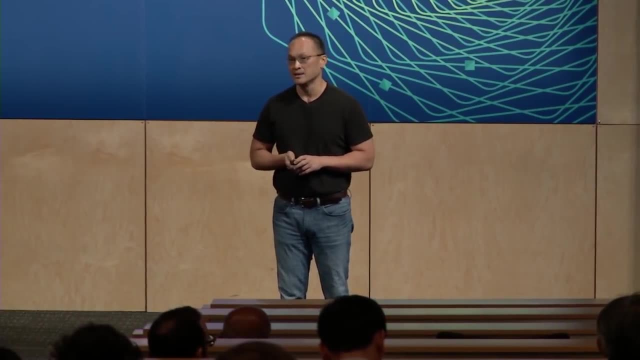 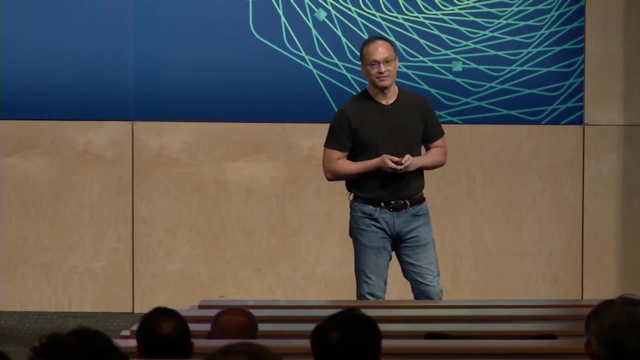 So encourage and hopefully frame that for AI transformations, both with the business impact and in terms of experience impact. I personally think knowledge is one of the core capabilities and it's a rich area for which we're still at the beginning of understanding, So I enlist all your creativity to help us make advances in this area. 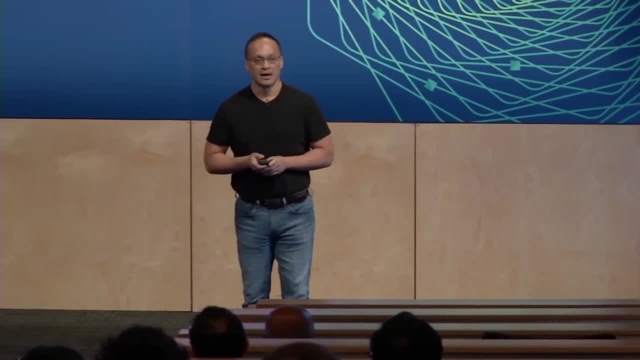 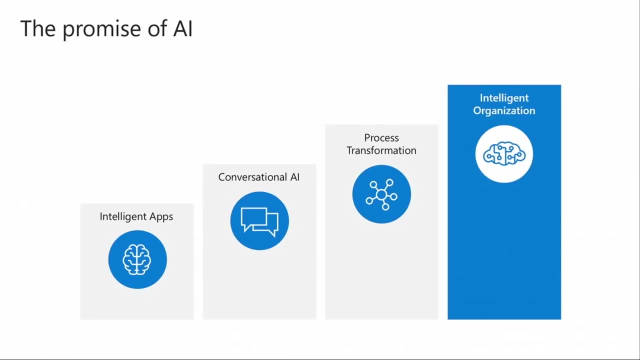 So let me start out by just talking a little bit about the promise of AI. So there's a number that comes up which is $1.2 trillion. That's trillion with a T, And that's the estimate that IDC has of the new incremental revenue that's going to be created in three years with AI. 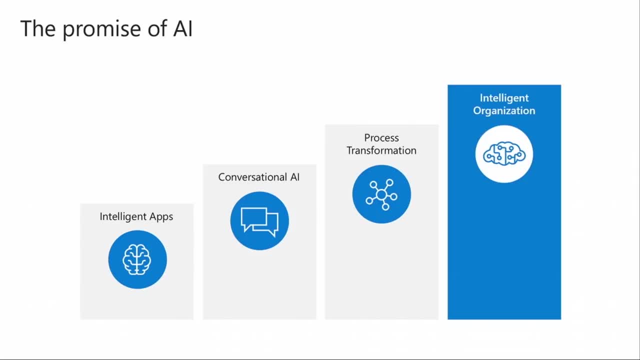 Now to do that and for this optimism to really come forth. there's really this belief that there is unlocked potential in the data assets within an enterprise or within a company that they can bring to bear to gain new insights and to change the way they interact with customers and to grow their business. 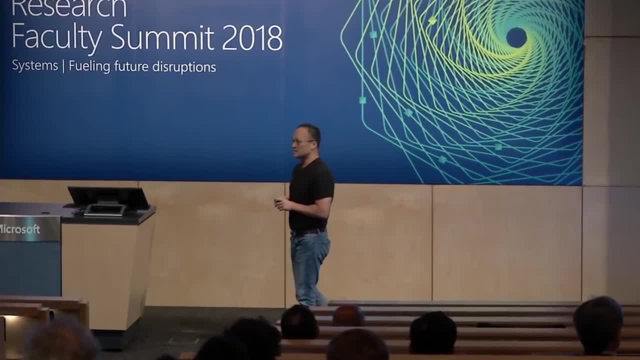 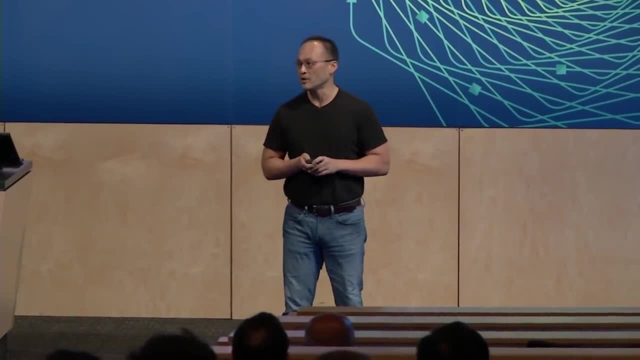 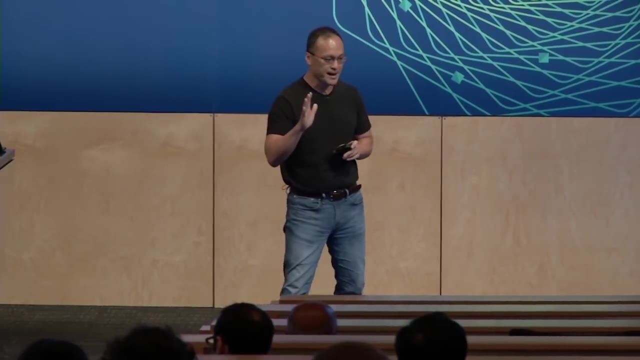 So that's a massive, massive expectation In the context of our engagements with enterprises that are looking to tap into the cloud, tap into AI in their desire to transform themselves. we've seen a pattern, And I want to list out the pattern of what they're looking for in their progression of platform. 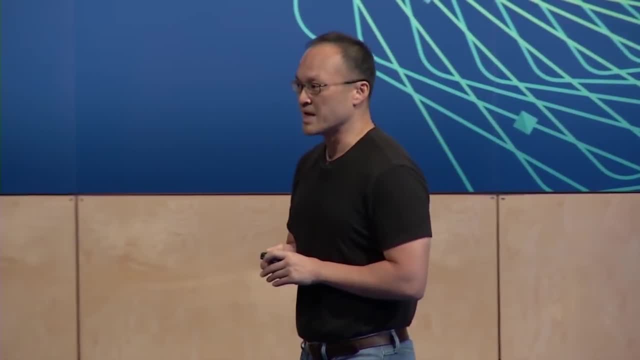 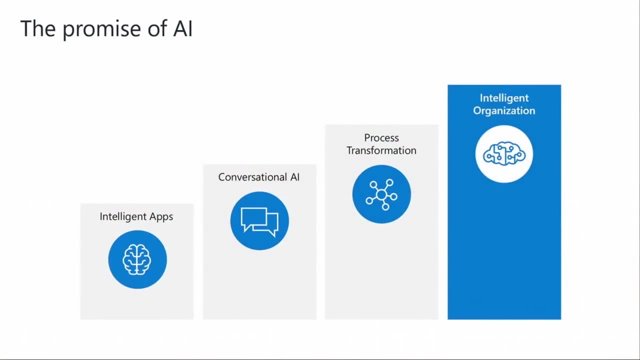 So we've got the AI in their business. So we're looking for a platform that's going to be able to take applications, point of sale, specific line of business, applications productivity and make that intelligent, feedback-driven, predictive analytical. 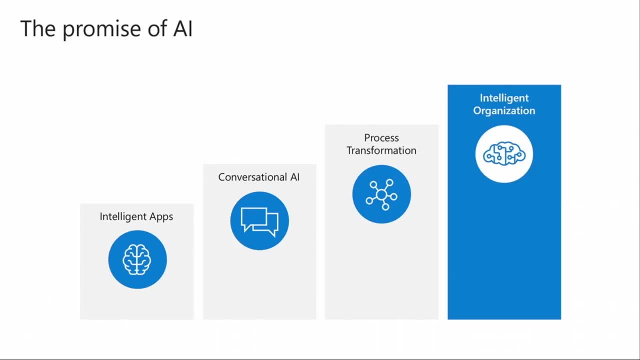 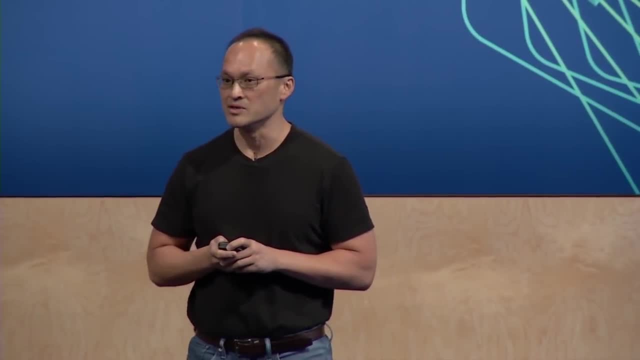 But beyond this, there's also this desire to use AI to change the way they interact with people, And that could be employees or that could be customers. And this is the wave of conversational AI where it's not just any set menu or interaction metaphor. 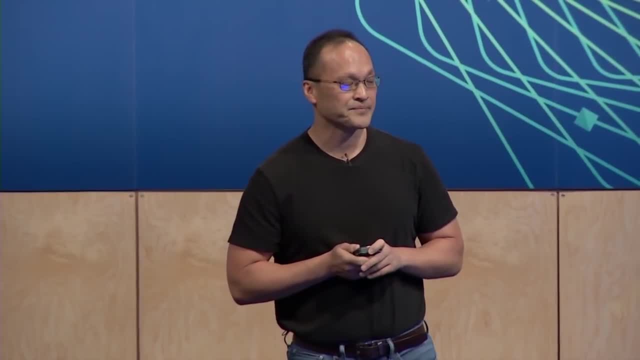 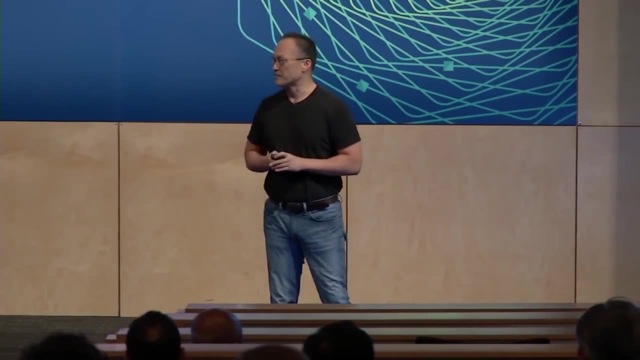 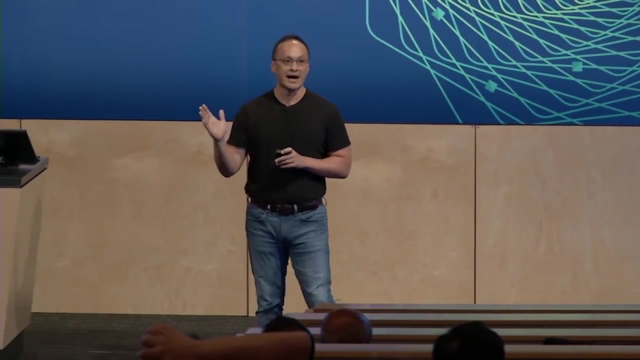 It's really just this language as the interaction metaphor And that, again, we're still at the early stages of exploring that trend. And then there's process transformation, like being able to understand- not just analytically, retrospectively- the difference between BI and AIs. 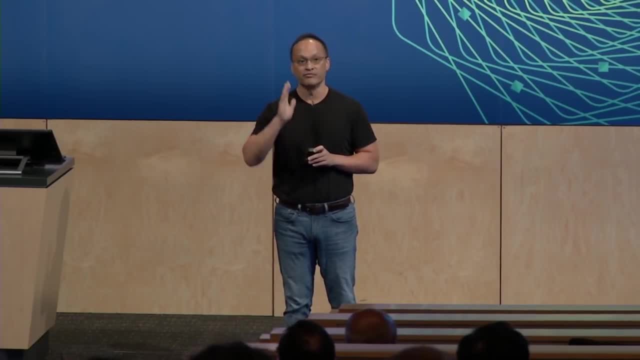 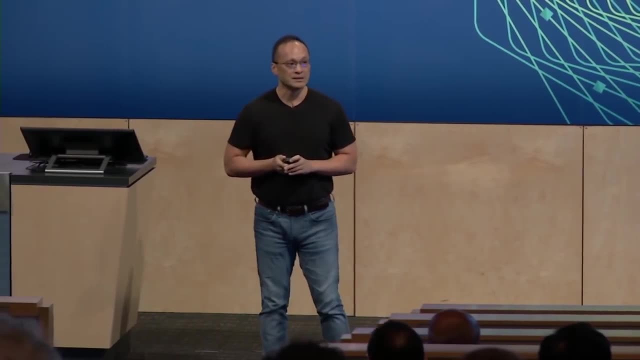 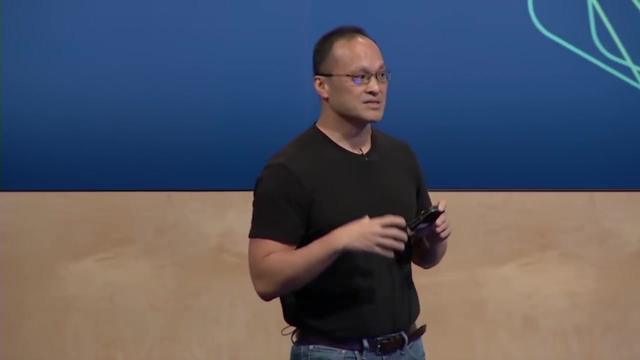 and, in some sense, the ability to predict, anticipate and optimize, going forward, not just looking backwards. And then a general desire that the transformation of a company is complete when every aspect of the system of the company is somehow modeled that allows us to reason, optimize and to drive. 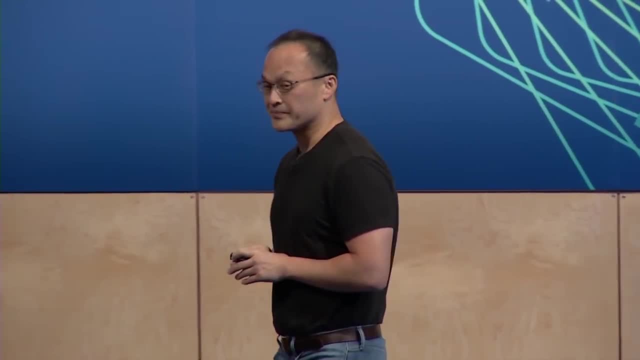 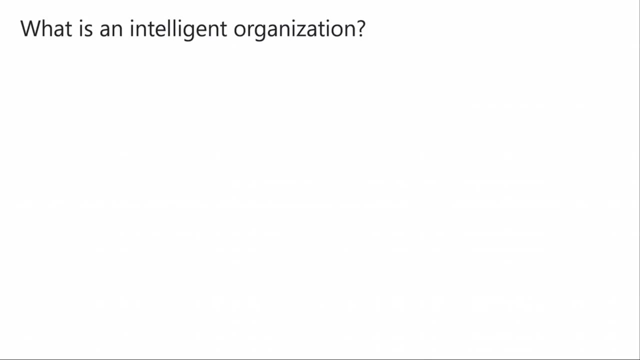 And so that wave of business value requires a company to really deeply look at what it takes to be an intelligent organization. So let's dig into it a little bit. You know, it's no doubt that the first, the first step to becoming an intelligent organization, 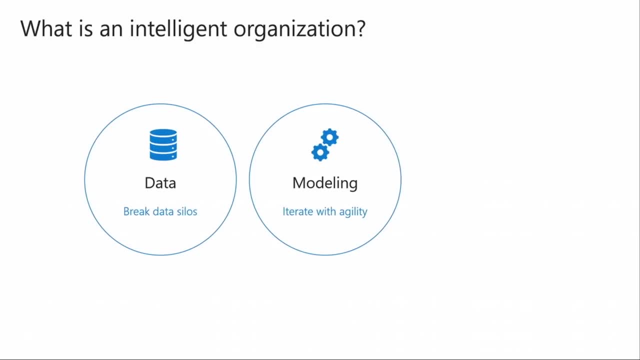 or for a company to be effectively embracing AI is to start with the data. Start with the data. unsilo it In many, many companies, starting with product companies, but also enterprise companies. they need to start to now look at untapping the value of their data. 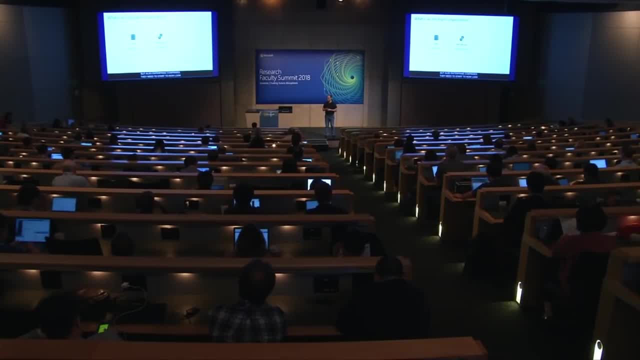 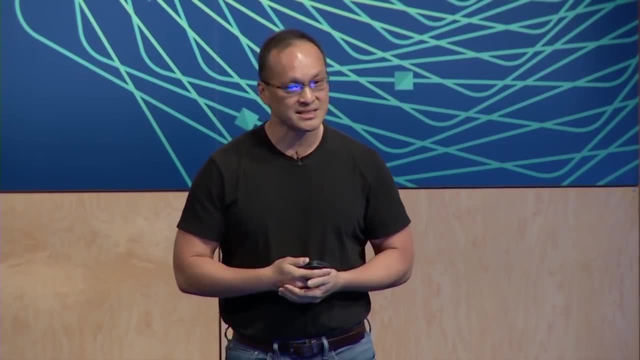 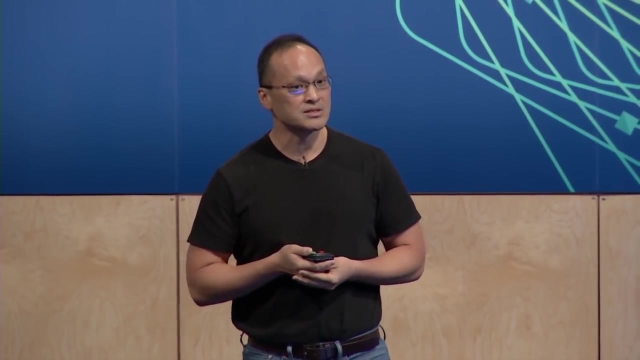 So lots of work in understanding the quality of the data, being able to connect to all the pulses and the inputs, both in terms of real interaction with the customers and internal processes and interactions, And to be able to have the ability to model, And that requires us to really have a foundation for rapid iterations. 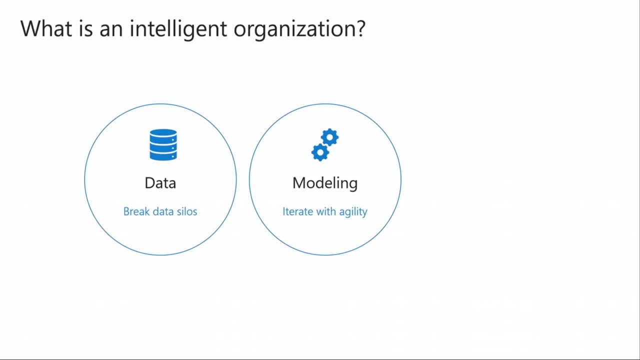 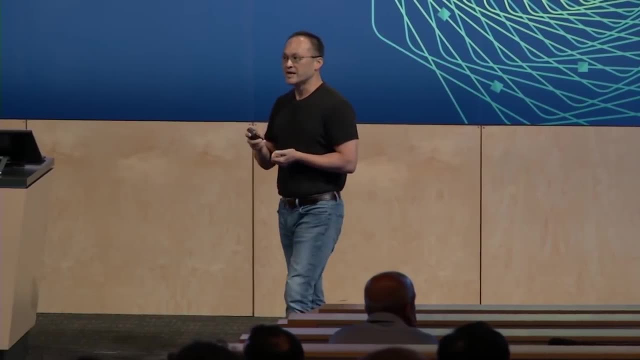 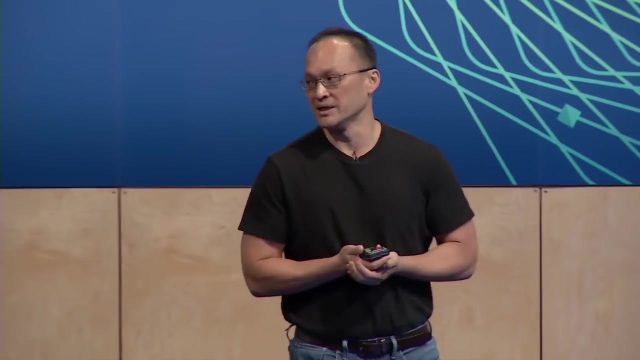 experimentation with all sorts of different modeling techniques, And so this modeling agility, with the ability to unsilo data, are table stakes. But when you start looking at what it takes for a company to truly embrace AI, I would posit that there is a third phase, which is the ability. 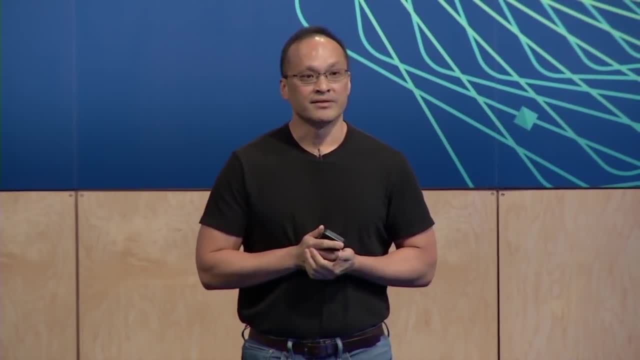 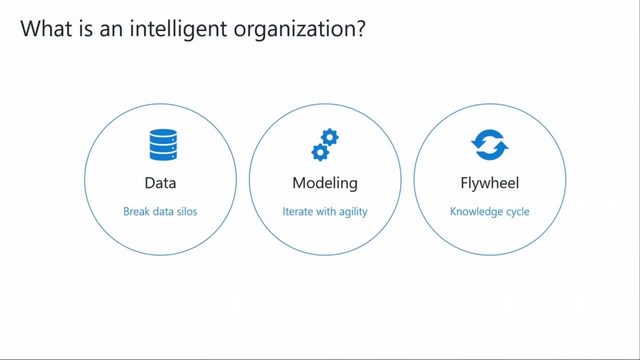 to start with the data, To start shifting the mindset, that data is in fact at the core, That there's a flywheel where everything evolves around, not the existing interaction with the customers, but in fact there's a knowledge, there's a model of the business. 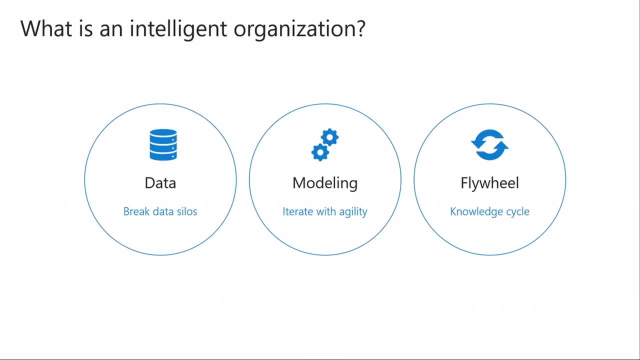 for which even software and experiences are there to help us understand that data and model better, as opposed to the other way around, And that requires a really fundamental thinking of what is the core asset of a company. Now, when you look at all this, 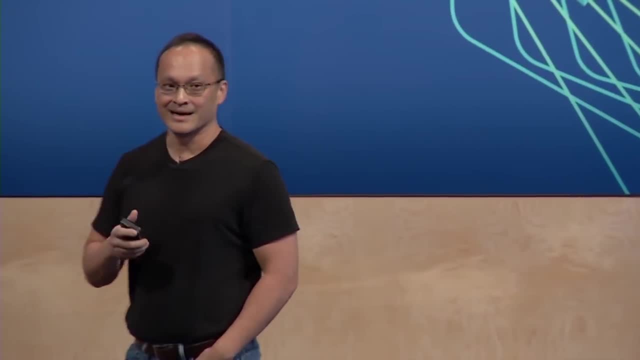 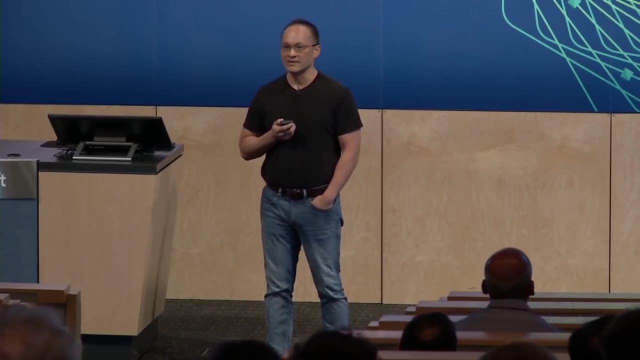 and you say, hey, this seems fairly abstract, And how do we bring this to life? Is this really something that happens in practice? I want to share a little bit of the journey that we went through at Microsoft, And certainly we're not alone. 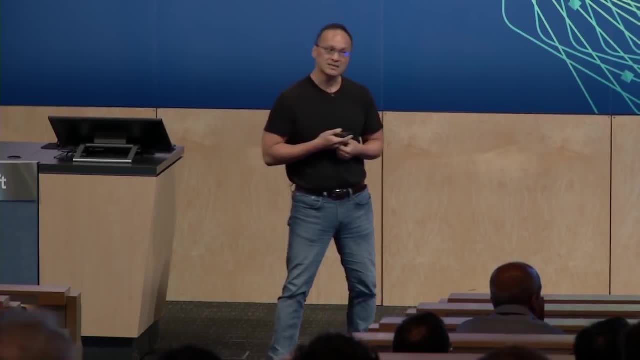 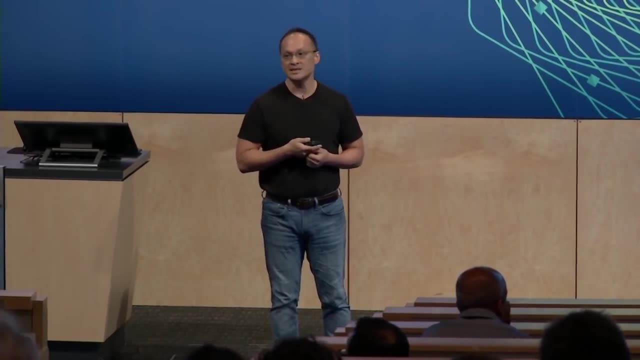 So this is not saying that this is unique, But I think it is indicative of this general understanding and the evolution of capabilities and mindset that is, in fact, changing the way we look at the world. So let's start with Bing, right? 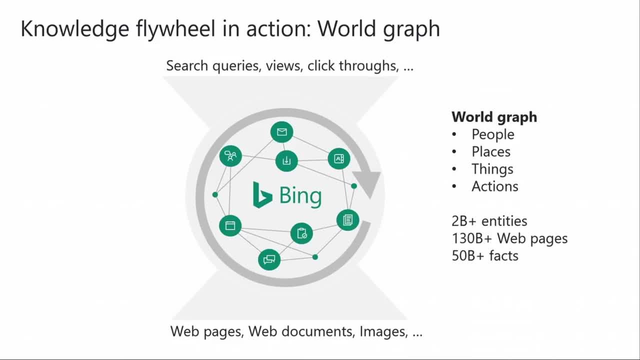 Bing is a search engine, web search engine. You've got lots of documents, You've got queries coming in. In fact, there's a beautiful, beautiful interaction model of ranking, feedback through clicks, from which you start building out a richer and richer index of the web, of the documents and the concepts within. 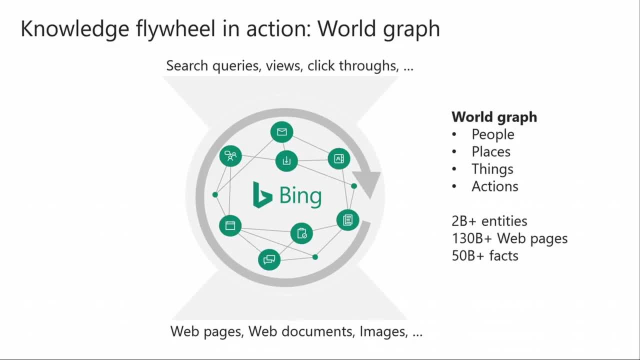 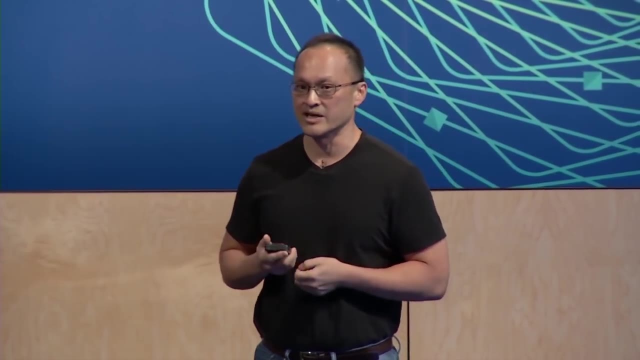 So as part of that, as we did several years back, probably 10 years back, we started working on Knowledge Graph because, hey, why stop at just going to links, Why not bring that information and start creating it? Why not create that information or that action that can be directly engaged, without one hop? 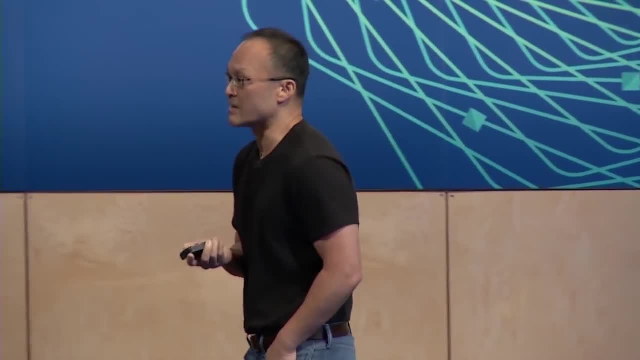 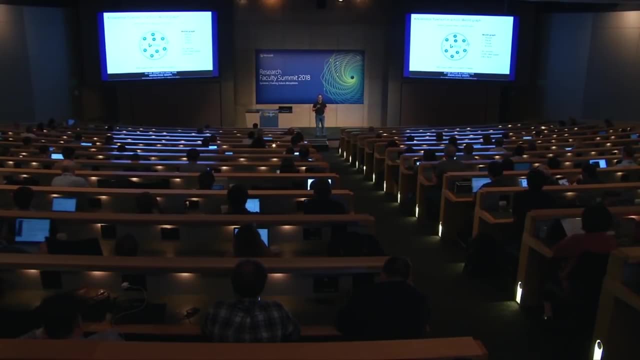 away. So we started building this Knowledge Graph. It turns out to be a pretty big graph: 2 billion plus entities continues to evolve across different domains. It's open domain, many, many web pages, lots of techniques on it. But the thing that is interesting is, around a couple of years ago, we started shifting. 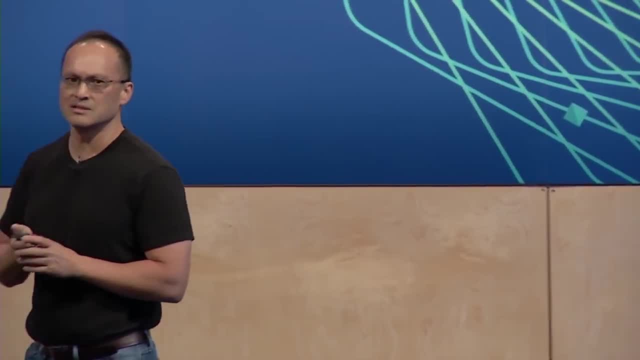 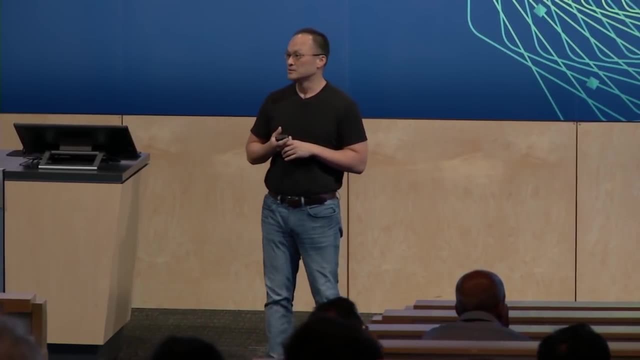 it from. oh, that's just a Bing graph. That's just a Bing graph, It's only useful for Bing, And we realized that. what underlies it? It underlies it is, in fact, a model of the digital world. 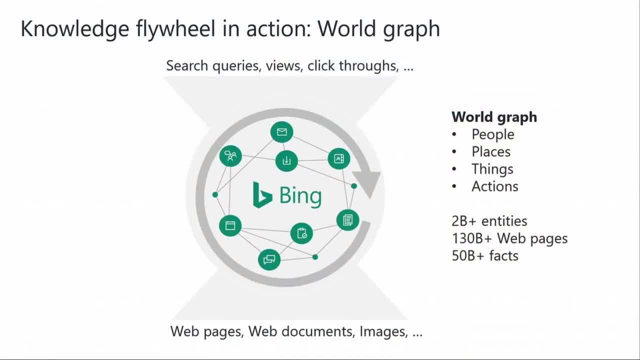 These are the people, places and things that happen on the web. These are digital artifacts on celebrities, people on locations, stores, And when you look at it from that standpoint, we're starting to now create, understand both the facets, the relationships of things in the world, the public world. 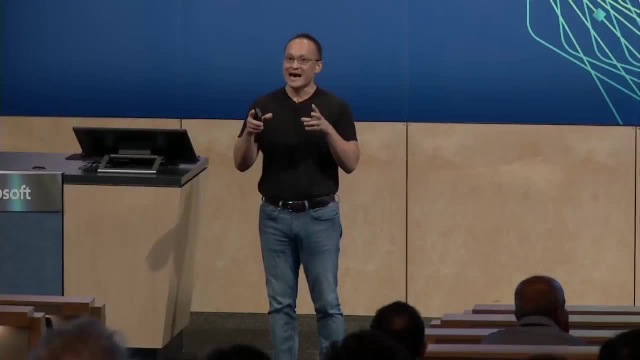 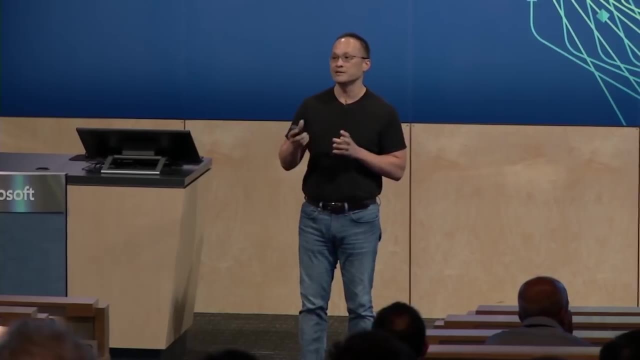 And we can start joining with structured data And, as a result, that piece of asset, That piece of asset created a life of its own. It's now valuable, not just in Bing, but it's valuable whenever you need a model of the. 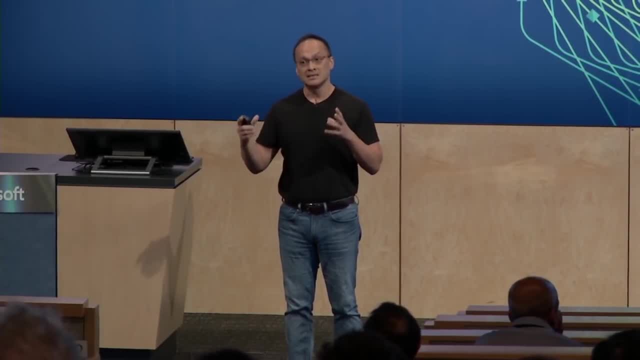 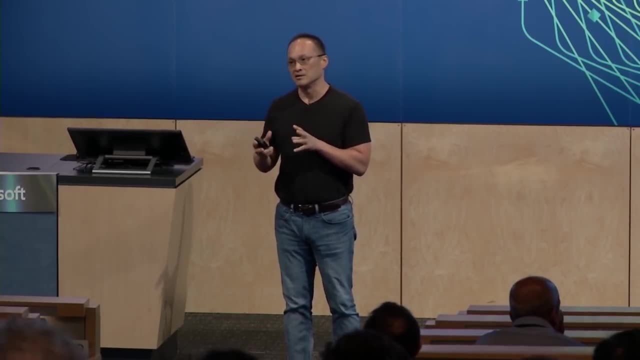 world which could be in Office, which could be in Cloud, And that's something we're seeing, this general pattern that you start out with an application feedback but you start creating valuable assets and knowledge models that have life beyond that scenario, And let's go into the next one. 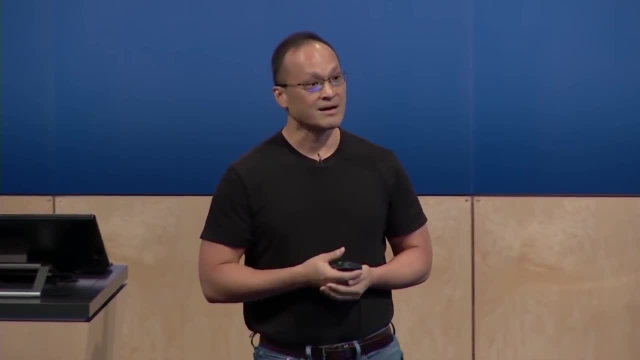 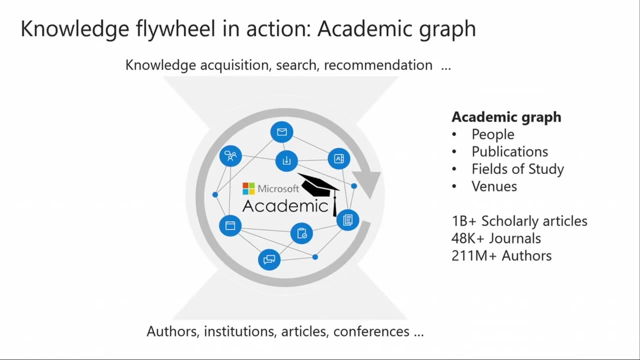 So a little bit later my colleague Kwong San will come and talk a little bit about the Microsoft Academic Graph And this one. think of it as this is a graph that models research and technology innovations and really that process of who communicates and what publish what collaboration from. 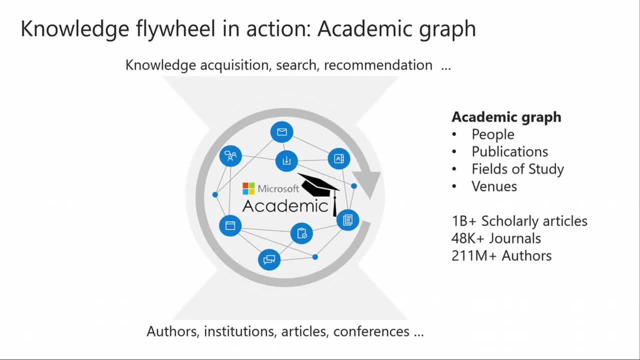 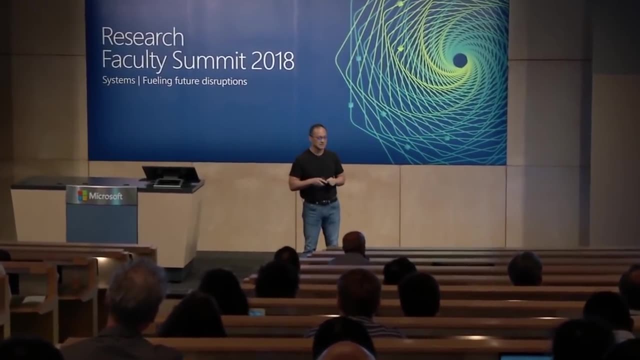 what institution and where does the flow of new ideas start to now come up from the minds of people into broader adoption and inspiring whole fields and domains? And that's another example where you can now use that aggregated signal from many, many different places. 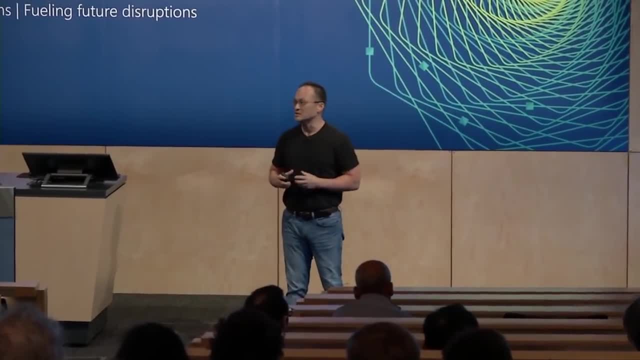 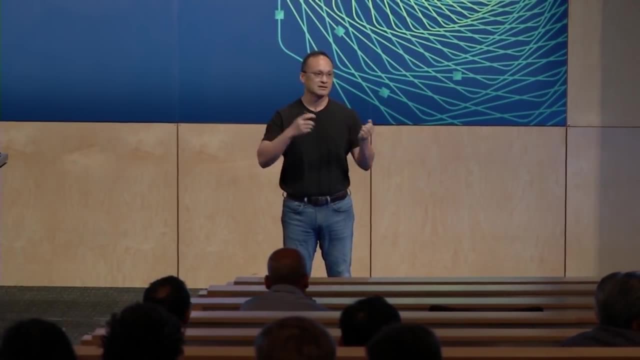 So if you look at the field of communications, the fields of studies and start to create that ontology that gives you predictive power on the impact of new articles or new fields, Is that a hot field? Is that going to gain traction? These are really that model that now takes a life of its own, that you can now extend. 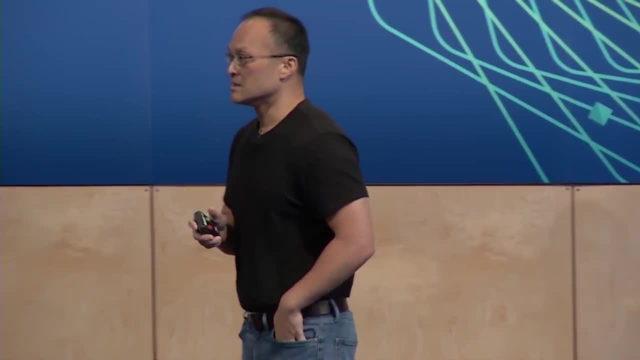 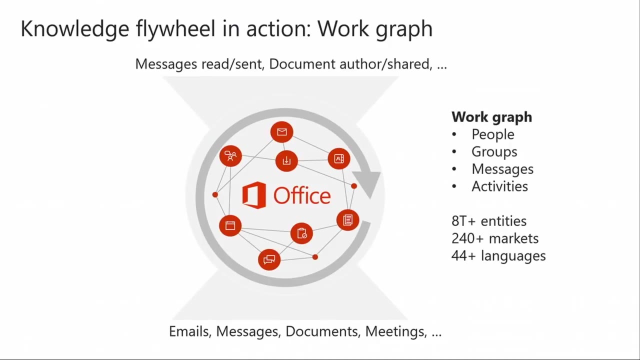 to other areas And in fact, it's not just the public domain, It's also in enterprises. So in the case of Office, you would say, hey, Office is just a bunch of Word, Outlook, email, SharePoint And in fact, Outlook is in fact, at this core of how people in a company interact and communicate. 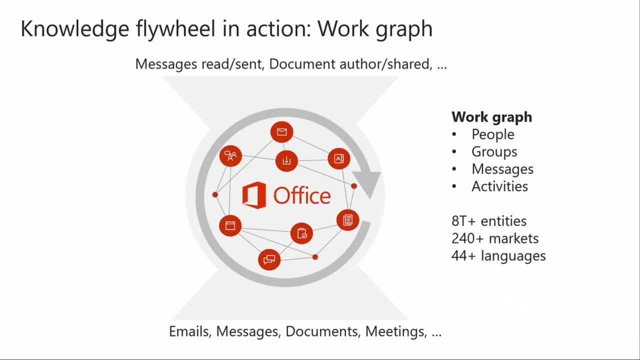 and collaborate, So that flow of signal allows us to start creating a model of digital work, how collaboration happens, on what topic? how does people in the organization impact that? how do we now understand the activities that people do? how do we now understand, in fact, the topics? 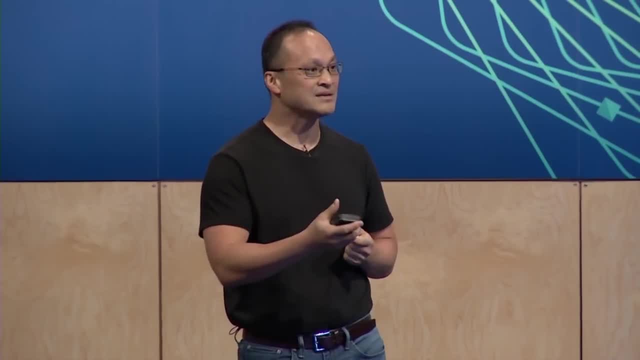 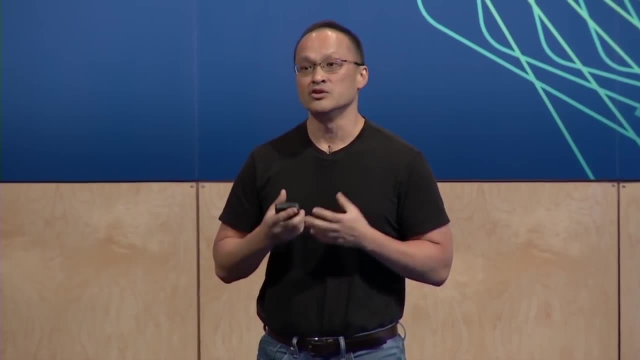 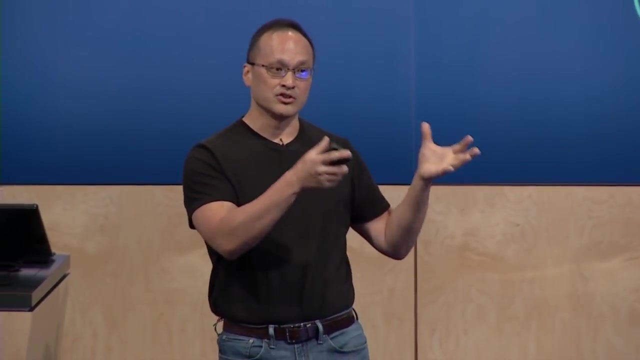 and the customers and the interactions to predict effectiveness of engagements with companies. collaboration across the board. Thank you, Oh, thank you, Mase, And I think it's really like one of those things that I think is really interesting is because it's not just Mase. this is a platform that you can access for anything. 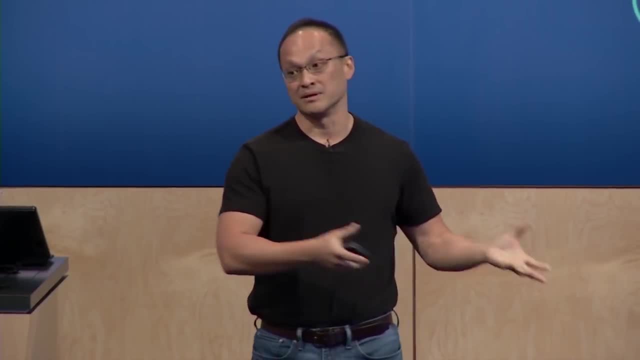 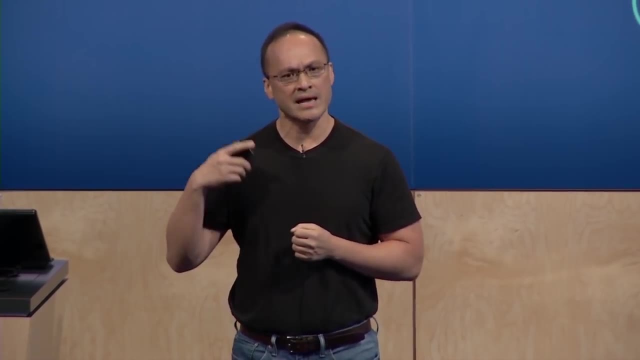 in this community for anything in the field, And it's not just the Internet right. This is the place where you can go to access the platform, And it's not just a few people, In fact. I mean, it's something that's going to be part of the system more and more. 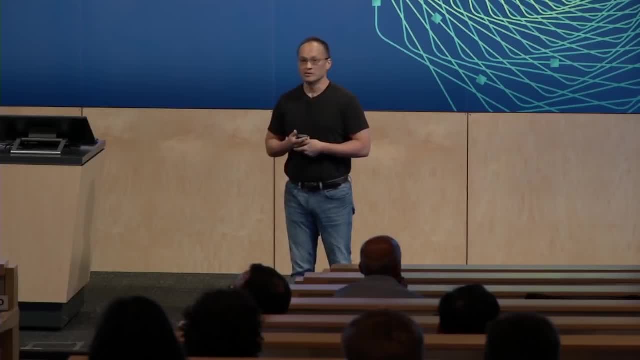 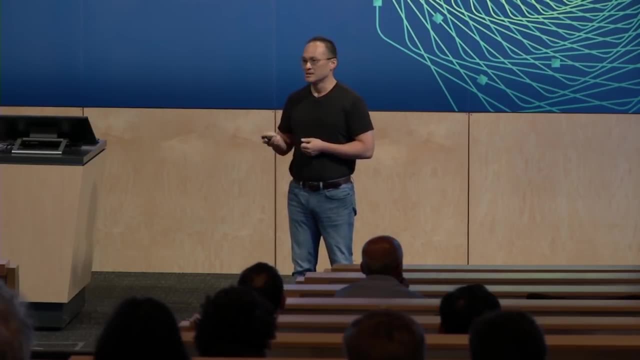 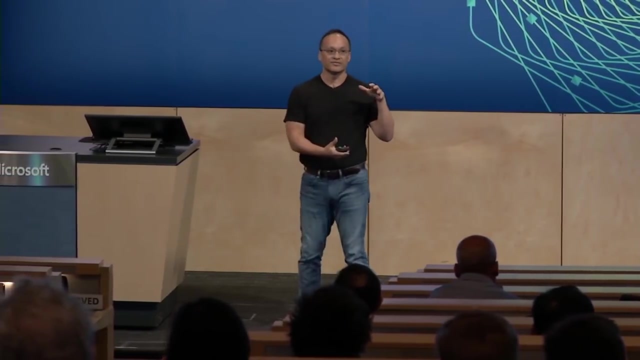 And so they have the opportunity to use that in their own way. digital work and can that create more delightful experiences, but also can that now be bolstered to help companies transform in the way that they interact with their employees and customers. These are just examples where knowledge starts out from. 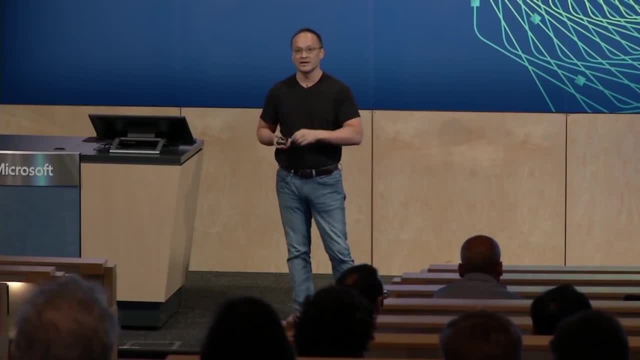 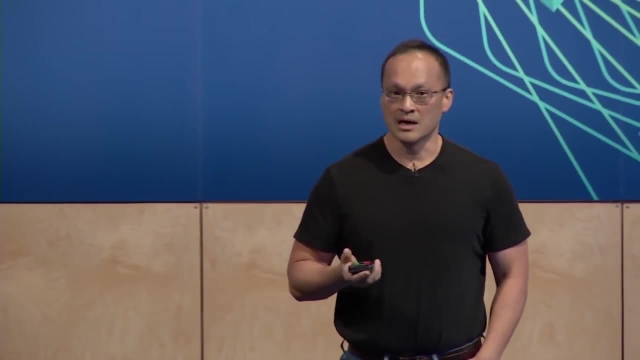 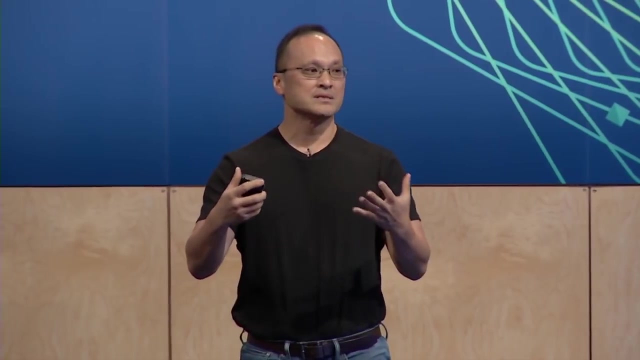 hey, let's make an application smarter- to starting to create data assets that can now inspire and connect to new scenarios. Now, once you have knowledge doesn't mean that it's readily accessible by people. Knowledge is semantically organized and understandable, but human's ability to interact and engage and 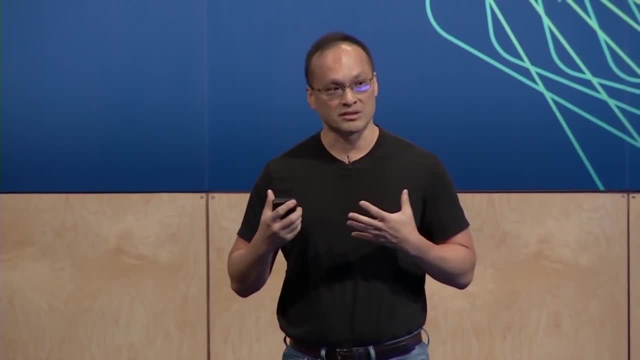 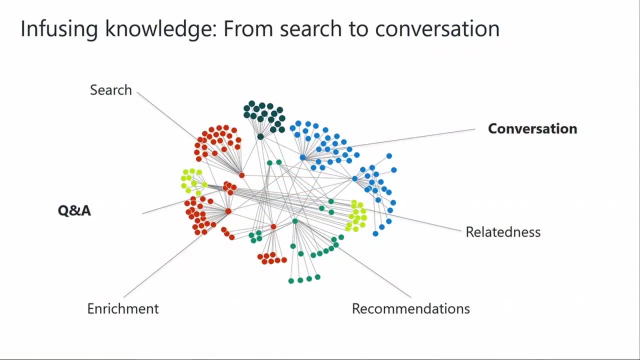 to conflate is in fact unstructured. Let's take for example search and Q&A. You can ask in any natural language anything, but you have to somehow map it to what's known and modeled in the knowledge. Well, that requires technology. 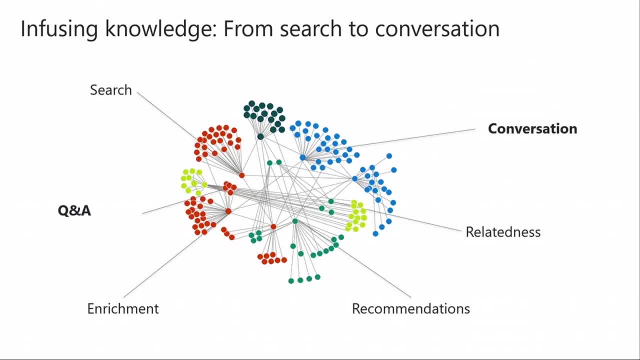 That requires understanding both how to model language but also the information and knowledge within. You can also look at enrichment recommendations, the relatedness of concepts, so that you can start to now connect the dots In the worldview that we have at Microsoft that Satya talked about. 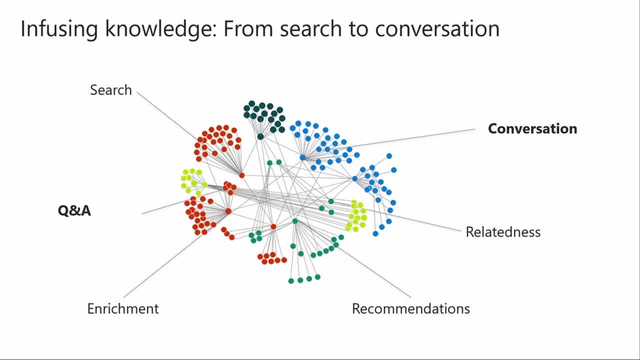 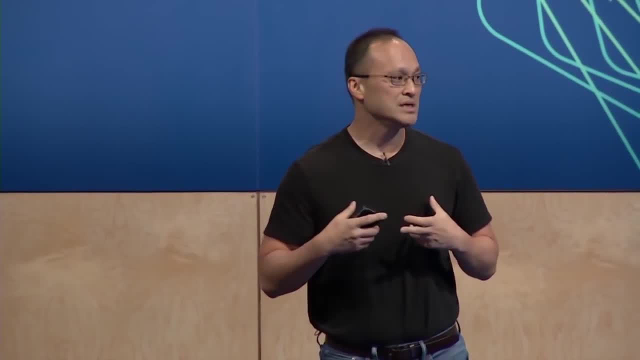 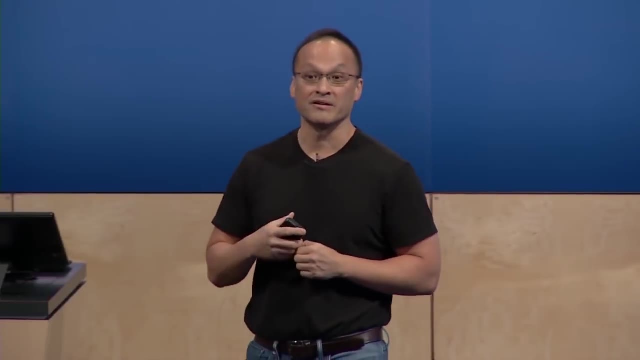 which is this intelligent cloud, intelligent edge. we talked about this ability to connect the dots. It's not just disparate interactions with different devices, it's a multi-device, multi-sensory coordinated world. That coordination, that glue, is in fact that connective fabric of people. 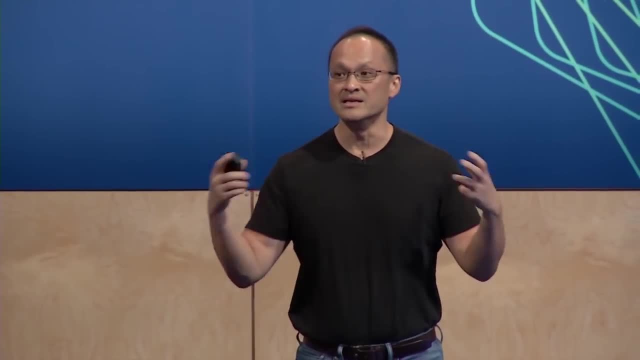 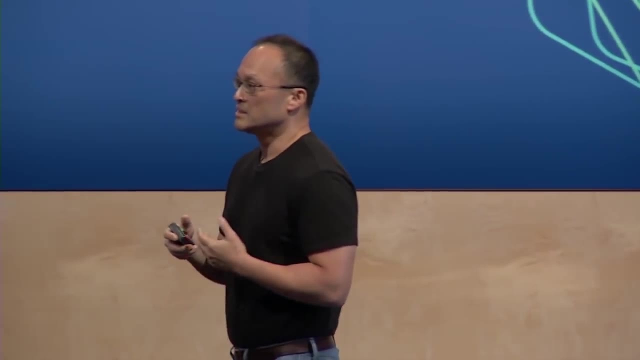 of things, of the environments, of the context, that what is the glue that starts to tie the different pieces together into something coherent? I want to now give some examples of the power of these experiences. when you have knowledge, This is, in fact, the thing that gets us excited. 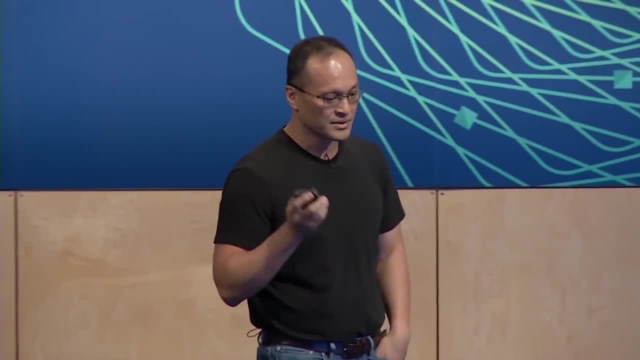 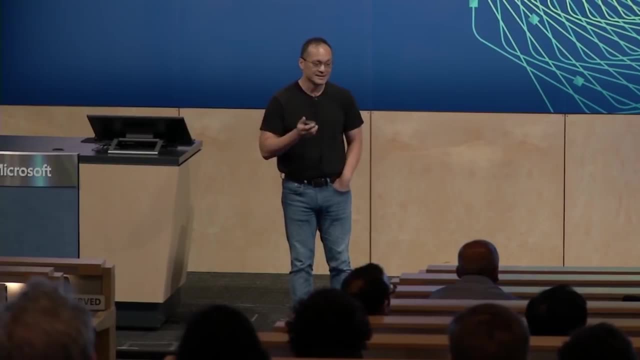 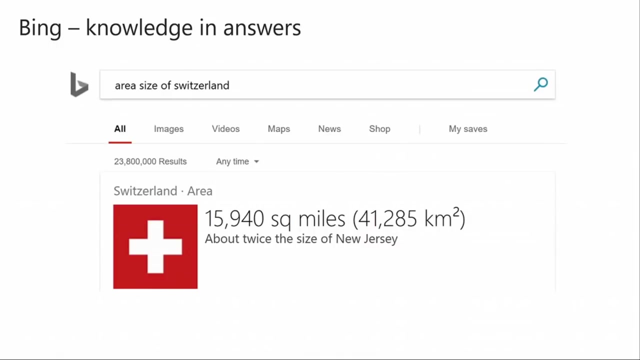 but again, we're at the early stages of it. Let's start with nice animation. Let's go with the Bing, Starting with Bing. clearly, we have the ability to have reasonable and interesting questions around the knowledge graph. In this case, what's the size of Ritzelen? 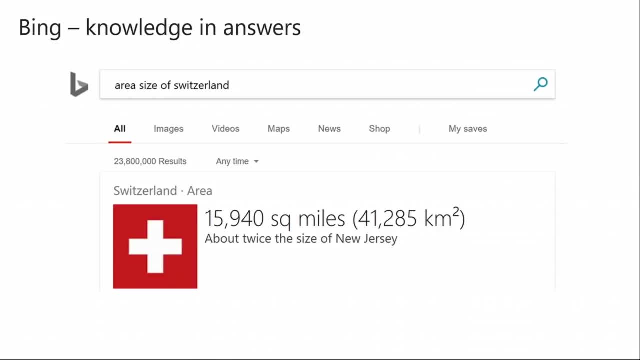 There's the knowledge graph. there are different nodes, there are different facets. based on that, we can now derive the computations to answer that in a much more directed fashion. You can imagine this across a large number of domains. But we've also recognized that that doesn't capture all the information. 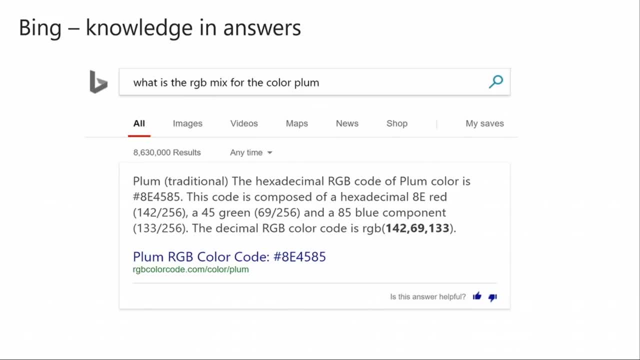 that there's still lots of information in the billions and billions of documents that may not be explicitly represented. So there's lots of advances in machine reading, comprehension, neural modeling, deep Q&A, and these are things that we have in Bing and also in the Maluba, as well as many. 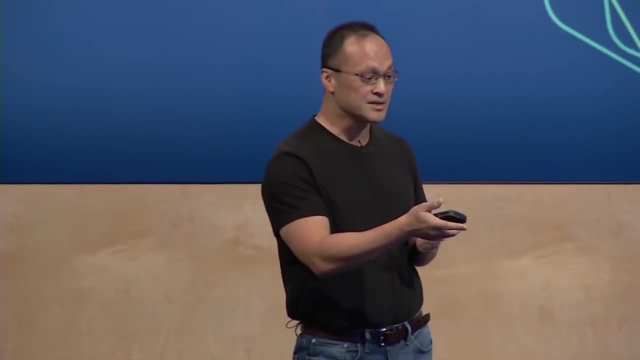 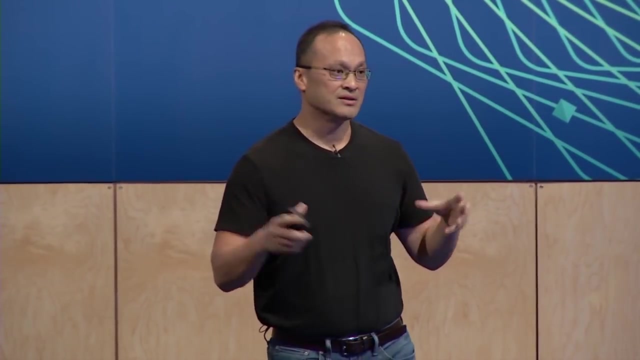 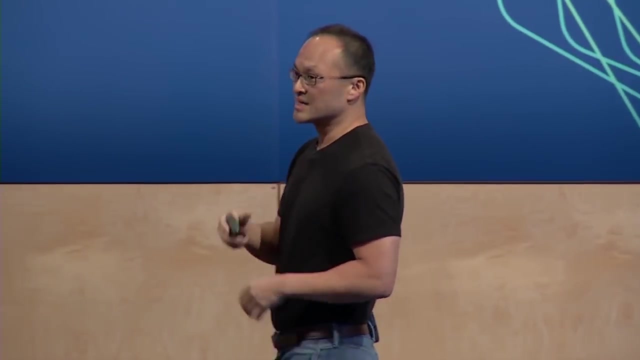 many academia and research systems that are out there. This is the case where now we understand semantically, model the knowledge that's within snippets, different documents, warranties, and be able to now have Q&A around it. In fact, we've taken it one step further and say it's not just one answer. 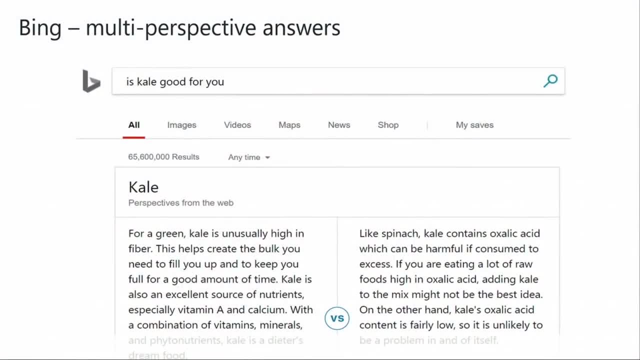 In fact there are different perspectives, because when you start looking at information, it is not the facts only, It is opinions, it's perspectives, and the ability to surface that and to recognize that is also critical. So we have this multi-perspective answers. 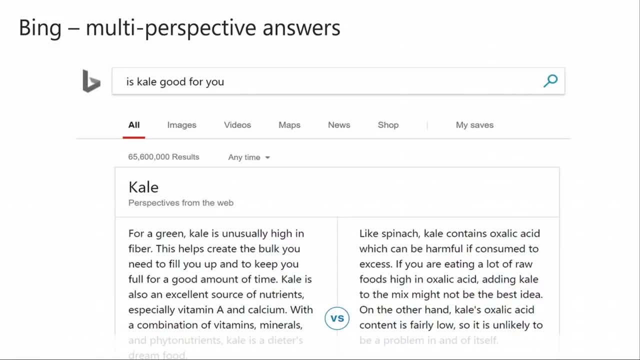 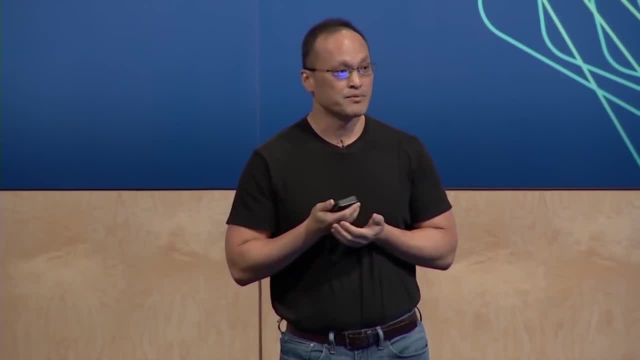 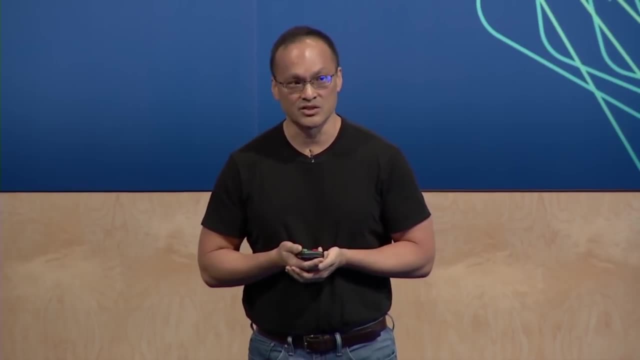 Now these are just examples that now go beyond the ranking of the 10 blue links- to now understanding what is the inherent intent and the need that people may have, and how do we start to surface that knowledge within the web. A lot of that requires us to now invest in technologies that now to 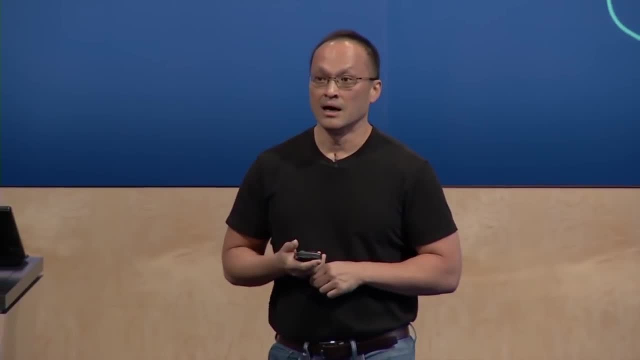 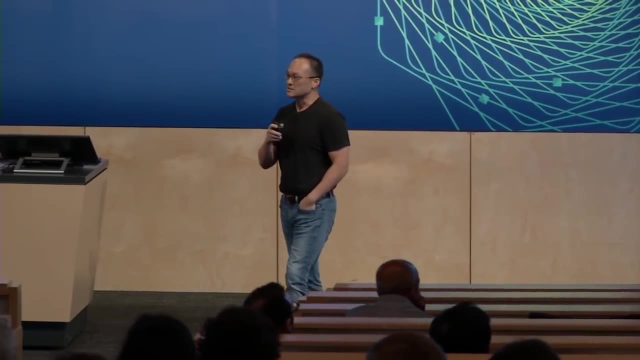 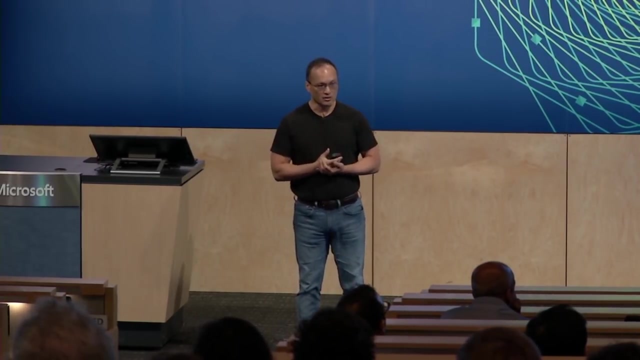 elevate and goes beyond the indexing, the posting list, and to start to look at the organization of information and to be able to reason around it. Now in Office, it turns out we're also starting to now bring that technology and that knowledge infusion into the experiences that you all know like work. 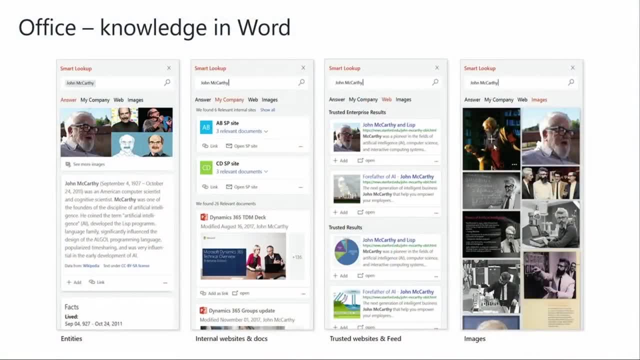 So in this case, imagine you're writing some article, you're writing a paper and you want to know: hey, I got to be inspired, or tell me a little bit of contextual information. So in this case we're- we're systematically bringing what's available on the web from the knowledge graphs. 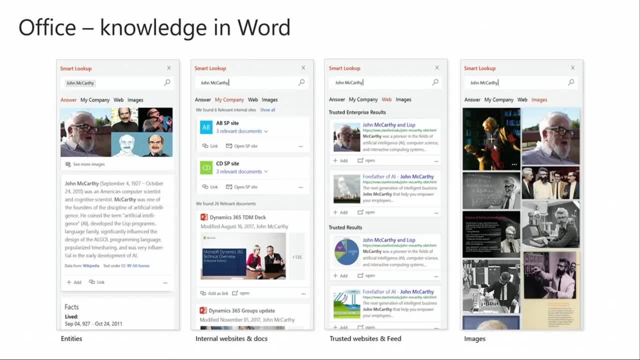 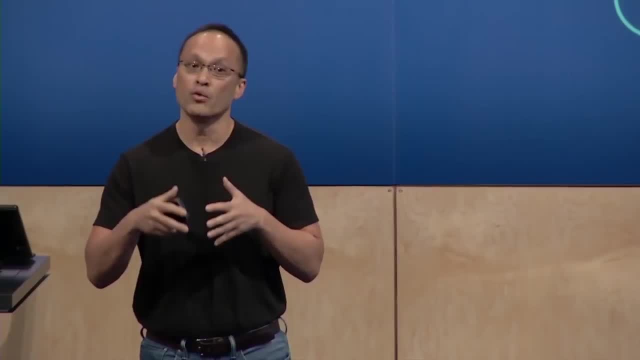 from internal the company to now be contextually relevant to the things that's happening in your workspace, in the thing that you're currently working on. So again, it's a different way of bringing in that connected tissue of context that we think allows you to stay in flow. 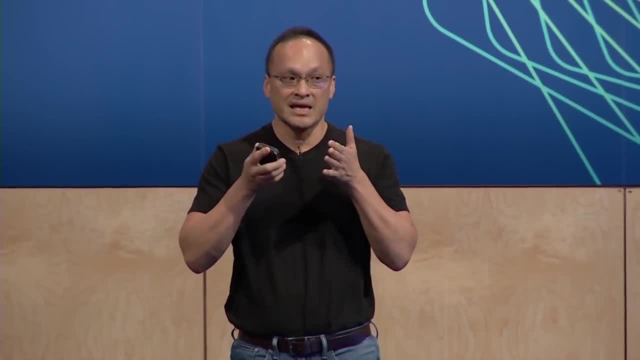 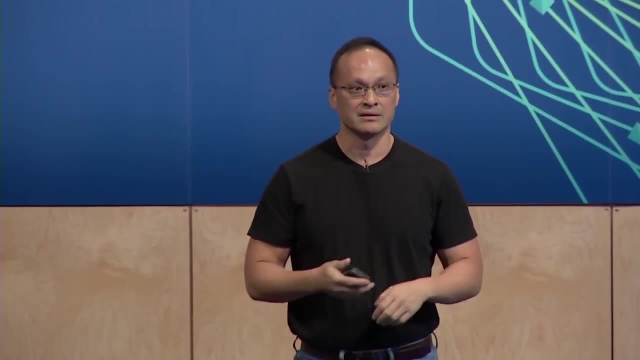 If you look at productivity, one way to define productivity is staying in the flow where you're most productive as long as you can, and bringing that contextual knowledge in a relevant, integrated way to anticipate that next step is, in fact, a hallmark of good knowledge capabilities. 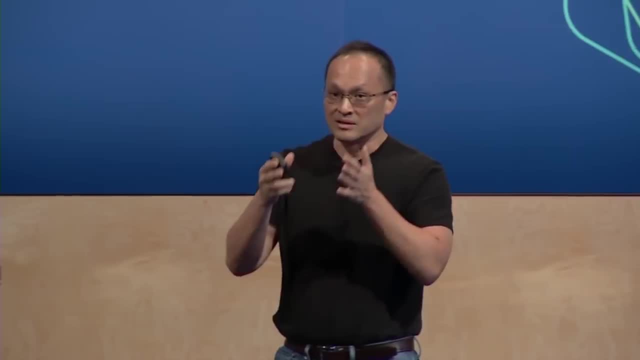 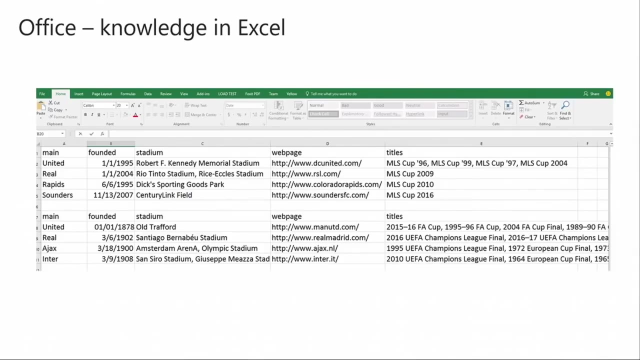 And in fact it doesn't even stop at the word or the flow. Imagine you're in Excel. you got lots of different ways of describing data and values And the fact that there's information that are referenced that may be valuable for you to contextualize. 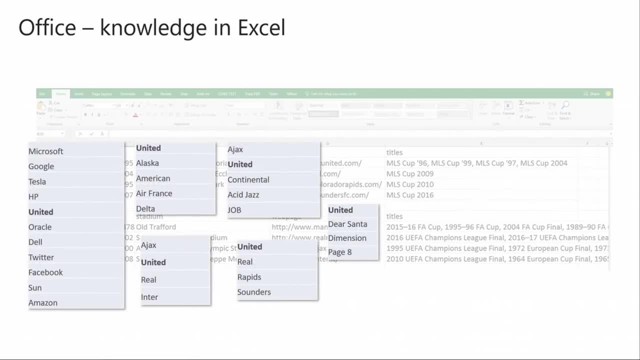 So in this case, for example, you can imagine that, let's say, you have the word united, but it appears in different contexts, And this is just to illustrate the complexity and the richness of the language, but also the ambiguity. So in this case, united in the last context is in fact a bunch of movies, right? 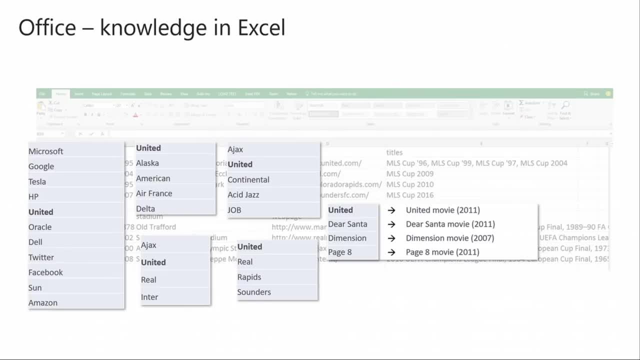 But we wouldn't know that unless we actually understood the other elements to be able to conflate, And likewise in other contexts. it could be an airline, It could be companies, It could be European football clubs. I mean, it could be many, many different ways. 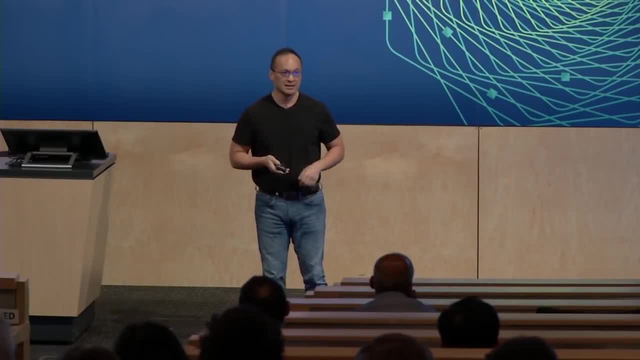 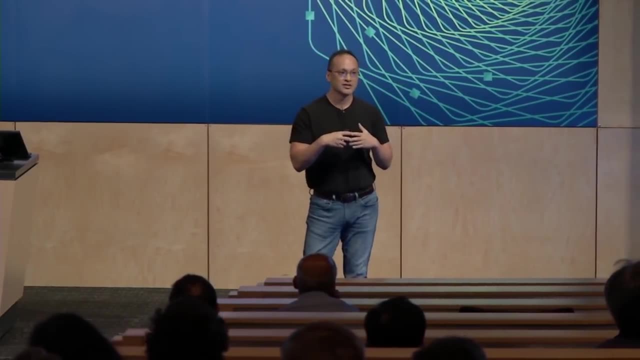 But again, context matters And the ability to model that It is in fact, rich, And so we're only beginning to scratch the surface of bringing information and knowledge in the context of user need, in context or through explicit queries and intent. 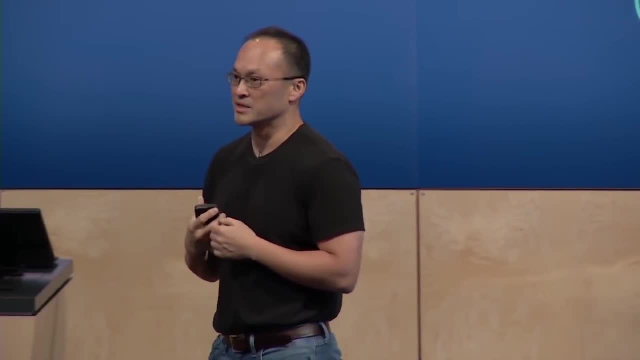 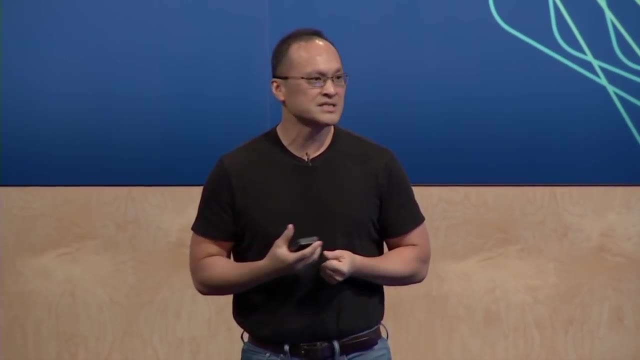 But even beyond this, the one thing that we've discovered as we start working on agents and assistants and bots is that, whereas knowledge may be considered to be valuable, but it's still nice to have, You can still get your work done with 10 blue links. 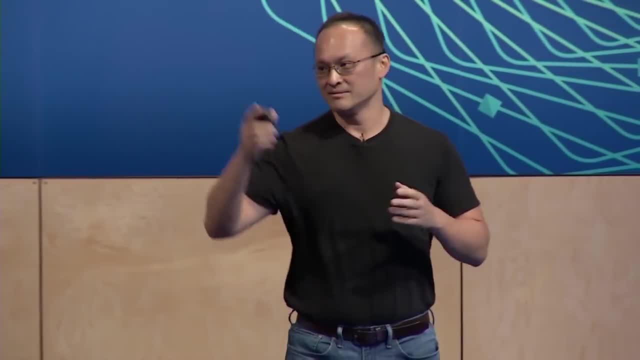 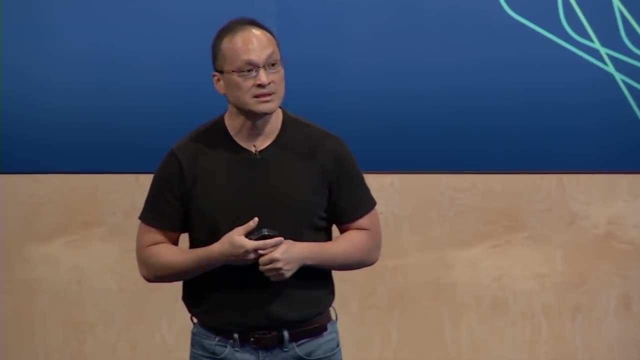 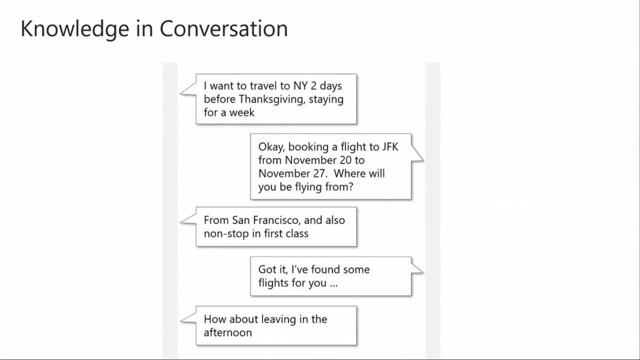 You can still get your Word document done without being inspired by contextual search. But in the case of conversations, especially conversations that go multi-turn, you kind of need knowledge And the reason is the context and the information interactions that you have in one turn needs to be passed and transferred. 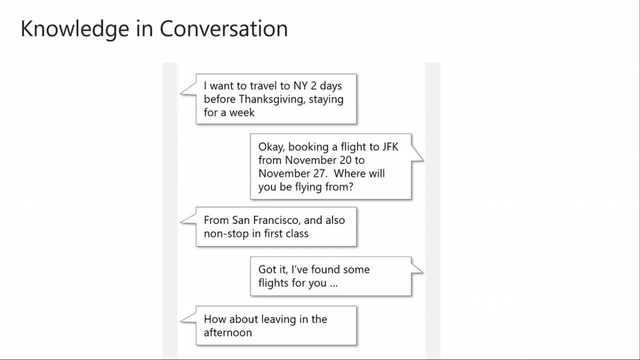 to the next one so that you can start to reason, And that fluidness and that sharing of context across turns, where the turns and the actions taken on each turn may be from different vendors, different applications and different knowledge bases, So it's, in fact, one of the hallmark challenges. 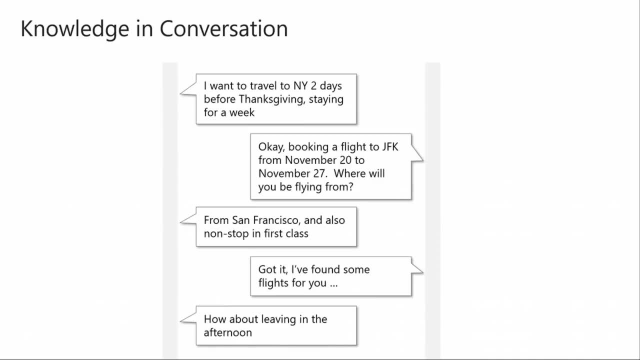 and opportunities in conversation design. So in this case, imagine that you're now going through this flow. In fact, this is inspired by our semantic machines acquisition. We were very excited to get Dan Klein and Percy to be part of our family, But in this case, imagine you say hey. 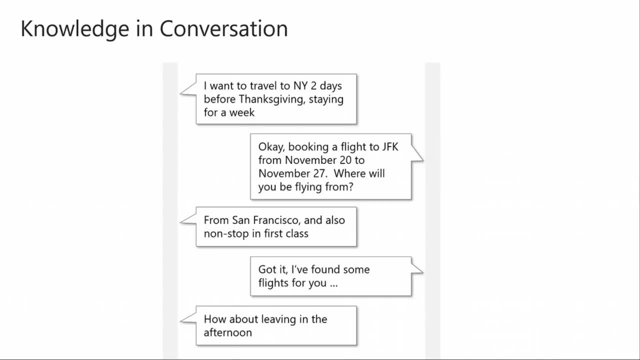 I want to go to New York two days before Thanksgiving. What is two days before Thanksgiving? What does it mean? on New York? Where are the airports? How do I understand it? How do I reflect it? How do I understand the facets for elaboration? 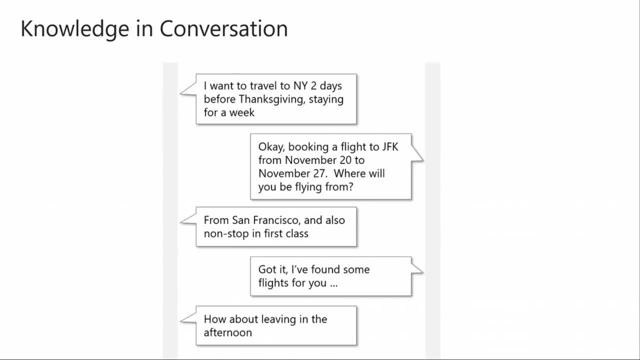 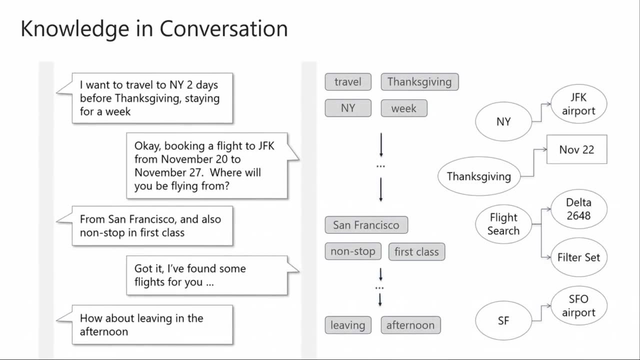 These are all things that you would say. yeah, it actually requires you to orchestrate across many, many back end systems and APIs. Each one has an ontology, in some sense, of the values, of the capabilities, And so, in this case, it's really about this ability. 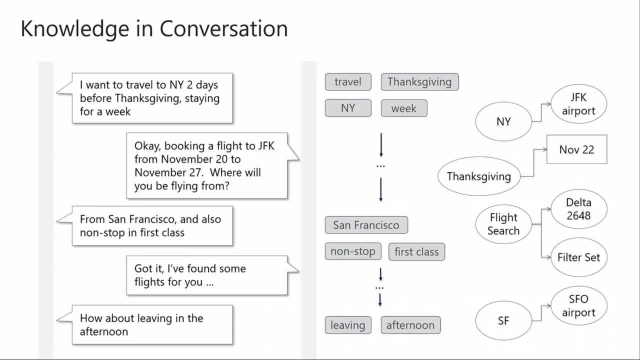 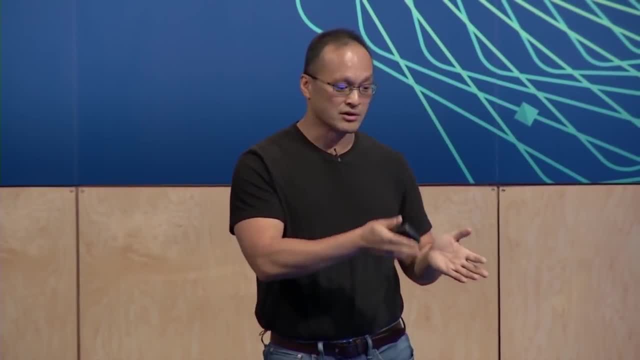 to use knowledge to connect the dots across turns, to be able to reason and contextualize and to guide that discussion. And so, in this case, take travel in New York, be able to now recognize that nearby airports of New York are JFK and this certain location. 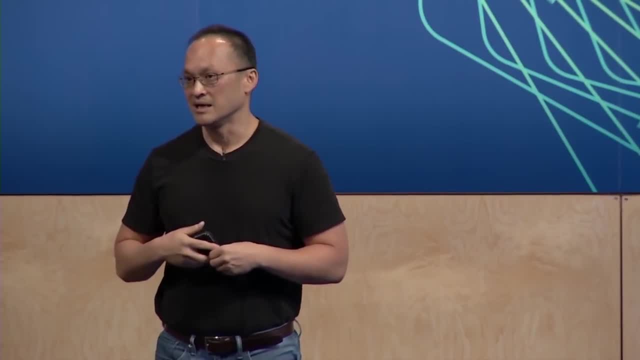 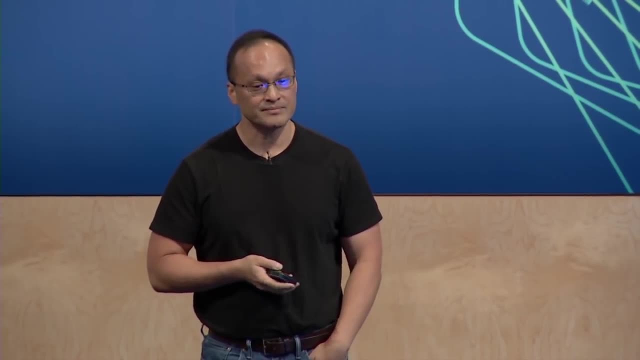 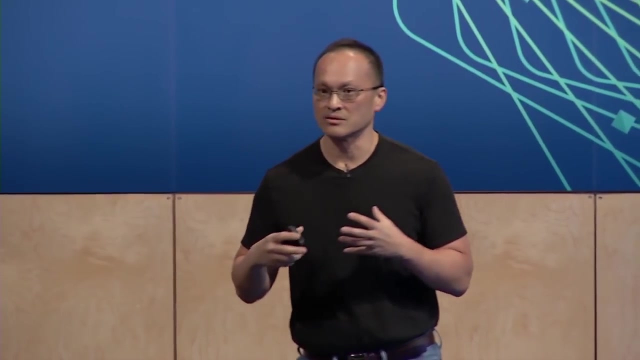 Likewise, you can now imagine each of the APIs and each of the systems having its own data And we need to learn the association and kind of do dynamic conflation across these. Now, with all of the things said, with knowledge, there are many things you can do to start to now. 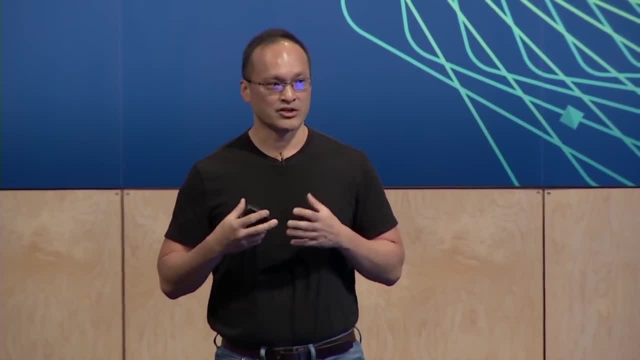 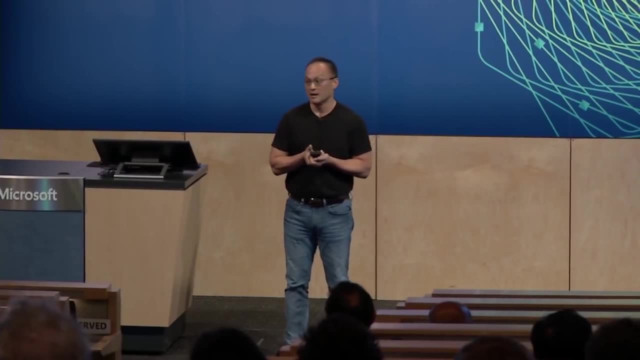 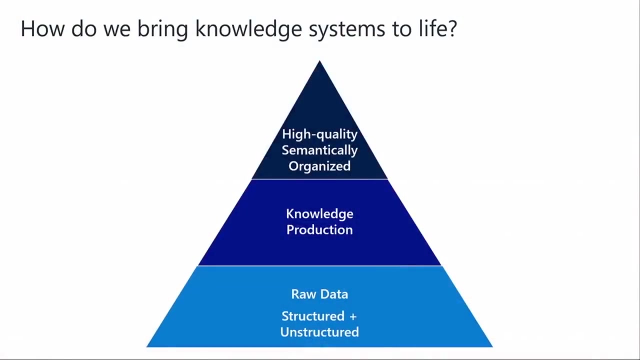 bring that knowledge in the context of interactions and flows, But how do we bring this to life? And this is a rich area of research and product efforts, And so I'm not going to go through the details on this because I think you're all kind of world experts. 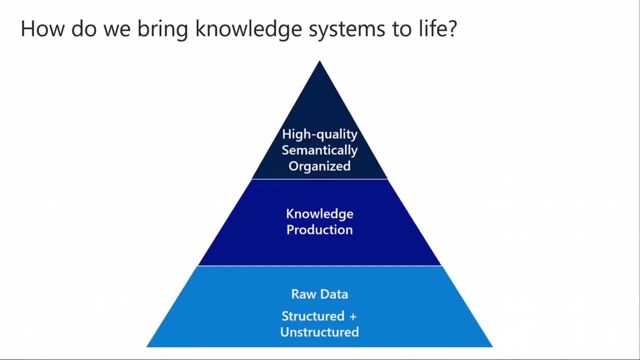 But I do want to share a little bit of how we're looking at the dimensions of what knowledge systems, the quality, what does that mean? and also some of the challenges that we have that we think are really pushing us to the limit. but certainly an area. 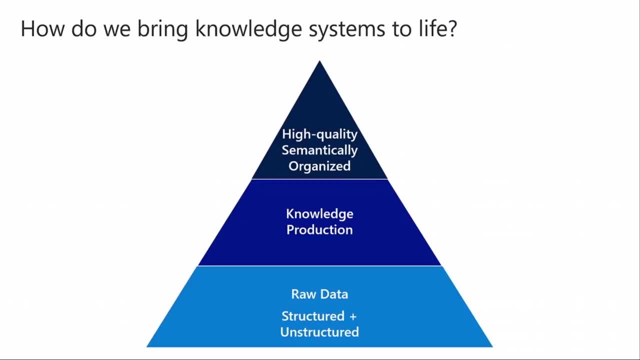 that we like to invite. So, in this case, to bring knowledge systems to life, we start with the fact that, hey, data can be chaotic and can come from structured and unstructured right. Lots of effort across different pieces, but bringing that together in some coherent knowledge. 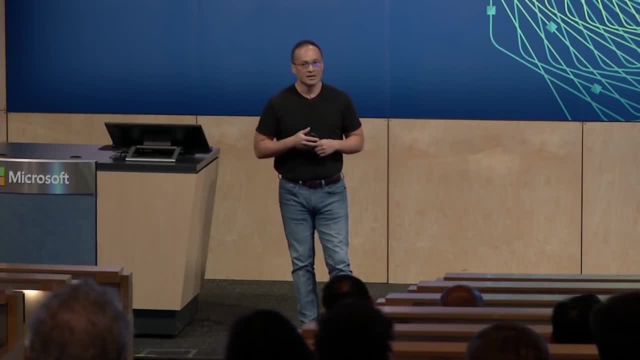 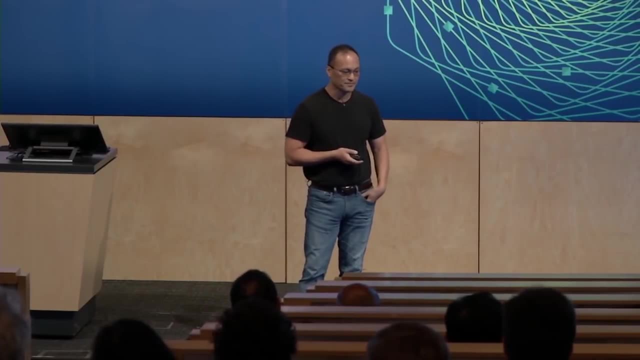 production process to be something where it's fresh, highly structured, semantically understandable. that's a challenge. That's kind of the data chaos to the structured semantics flow And there are different approaches, not that we're going to go through all of them. 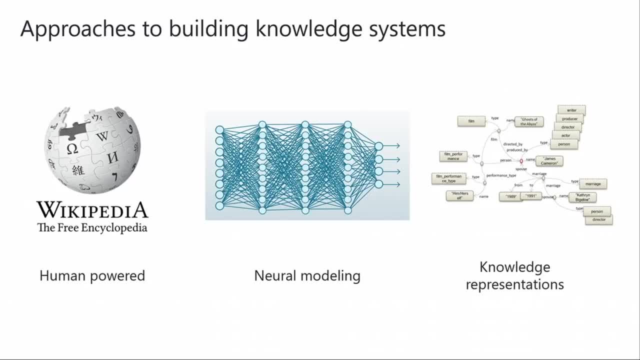 but one approach is better, But in fact, over time a number of these will work in concert. starting with people. You have Wikipedia, DBpedia. There are certain efforts that really do require the domain experts to start capturing that knowledge in some discernible way. 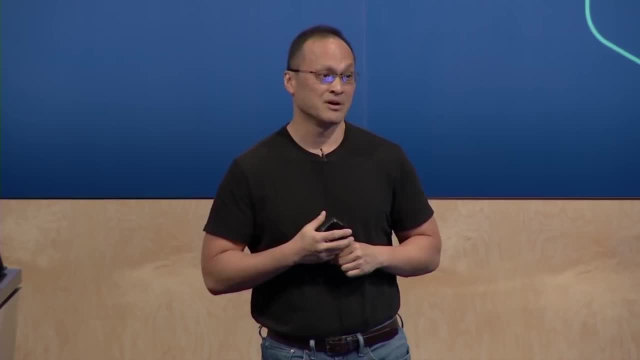 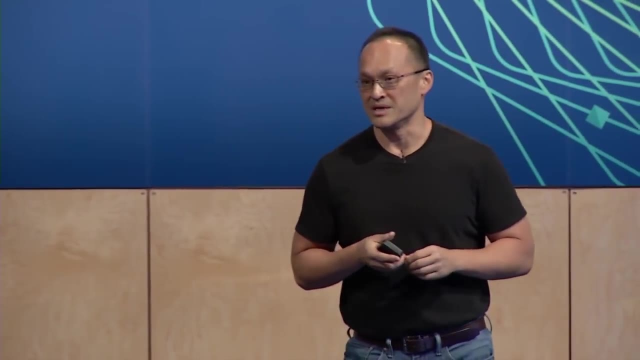 and to be able to now create an incentive that keeps it fresh. Wikipedia is the great example. Almost every search engine kind of looks at Wikipedia and say that's great. Let's use that to seed our understanding, because that's probably the best articulation of what's going on. 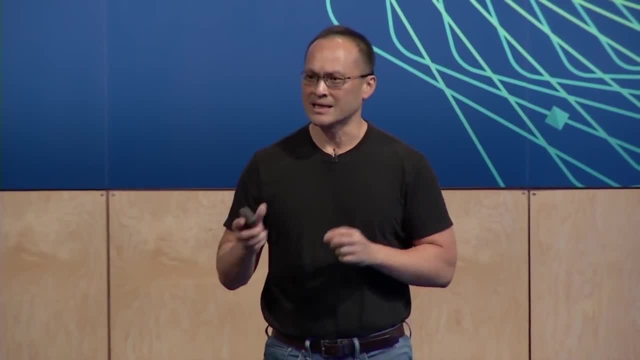 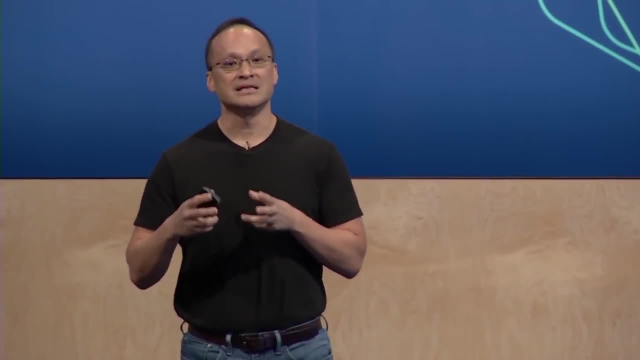 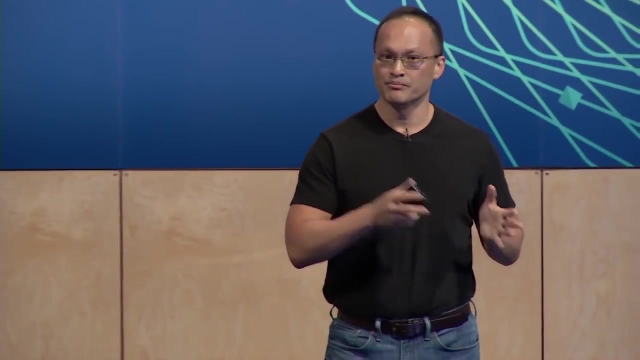 The basic, shareable knowledge that people interact, And that's one of the facets that I think is important for knowledge. It's not just important for systems to understand, It is something that needs to be understandable and explainable to people. But, beyond knowledge, people at some point 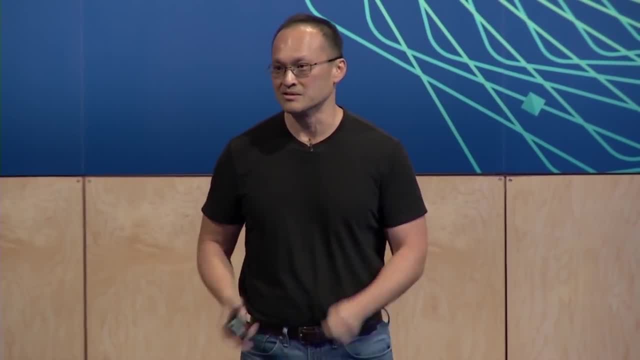 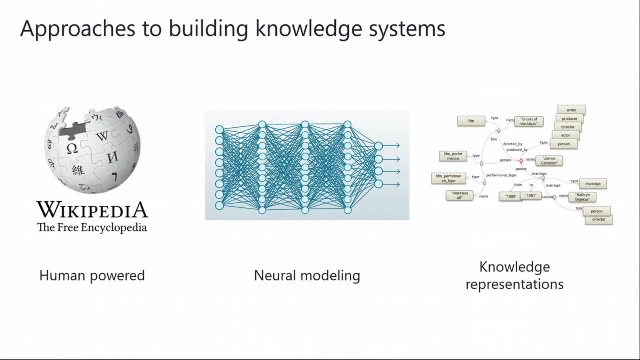 you're going to run out of steam because, at some point, either the willingness or the capacity of people are going to hit a limit, And so this is where systems start to come in. So this theme of systems for AI and AI for systems, 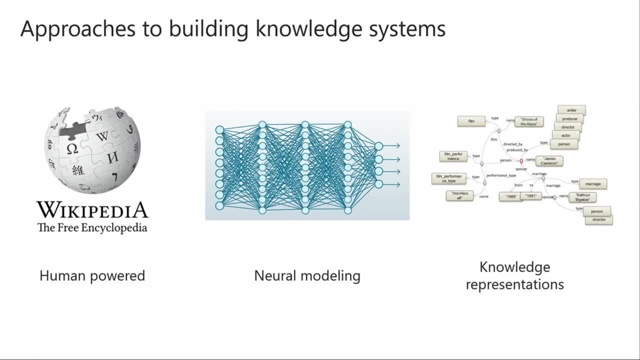 is in fact one of the hallmarks where I think it applies beautifully to knowledge systems. So in this case we can imagine implicit modeling. We talked about deep machine reading comprehension. We're still at the early stages of it, But again this is a case where we're now. 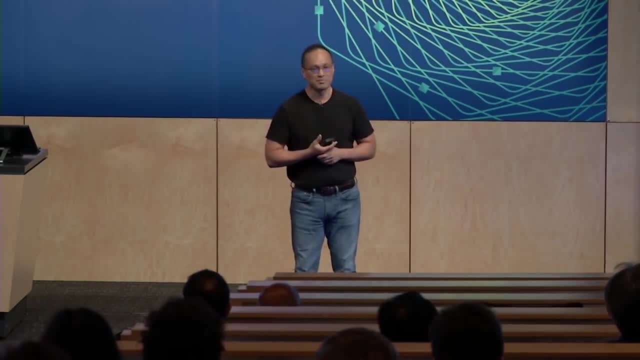 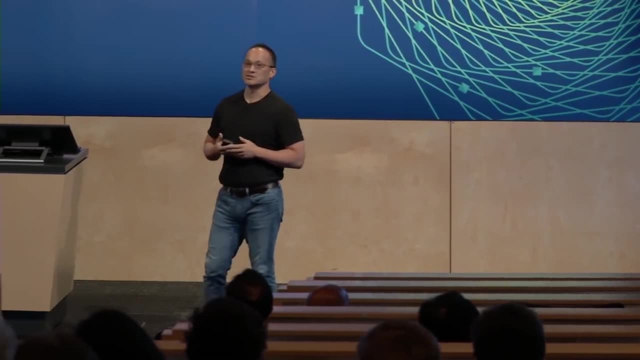 trying to understand the shape of the language, the shape of information and the shape of the retrieval. So lots of efforts on that. But there's also knowledge representations that are explicit. These are the triplets, These are the RDFs, These are the different graph structures. 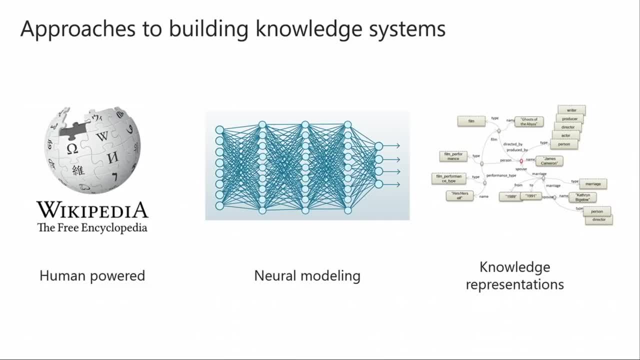 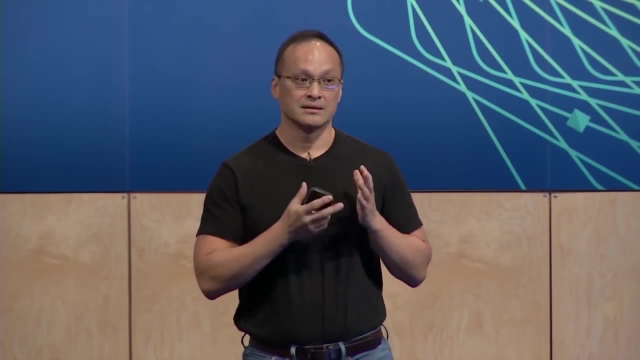 And there, I would say, we have lots of research and lots of production systems: Bing, Google, Facebook, LinkedIn. they are all the systems that are creating these knowledge representations, some of which are proprietary, some of which are public, And, in fact, a lot of the research systems. 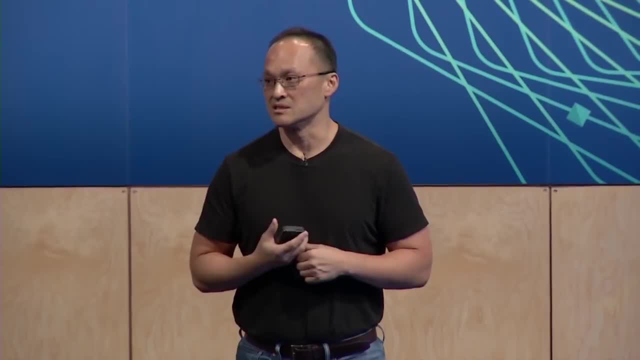 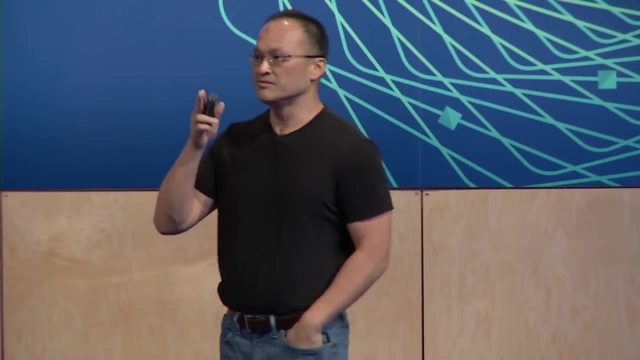 psych from the early days all the way to the research systems that exist today. So this is an active area. Now what I want to do is just talk a little bit about, regardless of the approach, there are different dimensions that we evaluate and assess: knowledge. 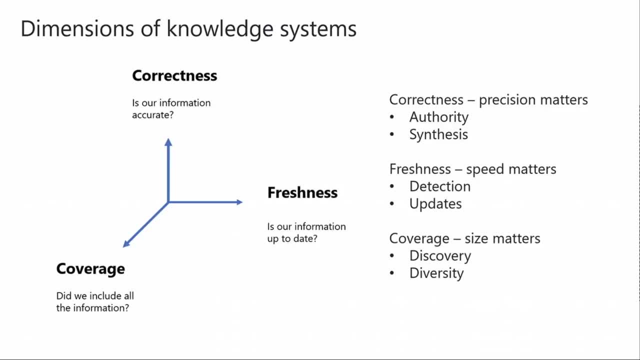 Is a knowledge system correct? What's the degree of correctness? What's the degree of freshness? What's the degree of coverage? There's a standard, But when you start looking at it they kind of work against each other when you hit extreme scale. 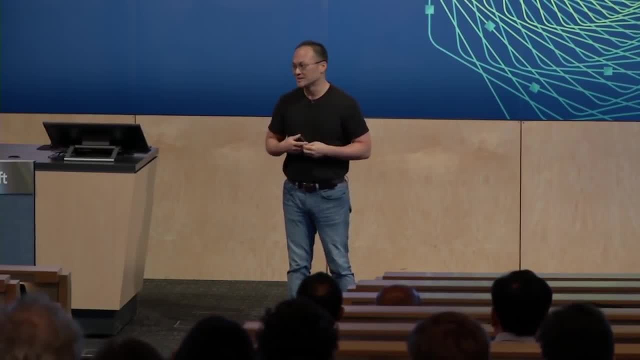 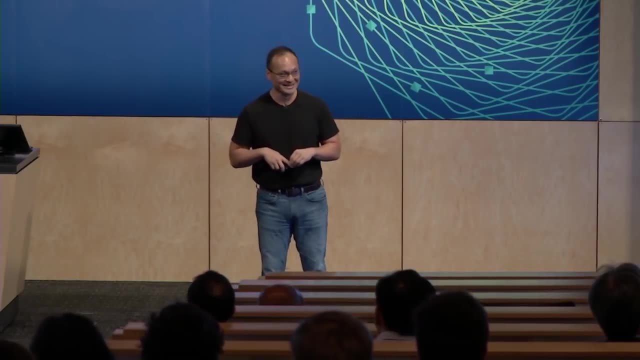 In fact, that's where we end up, which is: it all sounds good For 1 million documents, it sounds good For 10 million. it works really hard If you have hundreds of billions, And that's kind of the chaotic web. 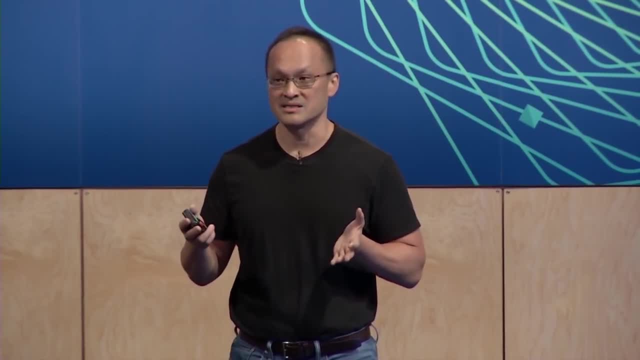 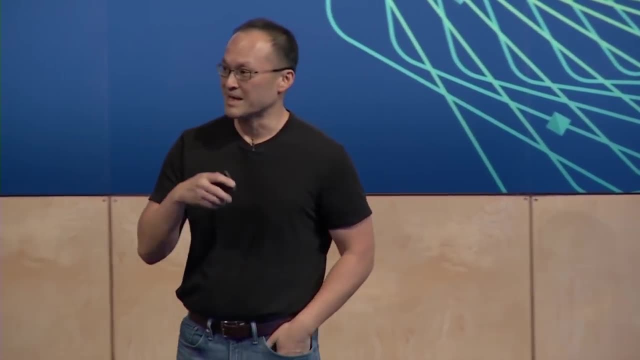 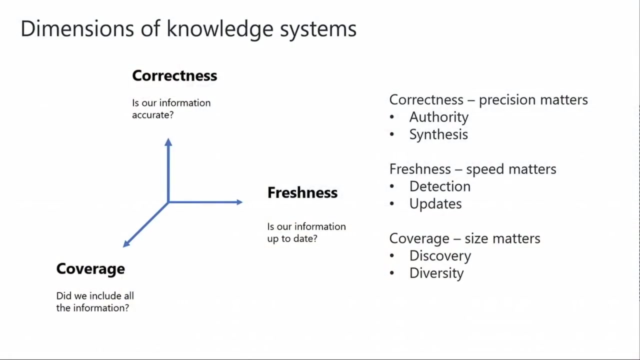 And it's not just a chaotic web, It's chaotic enterprise systems and kind of real life situations. So with that, let me just give some examples. In the case of correctness, precision really does matter, Because once you create that knowledge, you have to stand by the quality. 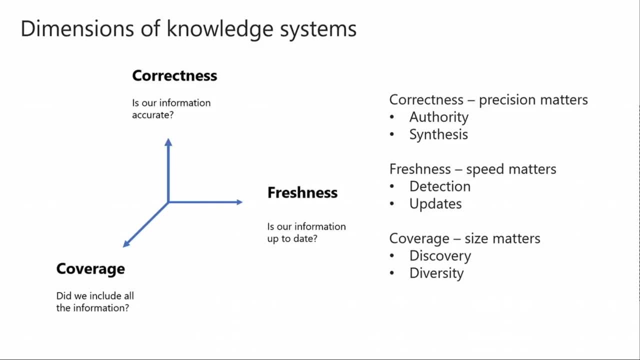 If something is wrong, you can't just point to the source and say, well, I don't know, I think I extracted it. This is fake news, It's fake knowledge. You got to look at authority. You got to look at authority. 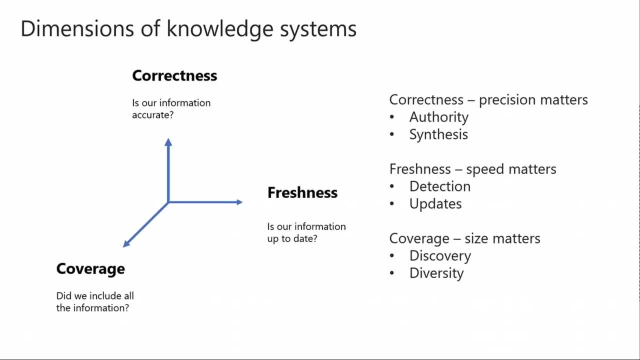 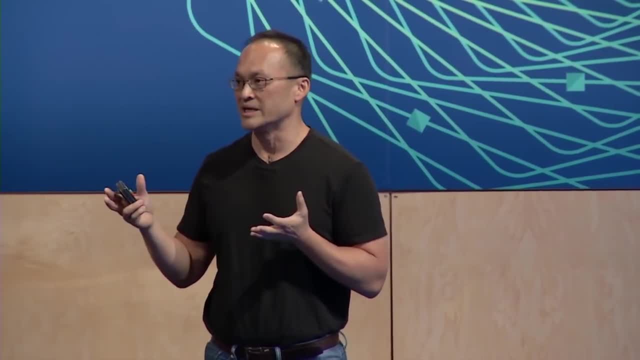 You got to look at the synthesis. How do I look at voting if I don't have an authority? How do I judge? How do I get user feedback? That's a challenge, especially when you have unorchestrated multi-party sources of information. 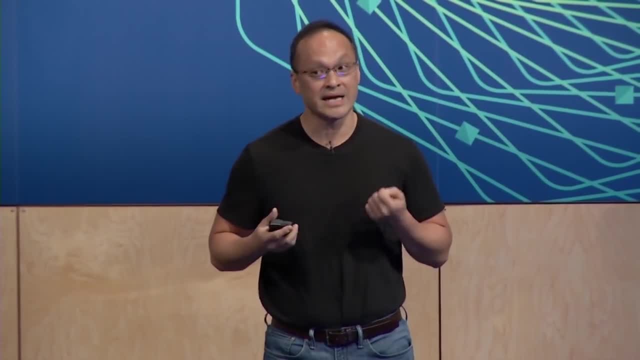 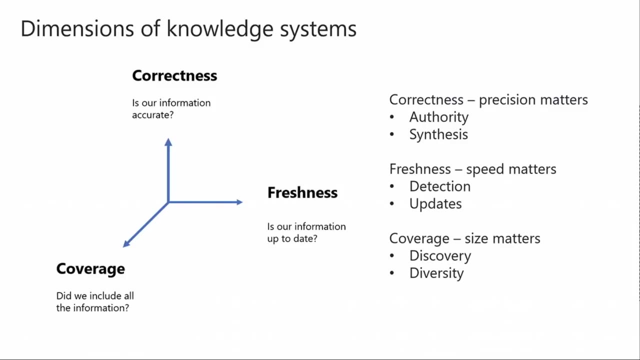 Freshness, speed matters. Things are constantly changing. In many cases, we don't even know what changed, Not to even mention the ability to propagate that update through the system in a way where we understand that some of the updates may in fact be incorrect. 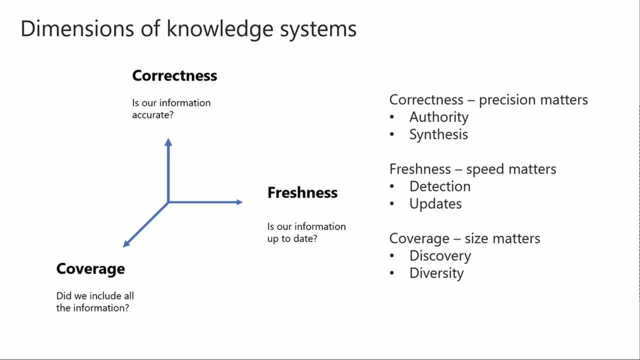 So you can actually start propagating lots of challenges. with one mistake You can ripple and destroy pretty much everything, And that's the lesson we have. And then coverage- right Size really does matter. At some point they'll say, great, this all sounds good. 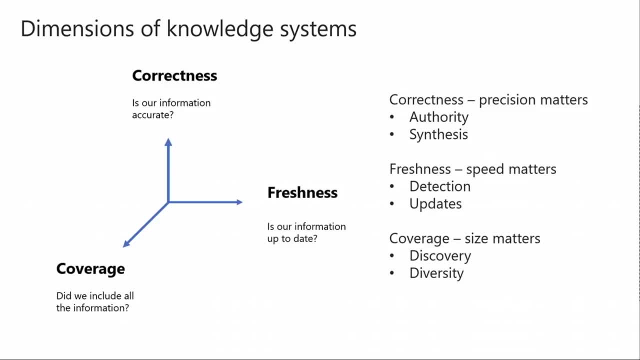 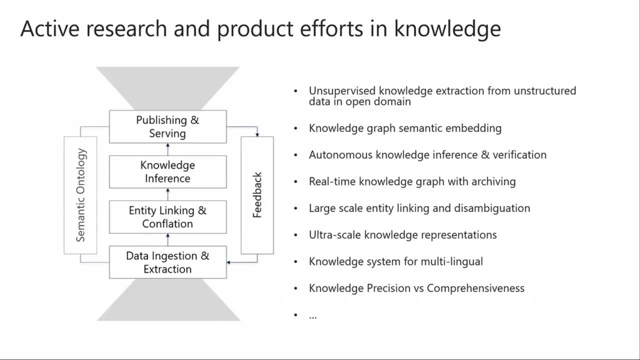 But is it complete? Does it capture that domain? So all of these work in different forces, And there are lots of systems and lots of efforts that are, in fact, at the frontier of this. I want to list out some of these. 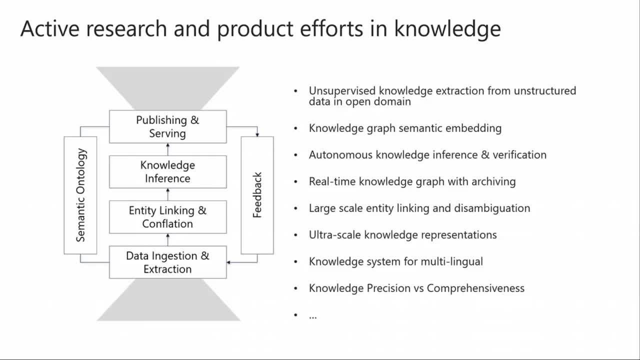 I want to list out a couple of them. One of them is: I think one of the most important is to both acknowledge that lots of problems still remain unsolved, but also the importance of these problems for us to get ahead in this world where I think knowledge. 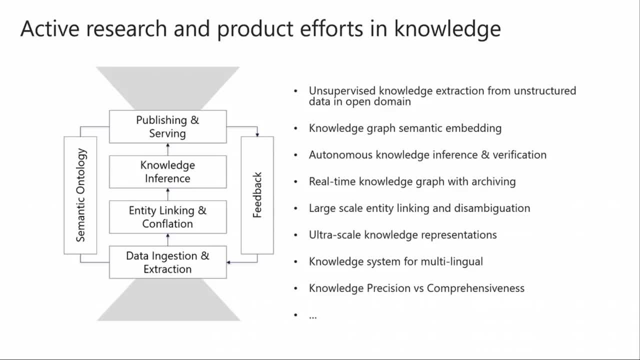 is increasingly important. Unsupervised, unsupervised, autonomous- These are all keywords. Basically, we say we can't put humans and depend on humans to do the final verification in all the cases. How do I unstructure? When I look at a web page, it's not just the head sites. 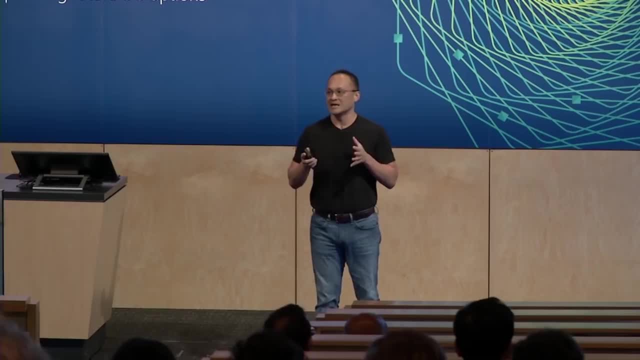 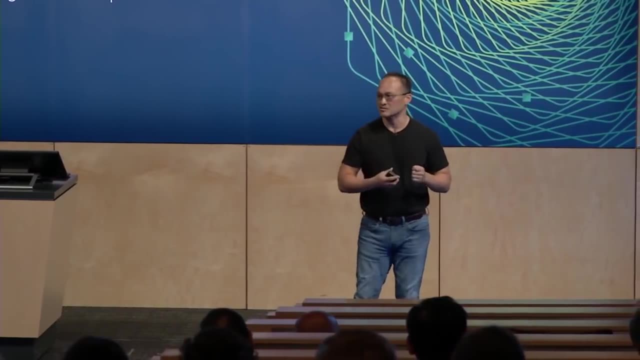 and production site understanding. Can I understand the unstructured nature of the information? Can I understand and cluster? Can I extract facts? Can I test that hypothesis through verification and validation? That's a whole body of work that pushes from the head to 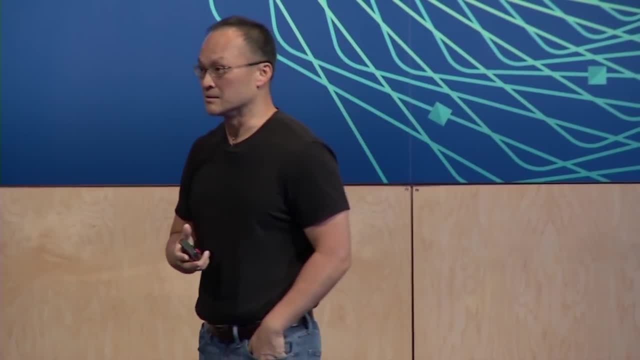 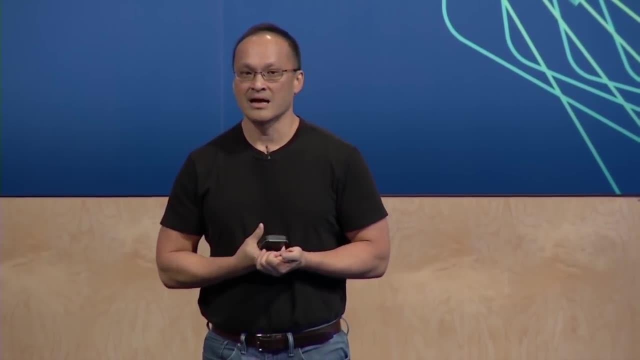 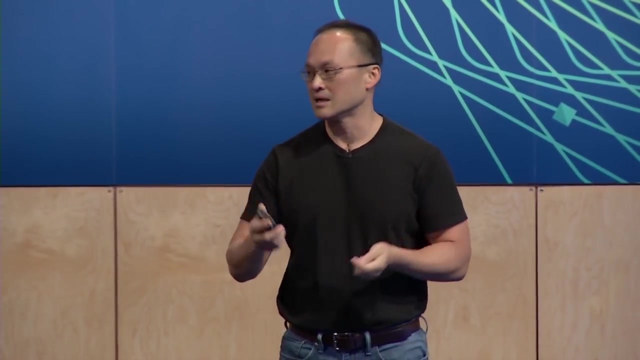 in fact, that torso tail Knowledge and semantic embedding. you've got lots of today, explicit knowledge that's present today through years and decades of human aggregation or capabilities, aggregation Right, OK, and yet we're building neural networks, and how do we seed it? how do we anchor that knowledge? 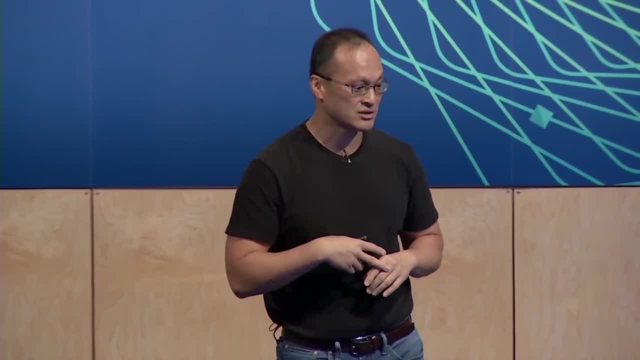 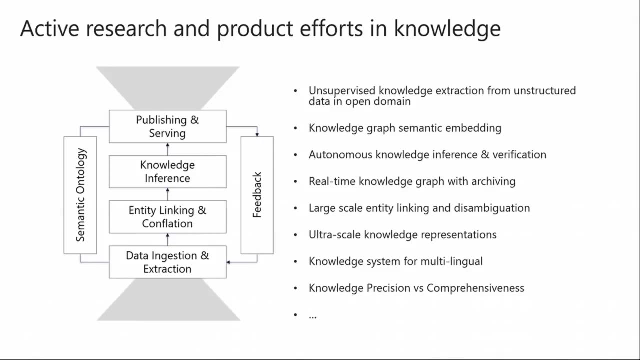 so that you build upon it as opposed to restart from scratch. And I'll just pick another one like multilingual right Language, fundamentally, is multilingual. In fact, information or knowledge may in fact be multilingual and multicultural. And how do you even represent that in a way in which you don't get too precise? 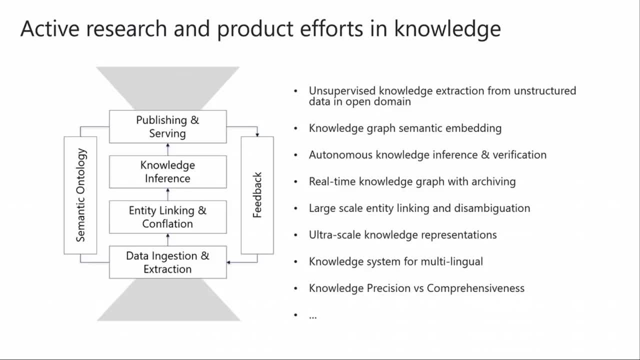 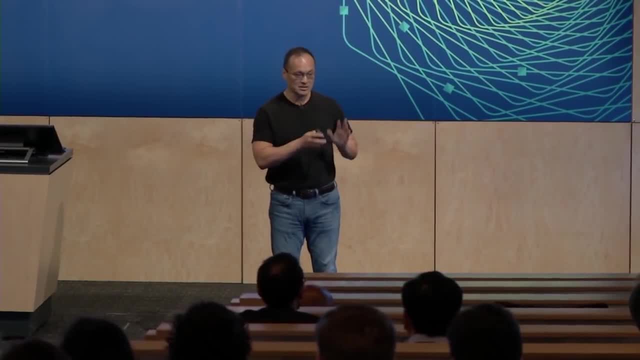 because once you get too precise, you get too brittle and there's no generalization all the way to. you're overly bucketing things and you're like it's not that useful. So these are lots of active research, both within technology product companies in research. 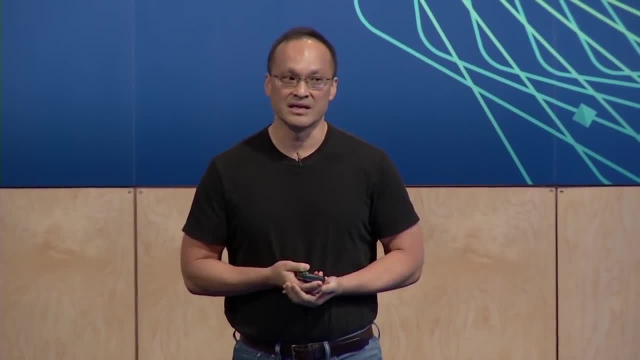 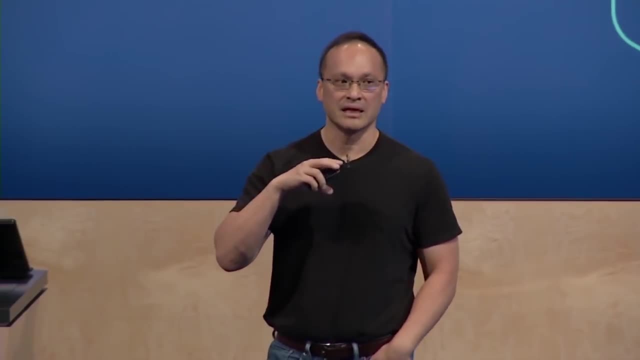 as well as in academia, and I encourage continued innovation. We will look to partner in any and all of these, But let's share a little bit of our learnings. There are many things we did throughout all the systems that you heard about. 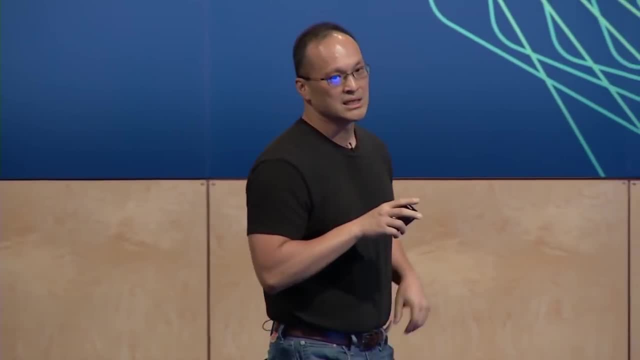 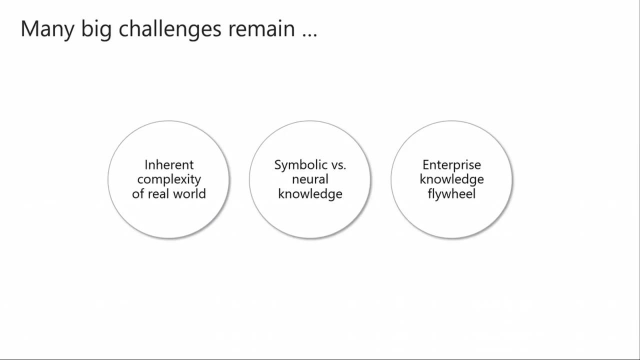 But I'll just pick a couple that I think are useful. One of them, I think, are really hard problems And we've taken steps towards it, But I think it's not a problem that's going to easily be solved. But I'll just use that, hopefully, to tee up the areas where I think there's productive research to be done. 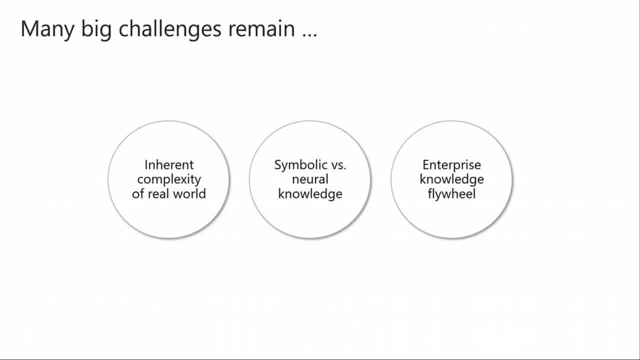 One is the inherent complexity of the real world. We talked a little bit about it. I will share some of the learnings that we had in addressing that. The second is this symbolic versus neural approach, where you can get the best of both worlds. 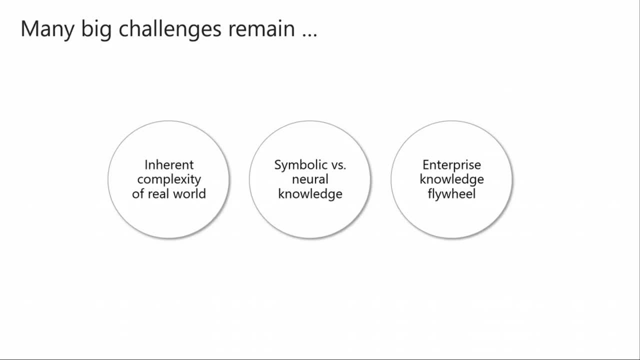 both the ability to now explore the world, but also anchor on the knowledge that exists and the ability to make it understandable, explainable. And the last one, in fact, is something that we're seeing, a huge swell of interest, which is how enterprises can start to take control, to understand their unstructured 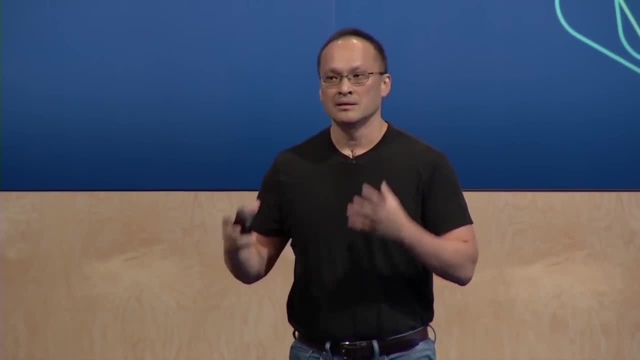 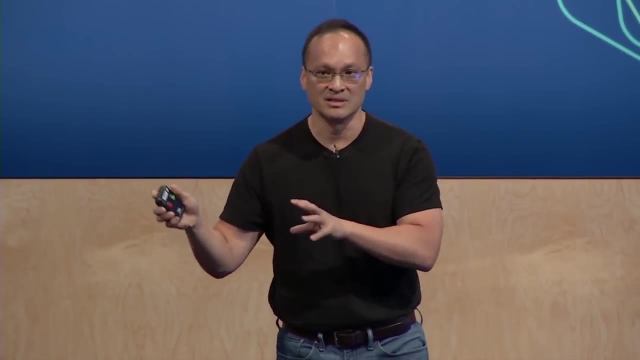 and their digital information assets in a way that makes it available for them to change the way they interact with customers and employees. So I'll just list out some of them. Each one has its own challenges. We've made some progress for it, But I wouldn't say that we've kind of cracked a nut. 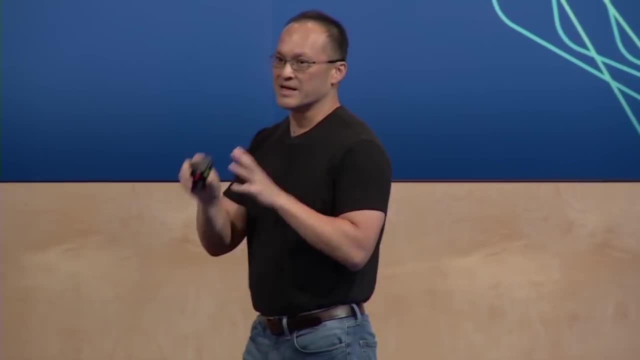 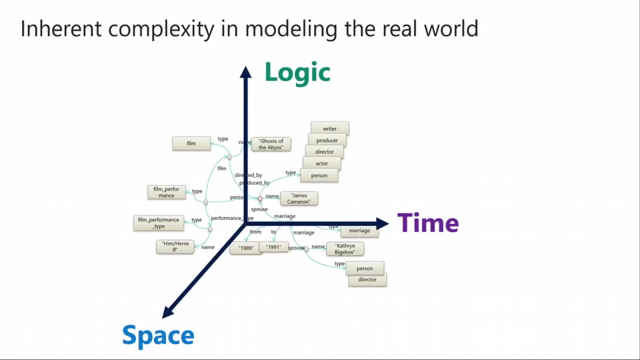 So let's start with the inherent complexity, Just to motivate this a little bit. Working in web search is beautiful. It's chaotic, Nobody has control over anything And things completely change at some breakneck pace. But there are three dimensions that really put pressure on the things we do. 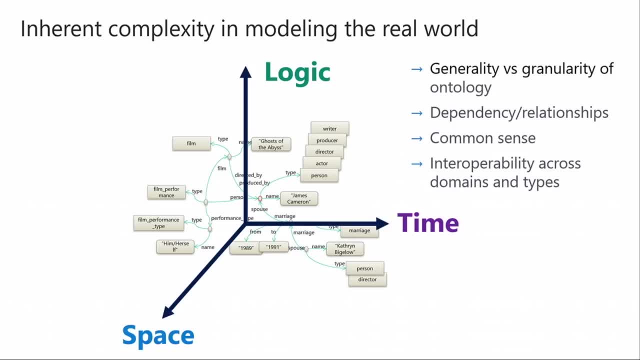 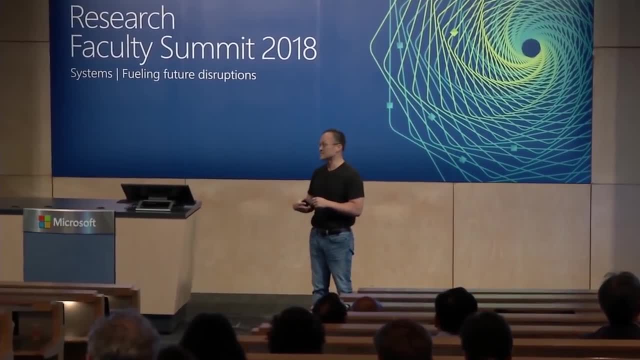 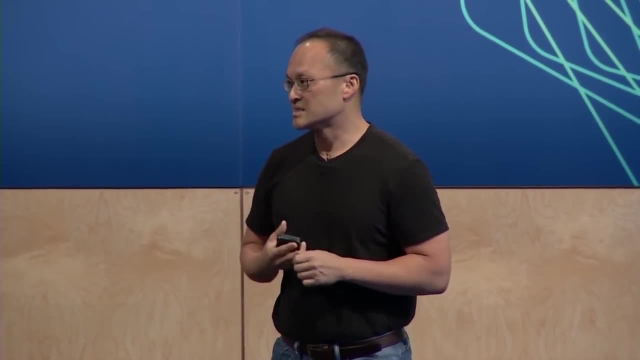 One is just the logic, which is: hey, there's lots of detailed information describing different ontologies across different sites. At what point does it make sense to generalize? At what point does it become common patterns across domains? How do I now enlist domain experts? 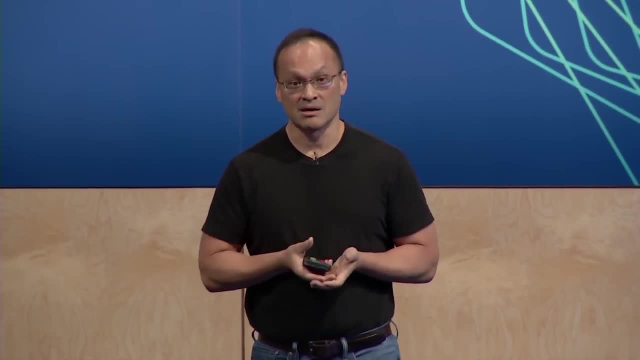 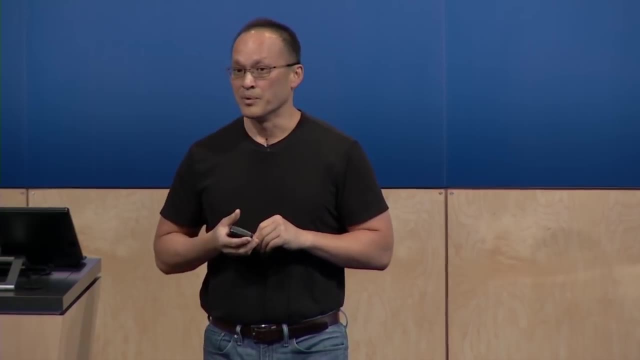 And how do I now recognize that domain experts don't exist in only one company, that in fact it's decentralized and distributed? So being able to tap into that and be able to reason on both the domain specific but also the domain general, These are the common sense. 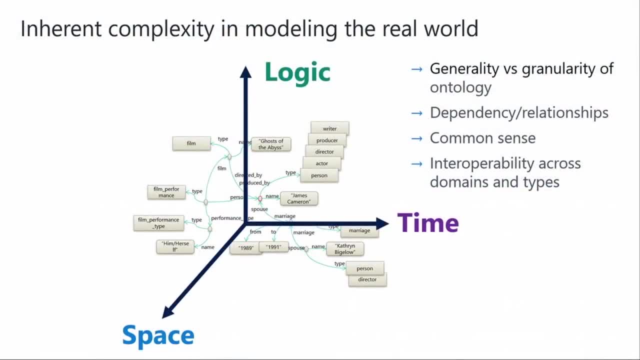 These are the basic things on units, on basic understanding of distance. There are lots of things that I think are shareable and fundamental. On the time dimension, everything changes. It's just that nobody tells us that they're changing And so even coming up with both- the ability to detect the status updates. 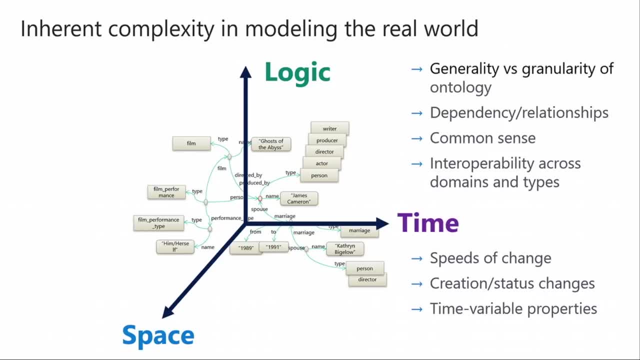 but also be able to see whether you can create even the incentives where they are willing to tell you that things are changing, And so to look at systems to system integrations And in the space, you can imagine that the category and the domain and the scope continues to expand across domains. 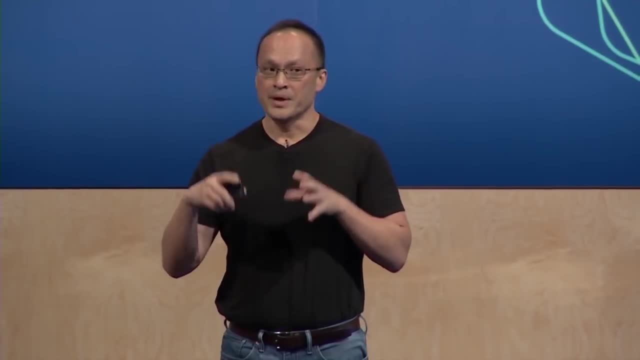 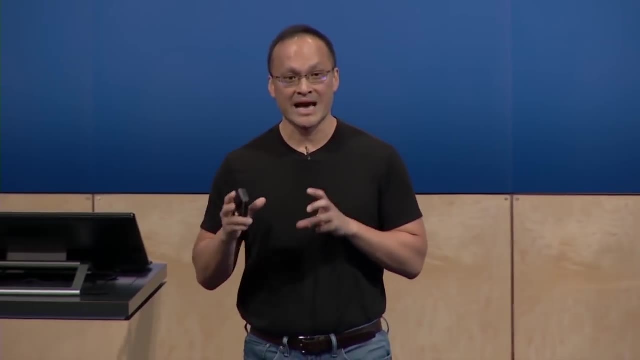 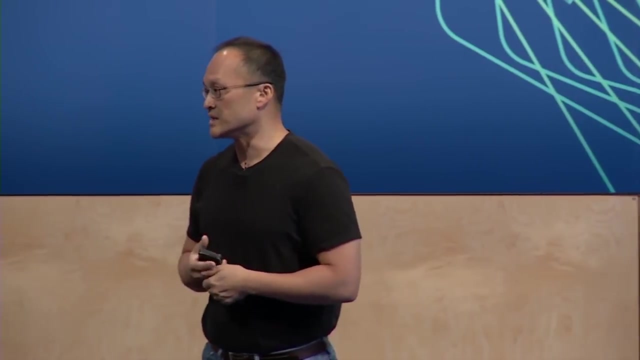 across facets, across entities. So in Bing I'd say that there are a couple of pivotal points in which we've shifted, that really grew our horsepower to tackle some of these. I'll list three of them. The first one is a shift from batch-based conflation to a streaming-based conflation. 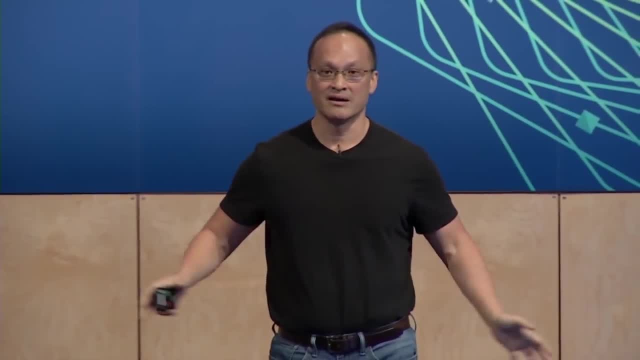 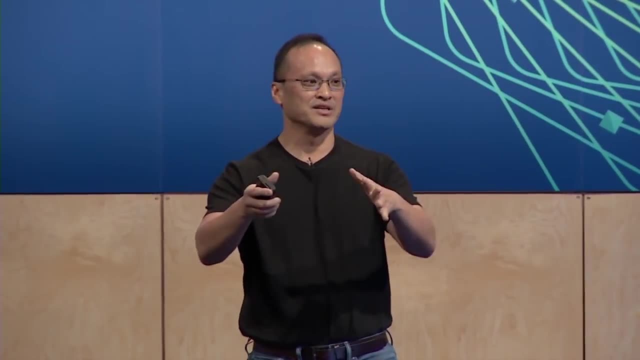 That's a fundamental shift. It's no longer that, hey, on Monday of every week, you take all the data sources, you do a big job and you publish a big blob of a graph. Is it correct? I hope so. 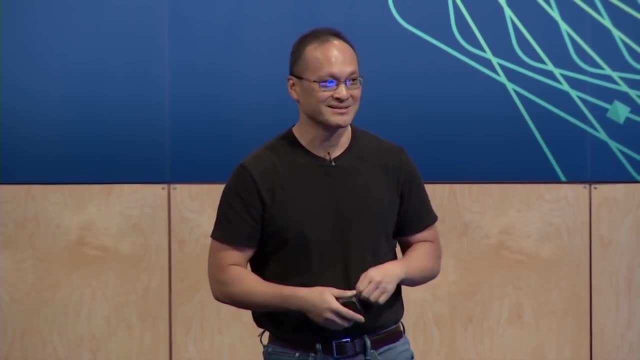 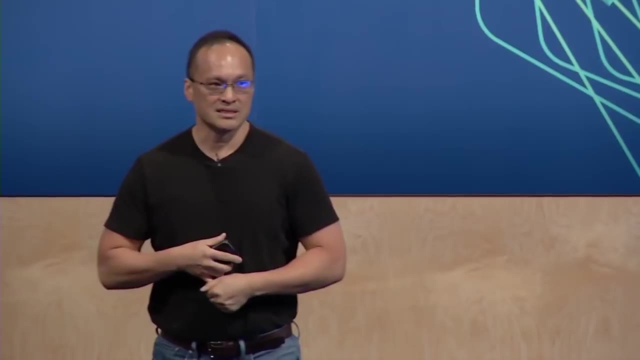 But it takes time. It used to be a couple of weeks, But the web doesn't work like that. It's not a discretized sequence event, So we shifted into a streaming-based system which changes everything. The notion of having an incremental base. 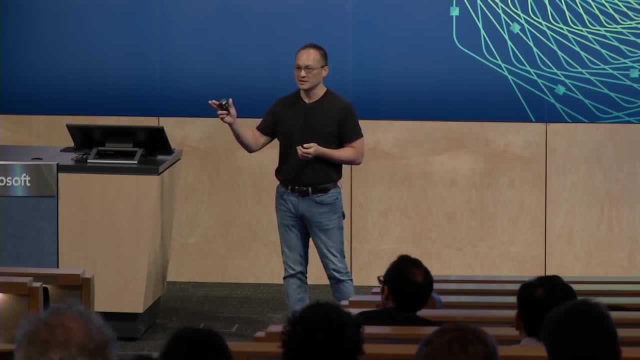 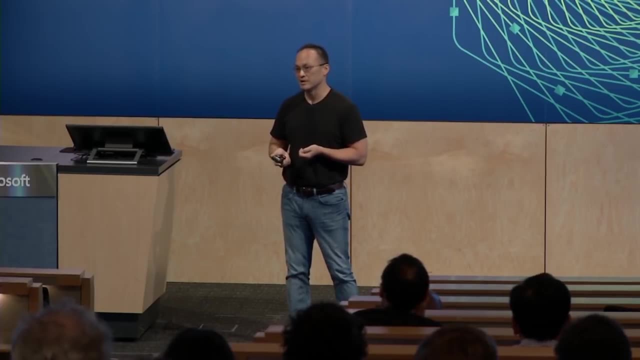 The ability to start looking at updates in a different way, The ability to now look at the incremental conflation and evolution, and even reason about correctness, in a different way. The second shift we have is to start to look at going from the head to the tail. 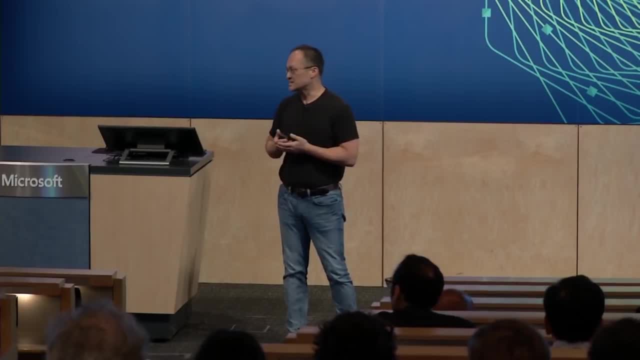 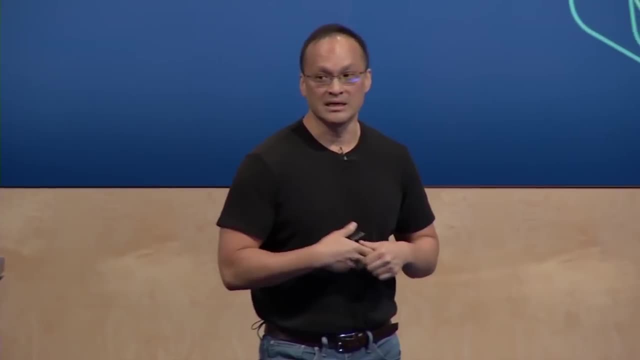 And that requires us to dramatically scale our ability to both manage the ontology but also start to go into deeper site and domain understanding in an automated way. Again, that's an area where we're focused. We're pushing more and more, but clearly lots more to be done. 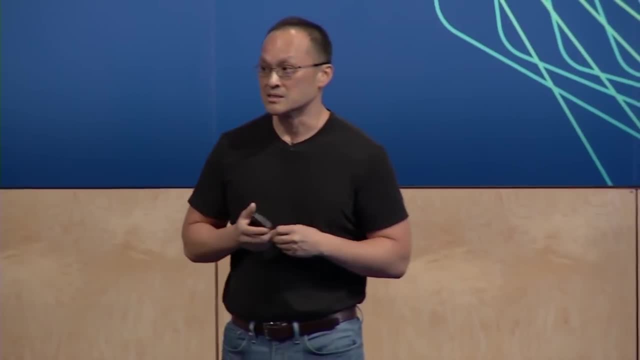 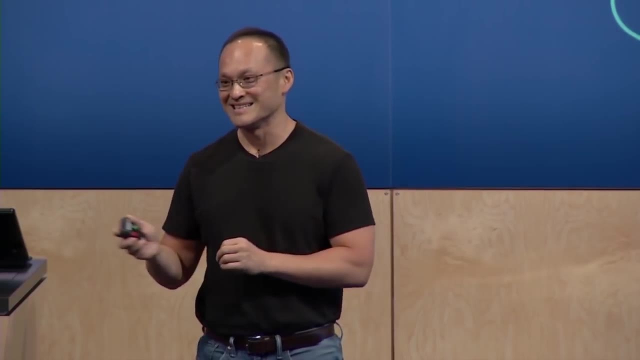 And I think, the last one that I think is notable is our view of correctness, Correctness. It's not like everything out there is correct, or in fact there are different shades of correctness, There are different confidence factors, And yet nobody's there to be the ultimate arbiter. 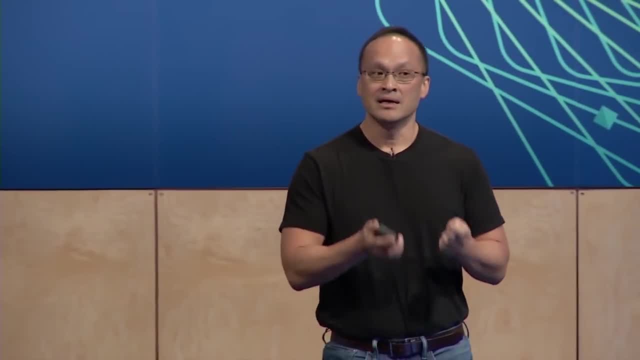 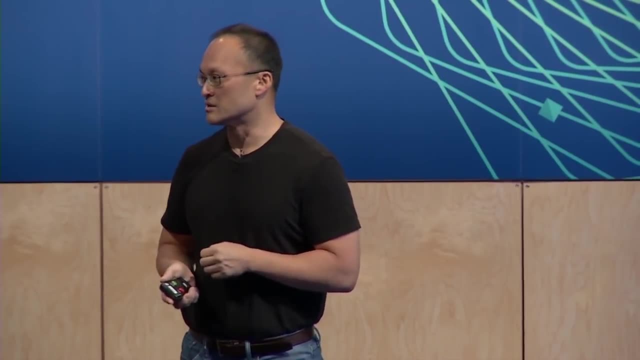 How do we deal with that? How do we now make sure that inputs and changes that are proposed are hypotheses? that allows us to reason, score, understand the likelihood of churn before it goes wrong, So we can then really go into the rest of the system and be able to now get that feedback? 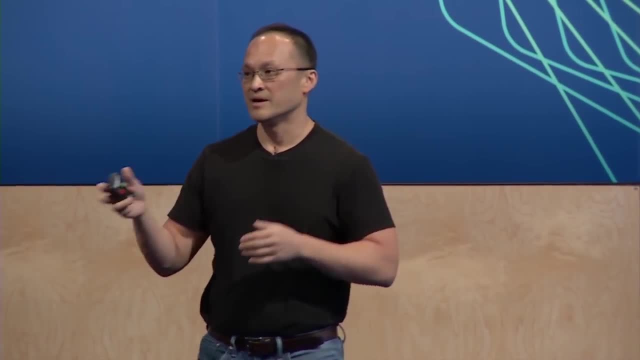 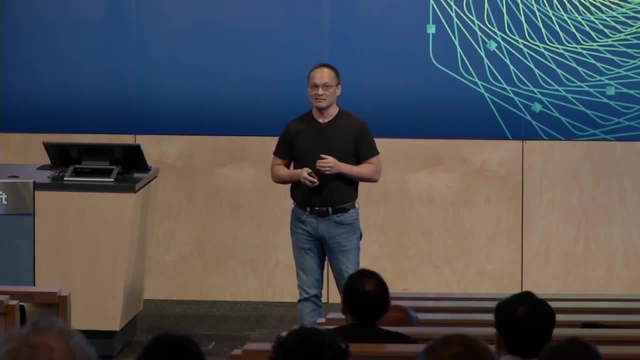 So these are just examples in which the current system continuously evolving. In fact, we like to say the colleague Yuqing Gao, who's in the audience, who's running the Satori team, would say that knowledge is always a life system. 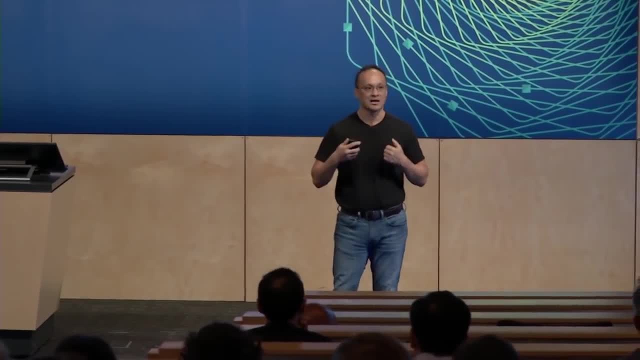 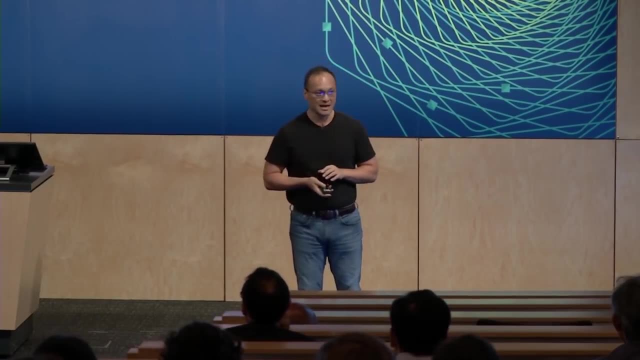 It's a life system. It's not like you build it and it's done. It's a constant, constant evolution. So lots of challenges. You can imagine both systems and algorithmic advances. that allows us to now tackle some of these. continue to grow and evolve with the complexity of the web. 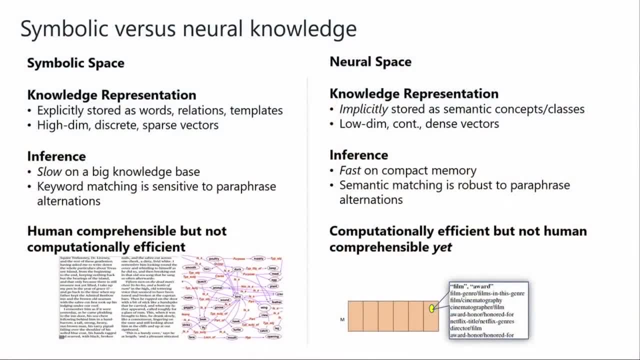 The second area is something we've talked about already, which is knowledge can be represented explicitly or implicitly. We've seen great advances and great promise in the neural modeling of information. We've also seen the advances on symbolic, but there are pros and cons, right. 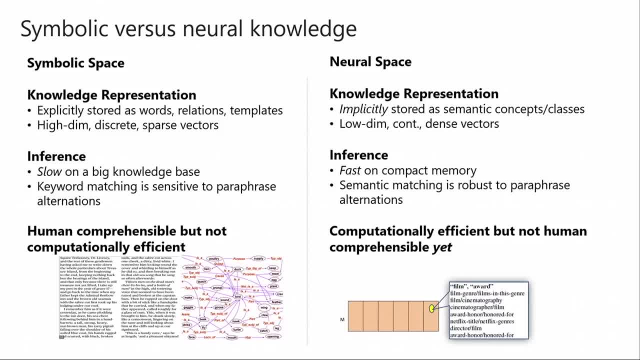 At some point. the discretized representation is probably too big and too hard to manage In the context of now joining against the intent or context and vice versa. And so there are benefits of both. There are benefits of both. One is understandable to humans but really computationally not efficient. 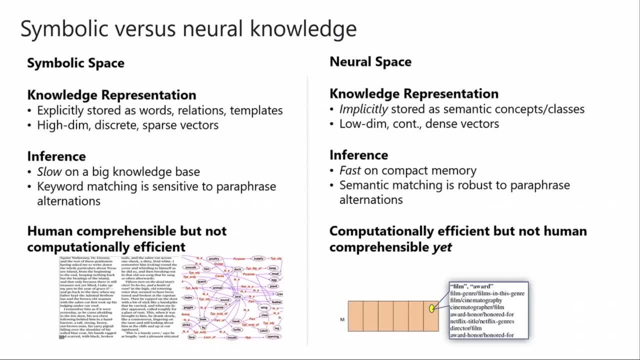 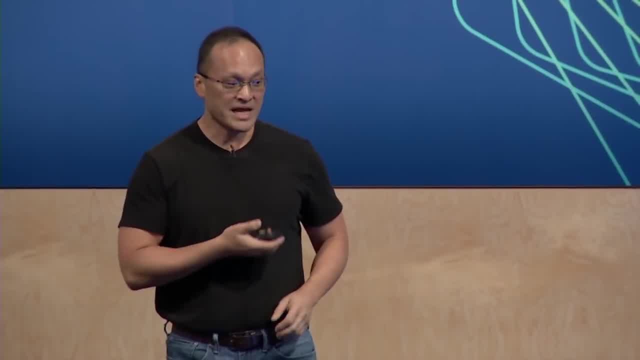 when you start looking at the myriad of understanding, the relatedness and all that stuff. And yet on neural it's efficient, but sometimes you're not quite sure what's happening. So we've taken some efforts. I just list out one example, but this is clearly an active area of research. 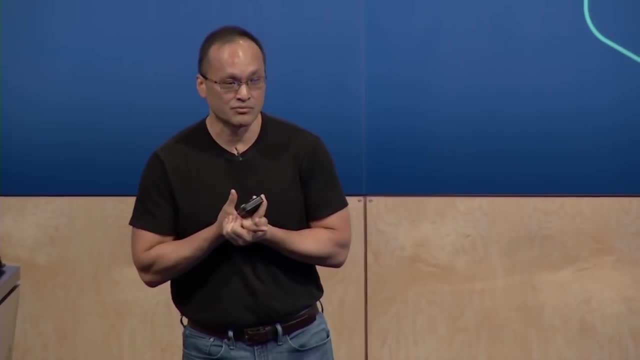 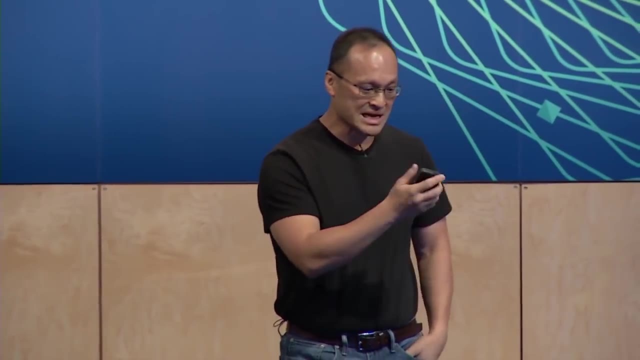 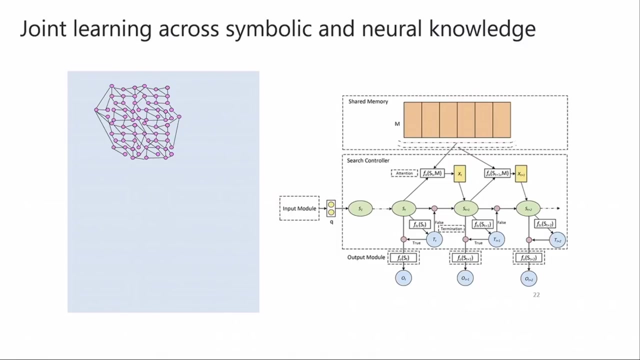 We hope that we'll see some good advances and breakthroughs. We're seeing the need to have actually both techniques applied systematically. One example is: let's say you do have a neural system that allows you to model against some embedding space and you have a knowledge graph. 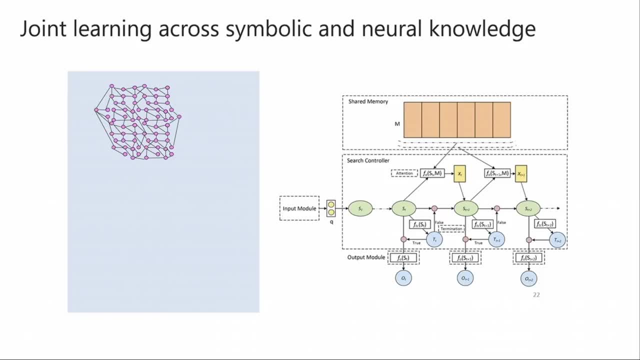 And the question is: how do I now use a knowledge graph to bootstrap my understanding And the way you do? that is, in order to do this mapping, we first understand the hypothesis that are available in terms of the questions and answers in the knowledge graph. 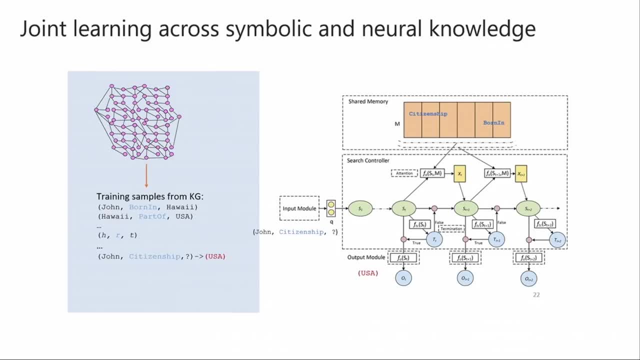 We apply that through the system so it learns and maps it against an embedding space- Oh sorry, I went too fast. Maps it against an embedded space. So over time you can imagine that through techniques like this or similar we can hopefully start to now bootstrap and connect. 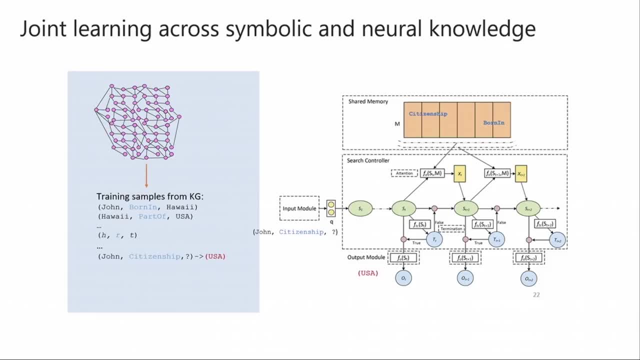 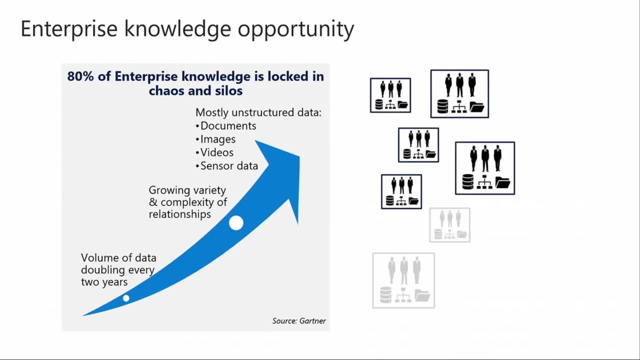 and hopefully even do this in a much more integrated way. But this is an active area of research that I encourage all of you to look at and see what we can do together. Then, on the enterprise, going back again on this enthusiasm that people have around enterprises and their knowledge, 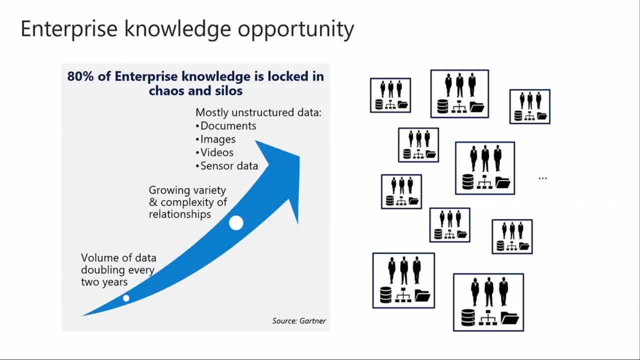 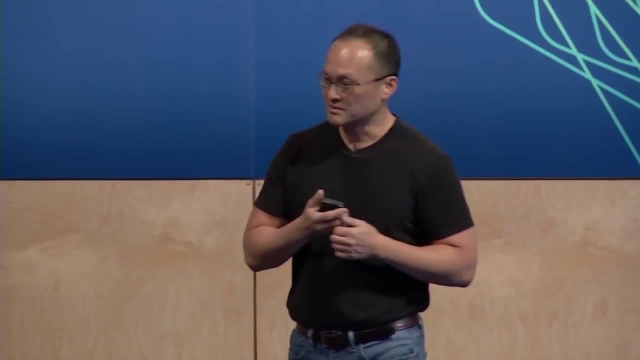 but lots of unstructured information in people's communications, in the documents people write. People don't write in structured facets and fields and certainly they write it with different variant degrees of quality. And there's a study from Gartner that says over 80 percent of people in the United States 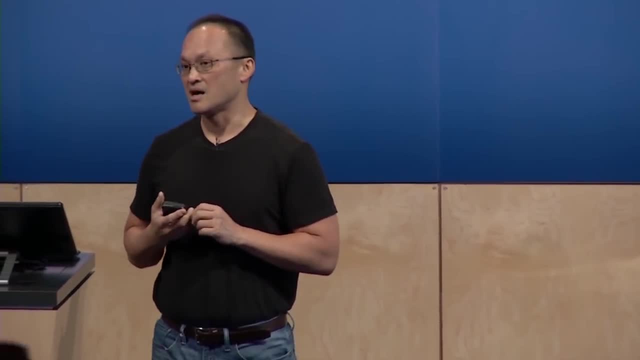 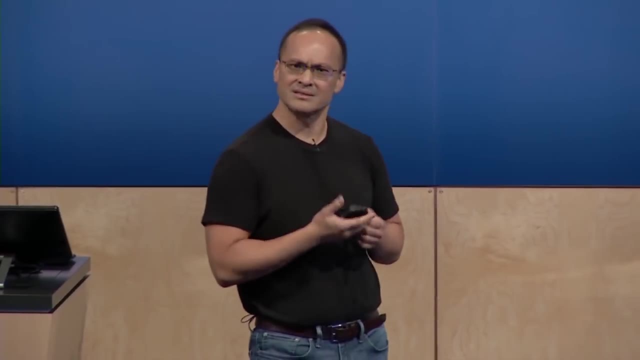 and over 80 percent of enterprises' knowledge is locked and unavailable for broader use, And that's a staggering number. You talk to IT, you talk to the companies. they're saying: you know, I don't know, like it's all kind of black box to me. 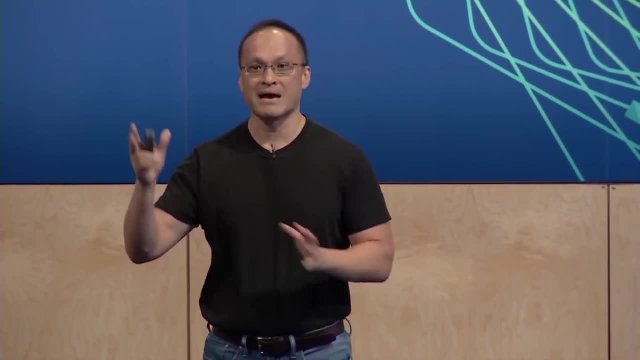 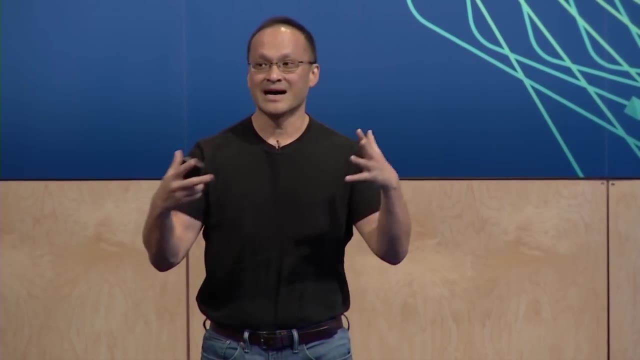 And the data continues to grow. So, in the world in which data is growing massively, they're seeing tremendous value, but they can't make sense of it because they're stored in different ways, written in different formats and not conflated. What do they do? 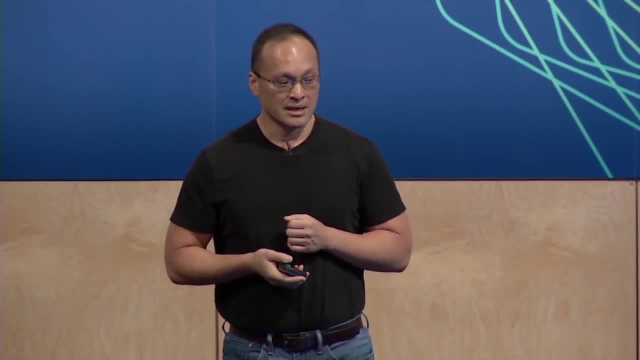 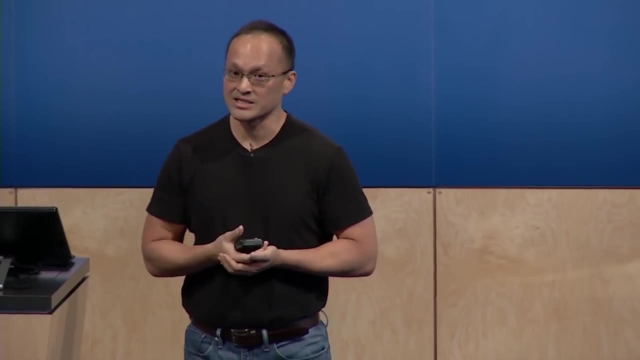 And that's a real challenge, but that's also a real opportunity, And so let me give you one example of how this is coming to bear. So about late last year and early this year, we engaged with Publicis, which is an advertising agency. 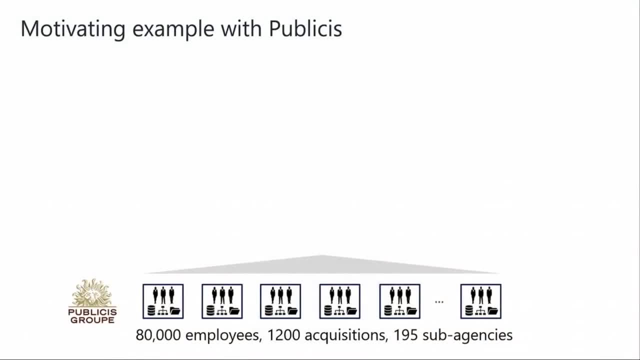 They have lots of agencies. They acquired like 1,200 acquisitions. They have 200 sub-agencies. They have 80,000 people, Each one. you can imagine having their understanding of clients, their understanding of the work, the advertising campaigns. 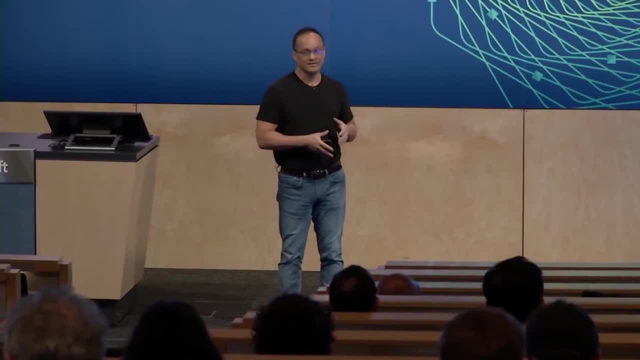 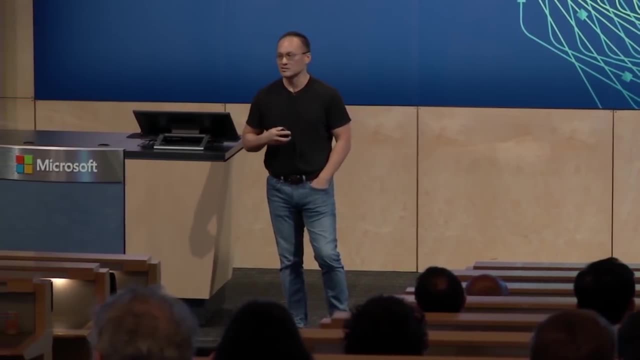 their deep understanding of brands, Their talent profile. So it's lots of information. So, in their case, what they're saying is they want to see the benefits of scale. Here's an example of a digital transformation where a company is really at a very fundamental level, which is the fact that I have 80,000. 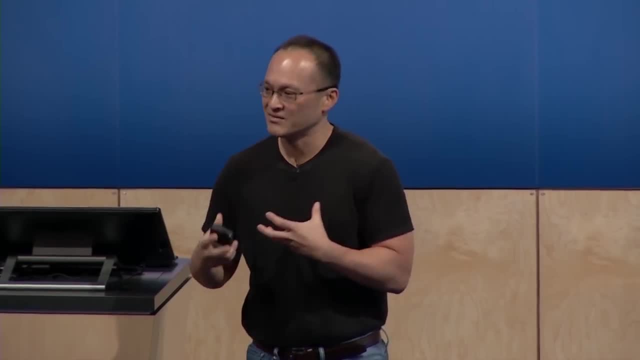 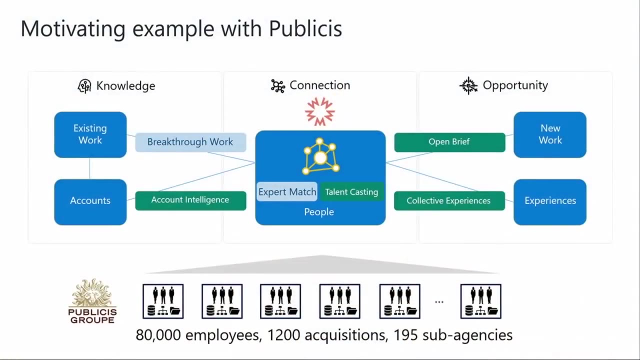 and 1,200 acquisitions. how do I get scale advantage? Well, to get scale, you've got to bring that re-information and that people asset together, And so what we're working with them is to start to bring together their understanding of their talent. 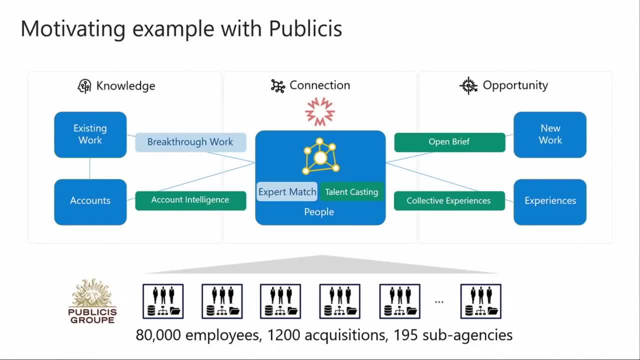 understanding of their accounts, understanding of the work they've done, and start to create really this ability to now reason, map and correlate. This is something that I'd say: that if you're an online company or a commerce company, you just do this. 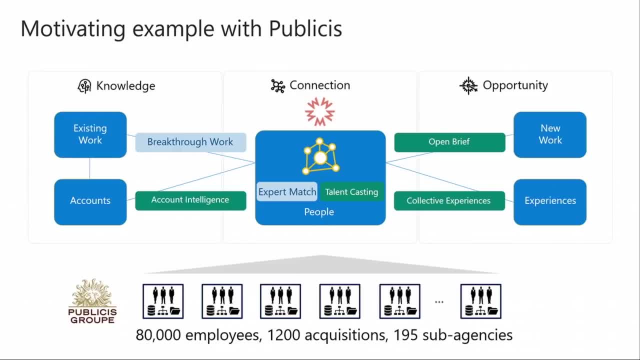 But for enterprise this is all new stuff. This is all new stuff And in fact it requires a deeper understanding and appreciation of how do you reason with knowledge and to get that flying. But in the course of these engagements, we also recognize that enterprise knowledge is unique. 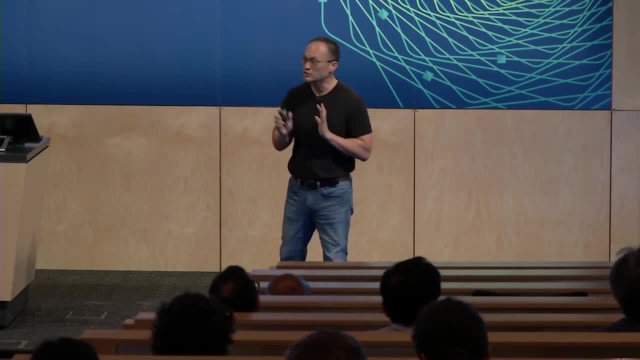 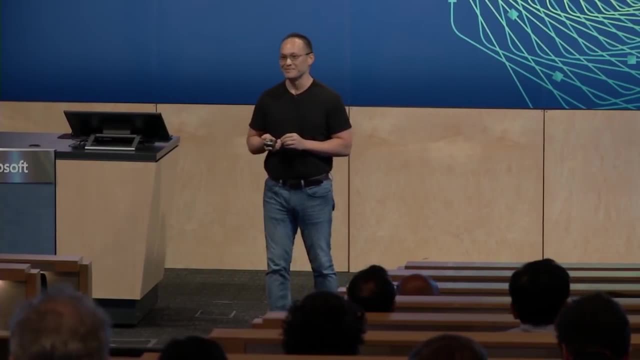 It's unique. It's got its own unique challenges in two dimensions. One is: data in enterprise is not readily accessible to everybody. It's not like it's a public web document that anybody can read. This is private email. This is documents that are sensitive. 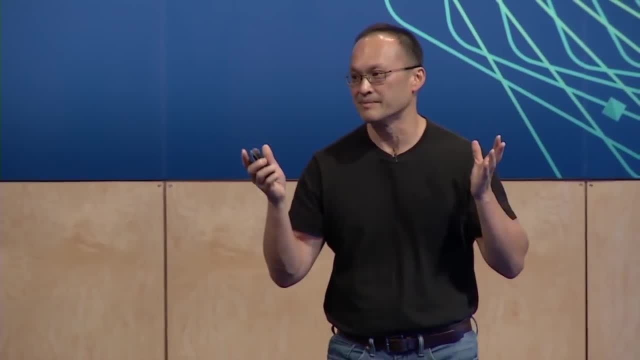 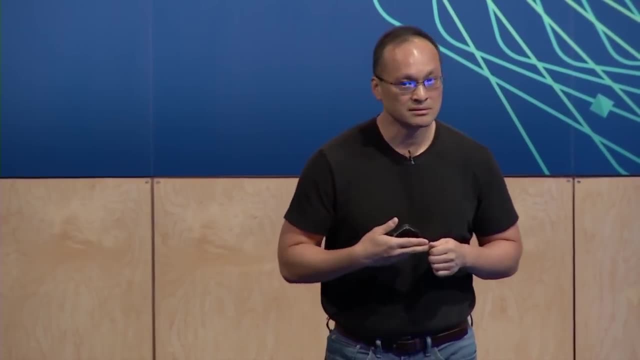 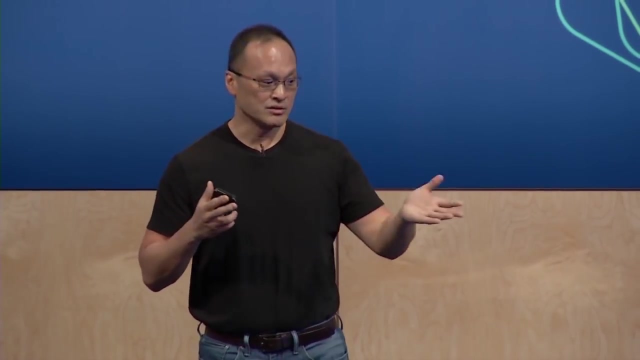 This is ACP documents. There are lots of information that you just cannot even see, And enterprises have obligations, both in terms of regulatory compliance. certain financial data, certain HR data, can't be shared. There are certain encumbrance commitments. 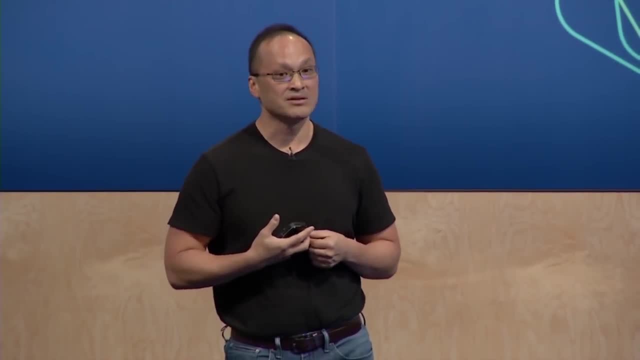 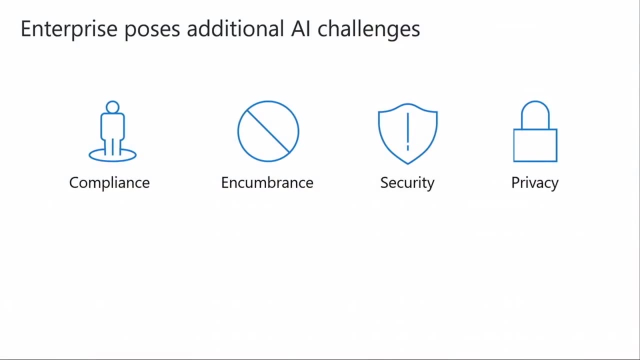 If you get data from third parties, for whatever reason, you have obligations to limit its scope of use. You have security considerations- Different people have different access rights And you have privacy- with GDPR, That ability for end users, both employees and customers. 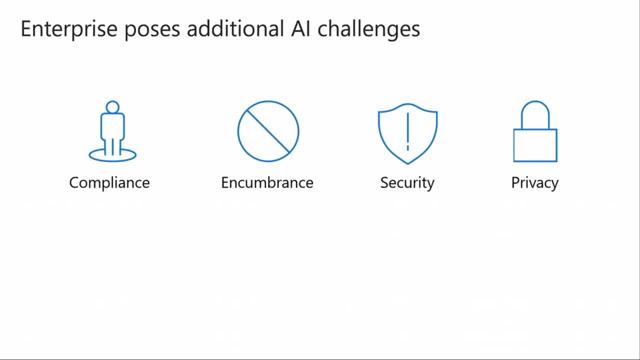 to now have control, and that ability to influence that data is critical. So all of this is creating a case where, in many cases, we're not quite sure: how do you build an AI model when you can't reliably see the data? That's a real challenge. 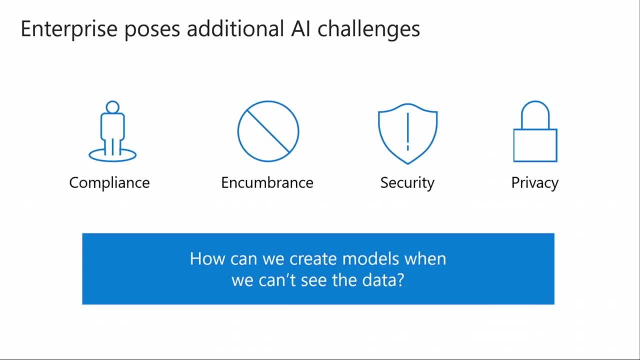 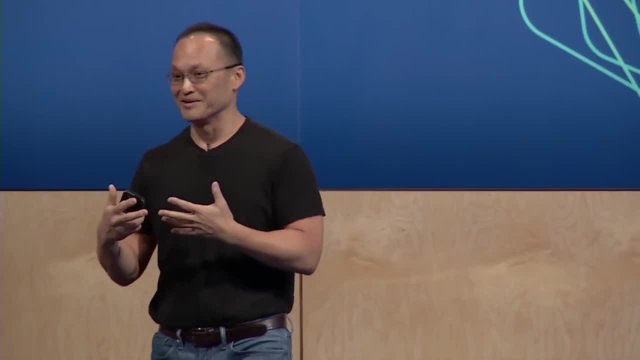 So within Microsoft, in the office, for example, we have different practices. We keep the highest standard and we in fact enlist the users, in this case Microsoft employees, to contribute a portion of their email for us to build the models. 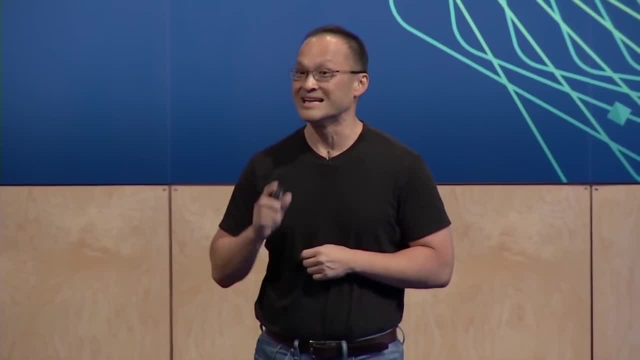 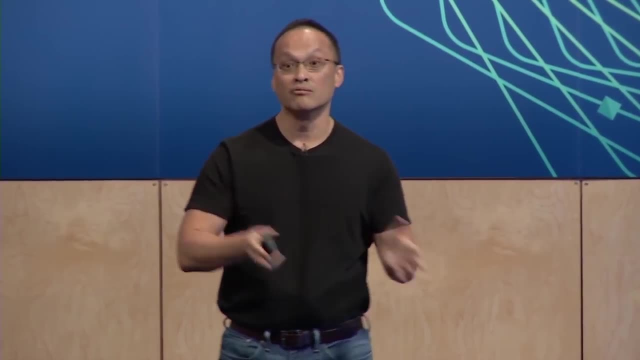 But you can imagine new techniques and new approaches are needed for us to get beyond this hump, And that is not necessarily the same algorithms and approaches that works in the web and in public data can work in the enterprise setting. So lots of innovations around multi-party secure computations. 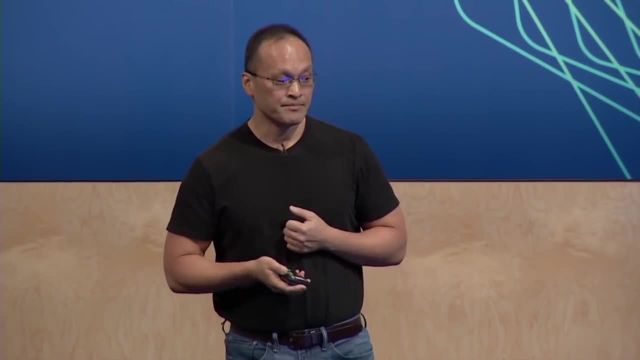 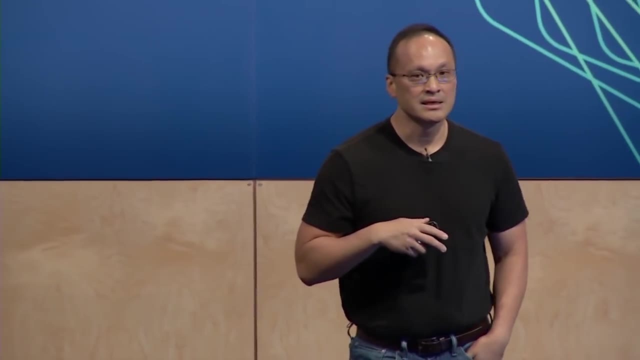 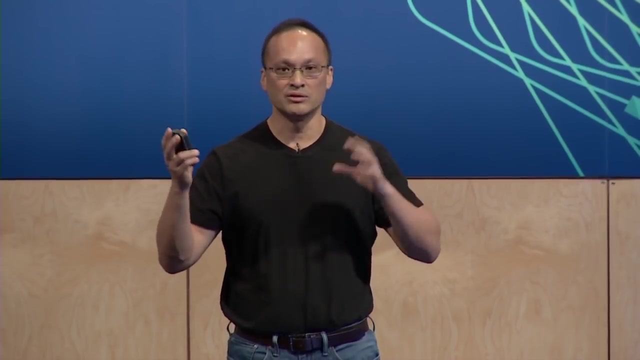 private computations that are potential here, But perhaps the most challenging is that their access to the data within an enterprise is of mixed degrees of quality and completeness. It's a bootstrapping problem. Hey, I'm interested in doing all this, but the data may not be clean. 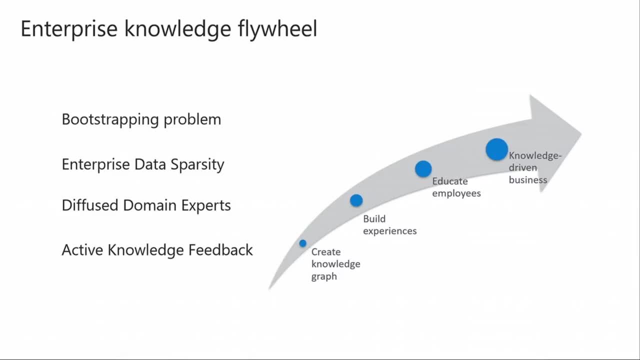 It has the varying degrees of quality. It may not be complete. In fact, in order to bring that domain expertise, it's typically diffused and it's not any one organization has that depth and certainly not the talent that knows the domain. 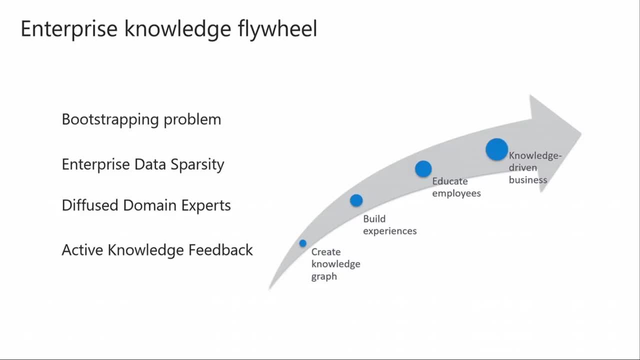 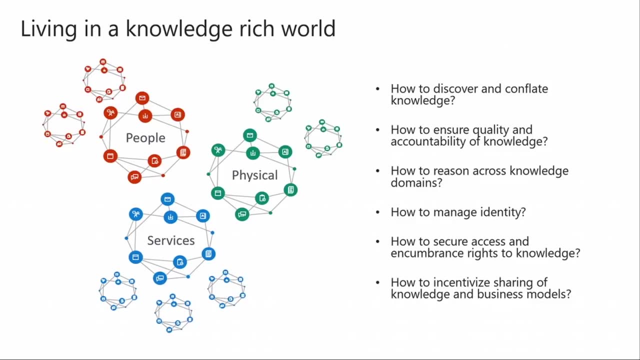 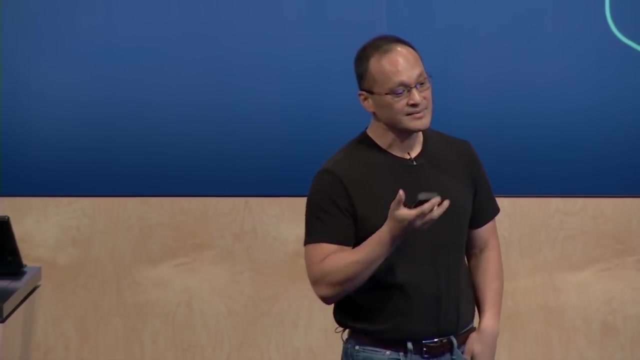 doesn't necessarily understand the systems. So, with that, I would say, we're at this stage where we are seeing this desire to transform, and knowledge is increasingly this fundamental capability that is starting to reshape the way we think about information and interactions, And so I would just say that imagine, fast forward, a couple years from now. 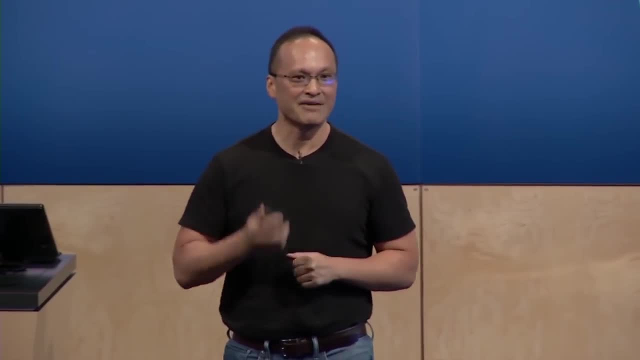 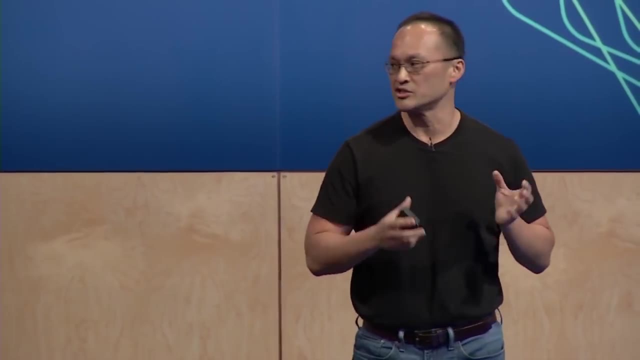 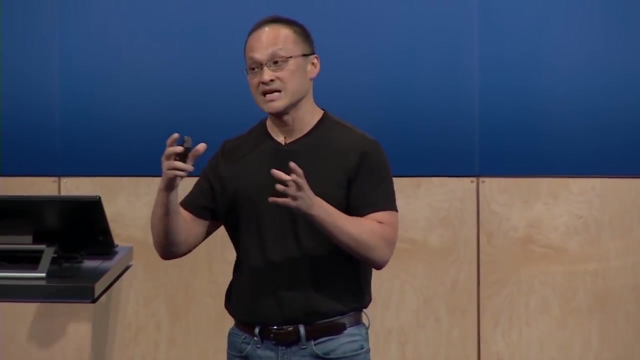 where you're saying: imagine you're living in a knowledge-rich world. Every person has behind him or her this rich knowledge graph of their activities, interests, interactions, relationships. Every object, every physical space has its own knowledge graph That's created from different organizations for different purposes. 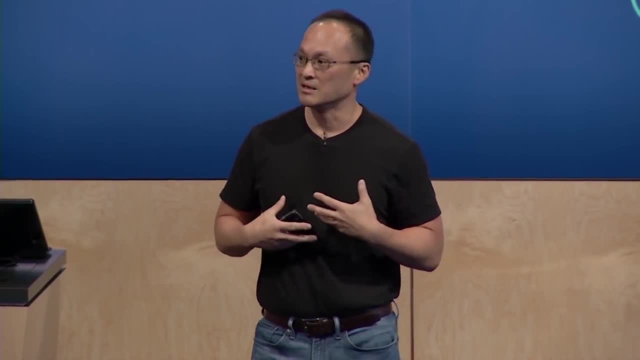 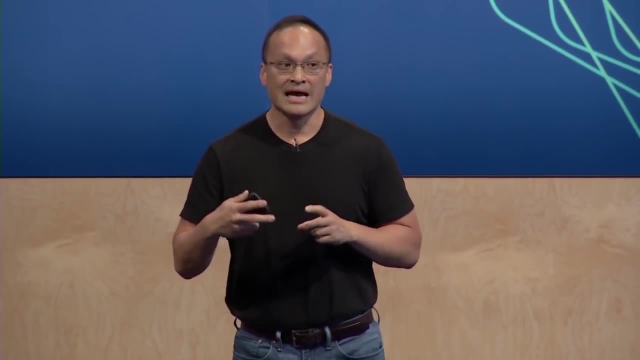 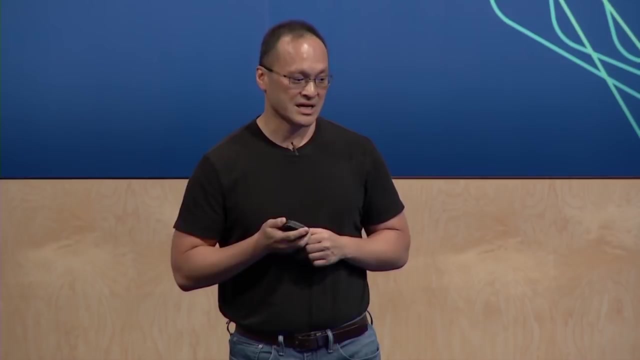 and every service has its own associated knowledge. Bringing all that together in some coherent way- where they're multi-party, they aren't working together and yet you need to now attest and navigate and interact in a fluid way across- is a real opportunity, but it's a real challenge. 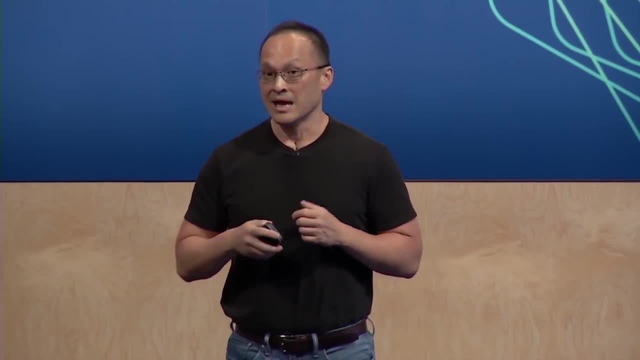 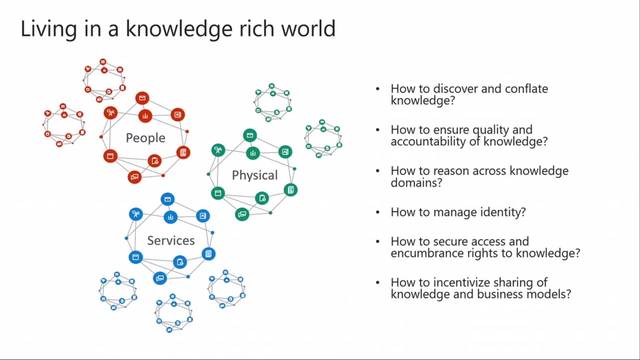 And so, with that, these are some of the questions and domains, and it is hopefully there to inspire that I believe we are heading in a way where we are going to see a knowledge ecosystem. We're going to see knowledge technologies for both the production. 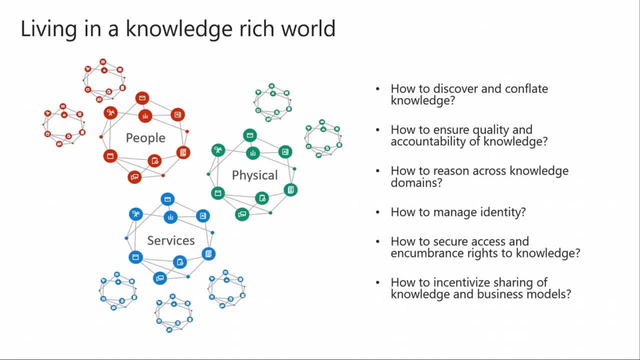 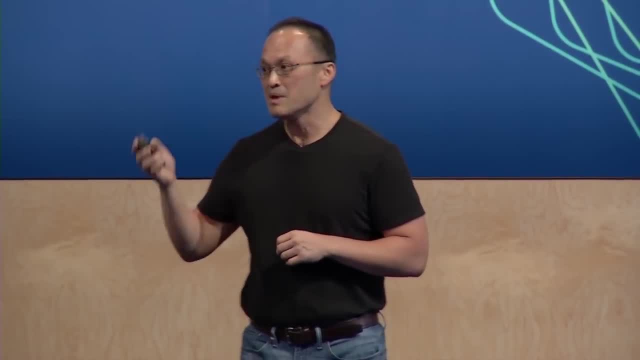 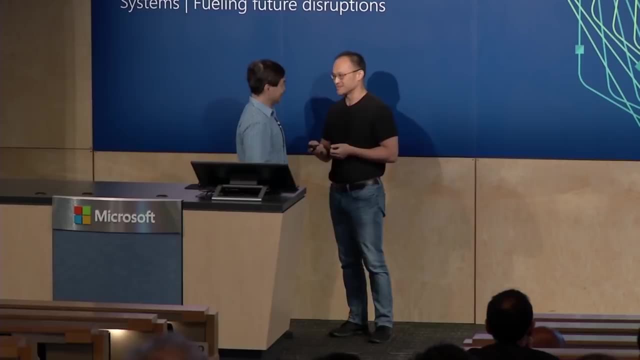 and the consumption of knowledge. It will require different teams and different people to work together, and we're still early in this research and technology innovation wave. So with that, let me bring in my colleague, Kwon Sung, to come talk to us about one example of how we want to push on this process. 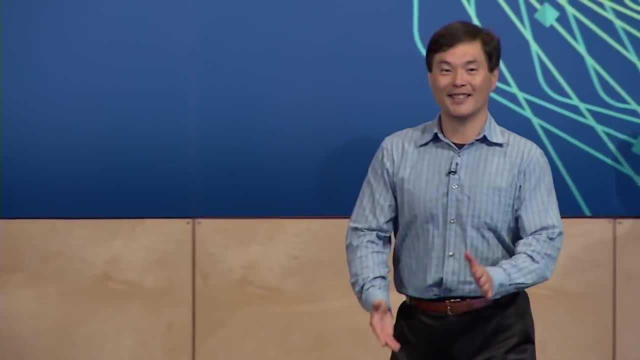 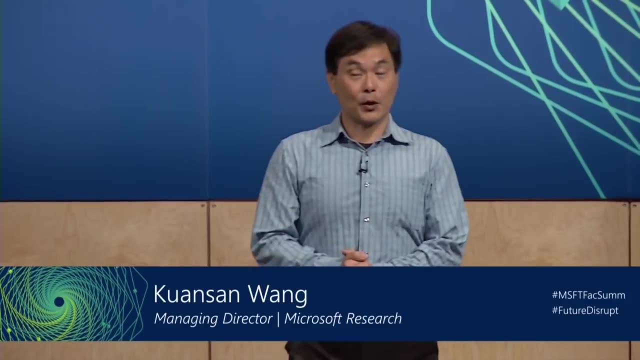 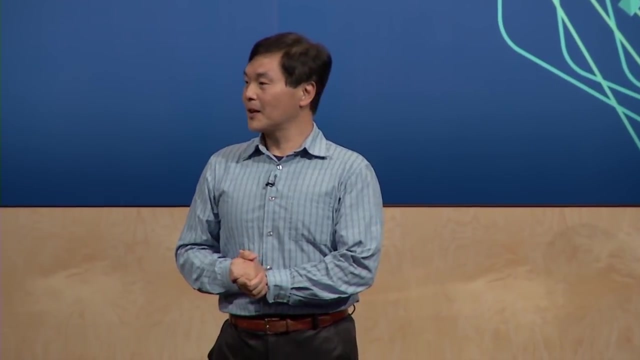 Great, Thank you. Thank you, David. Good morning. It is my pleasure And to be here to talk to you about knowledge system and AI. After all, it was eight years ago, in this very venue, Microsoft Research Faculty Summit in 2010,. 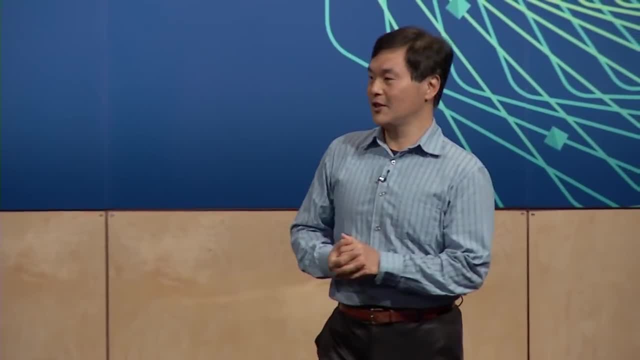 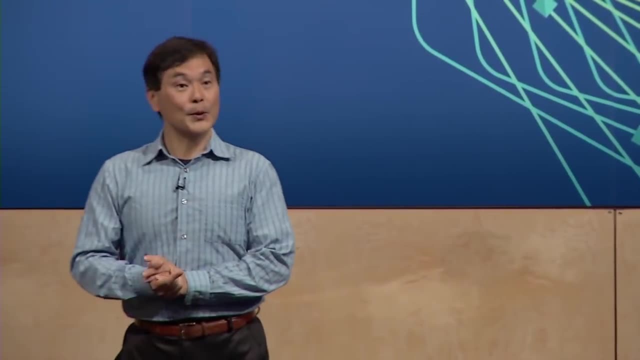 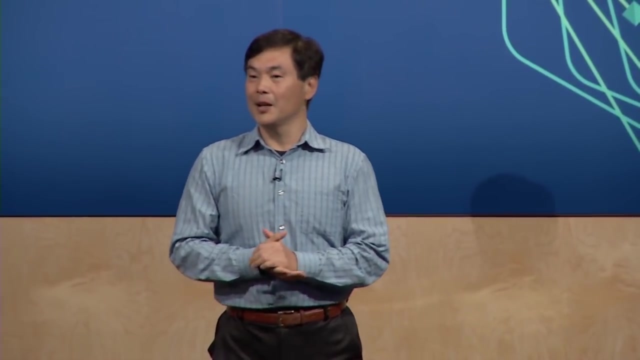 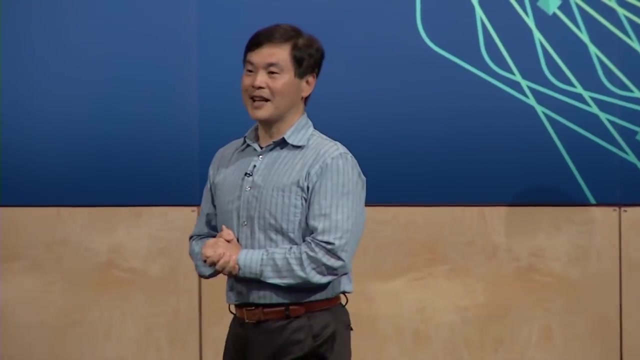 that we first described our ambition to teach the machine to acquire knowledge from the web by itself. In the ensuing years, in addition to the continuing investment from Microsoft that David has just described, we are glad to see the little idea presented eight years ago has received industrial adoption. 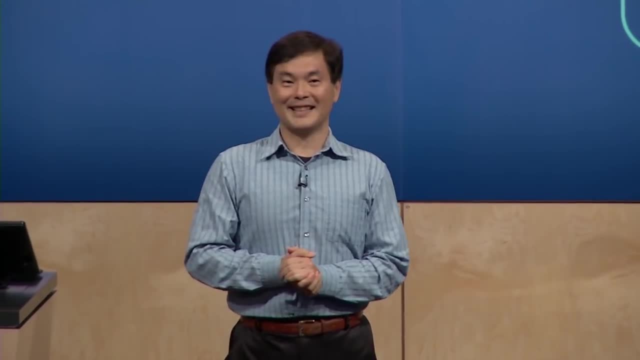 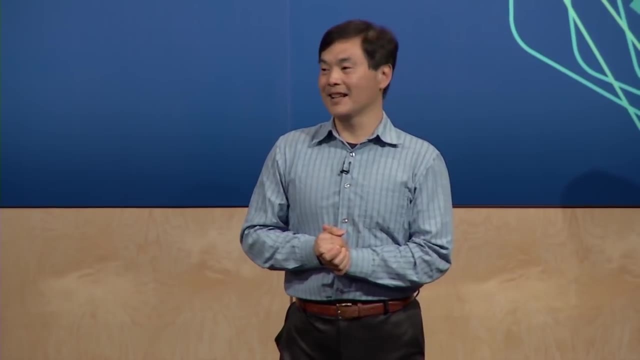 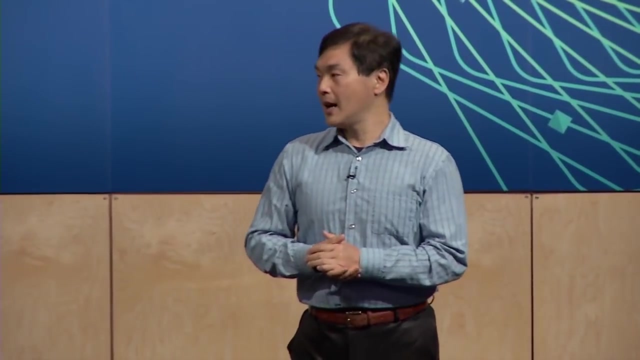 including the Google Knowledge Graph efforts, two years after our Faculty Summit and the Baidu's announcement in SIGIR 2014.. So today, it is my pleasure to be here to share with you the next evolution for us: to share the resources we have from the industry. 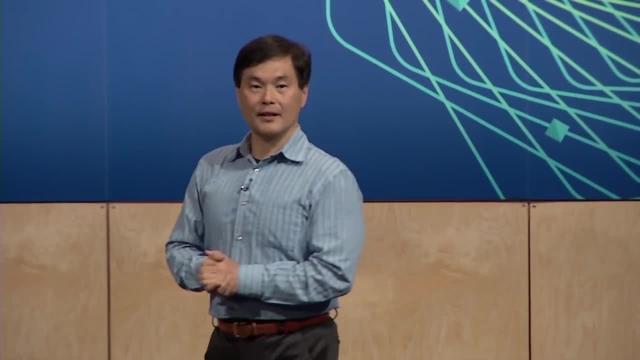 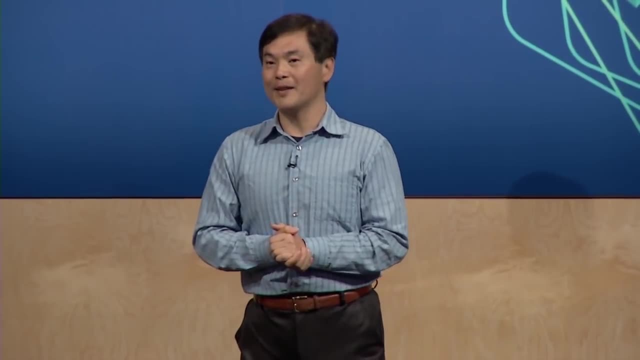 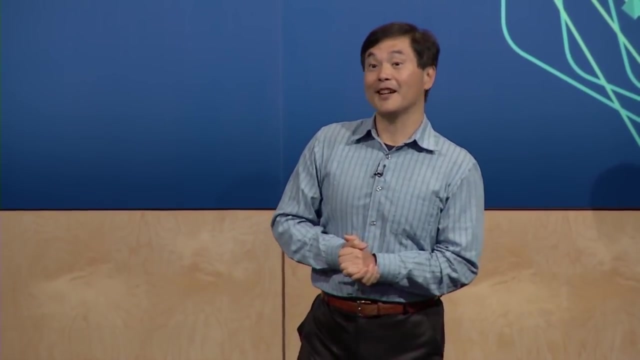 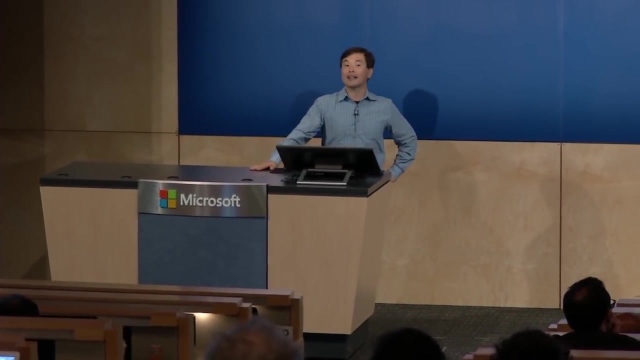 research lab that consists of a dataset and open source tools that can facilitate research, with the hope that more of you can join us in the journey to advance the state of knowledge systems and AI research. So let me start with the datasets. This is, as David alluded, Microsoft Academic Graph. 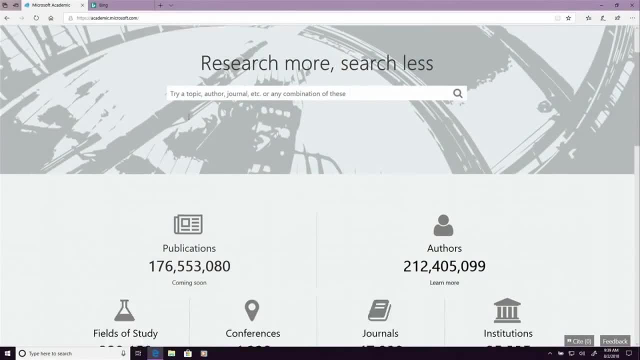 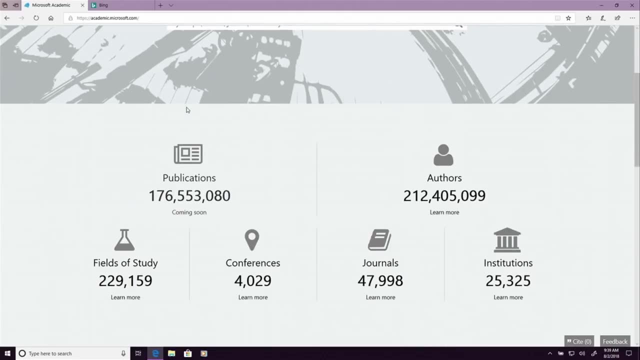 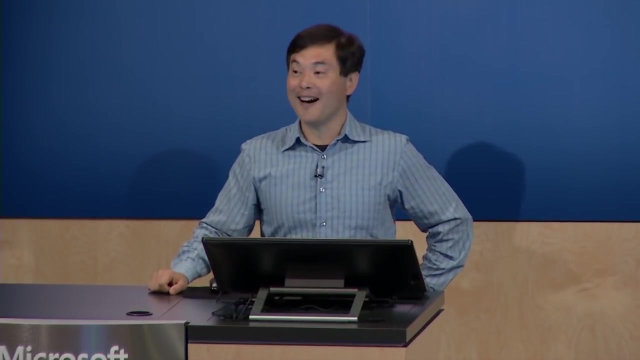 Like the Bing Knowledge Graph, it is built by extracting the knowledge from the entire web, And so we have the scale to cover all the scholarly communications published in the past one and a half centuries. So, speaking of an ecosystem, this is a knowledge graph that every one of you is already on as a node. 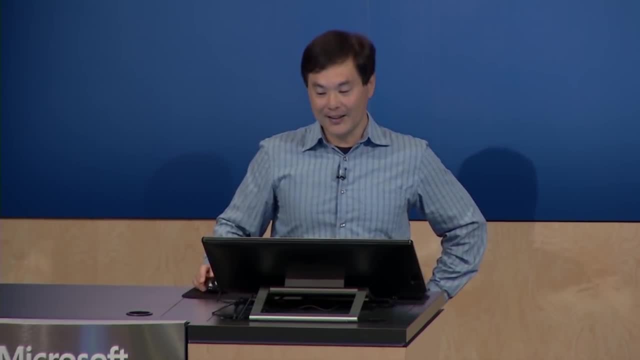 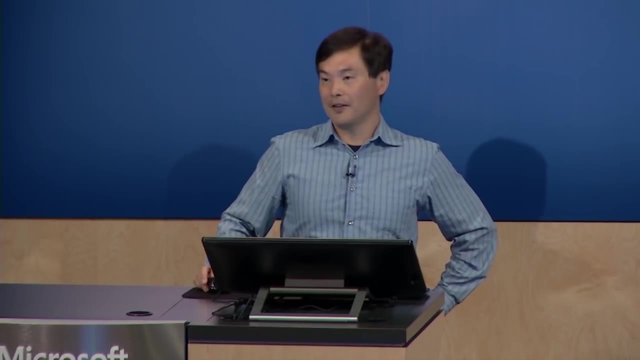 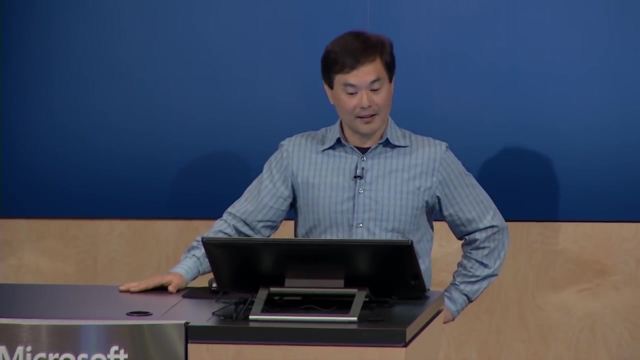 So is every student that you have supervised, every institution that has supervised, sponsored your work, all the journals that you have cited and the conferences that you have gone to present your work. So, as you see, the number is increasing, is massive and it's growing rapidly. 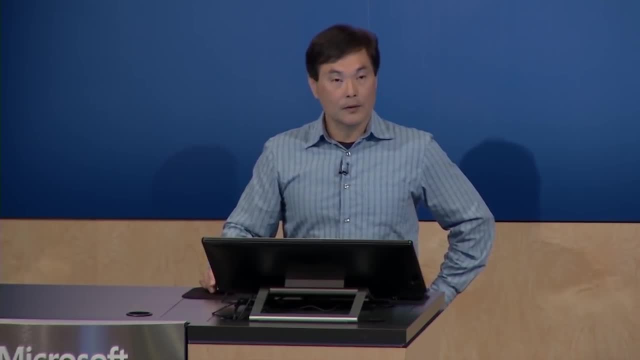 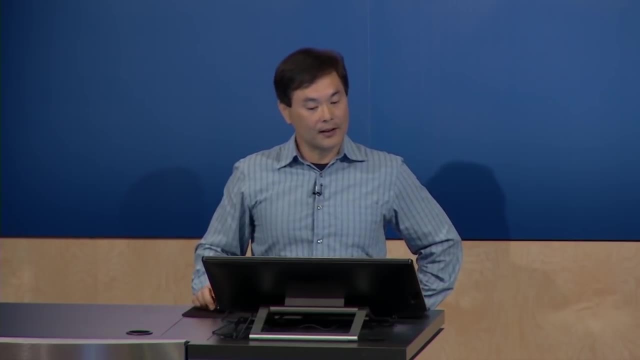 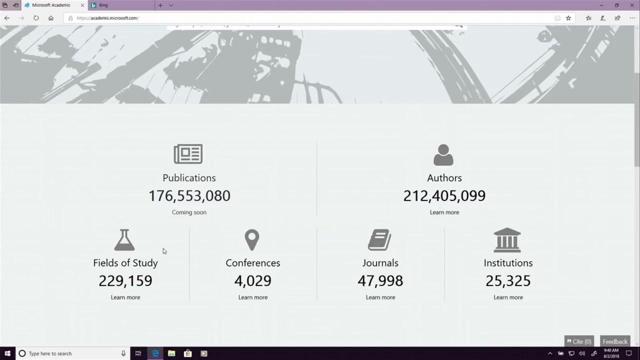 All right. So one of the benefits of sitting on top of Bing is we have the broad coverage. So, as you can see that we have teach our machine to go beyond computer science and to cover more than 200,000 fields and subfields. 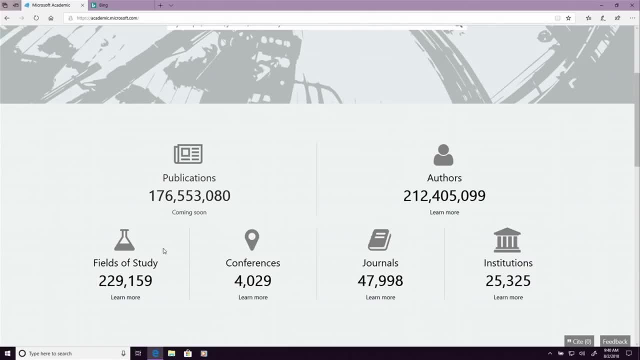 including medicine, art, history and so on. This broad coverage turns out to be very important for research managers and your provosts and deans, maybe to understand the impacts- broader impacts- of our research and for many decision makers to determine the investment or research. 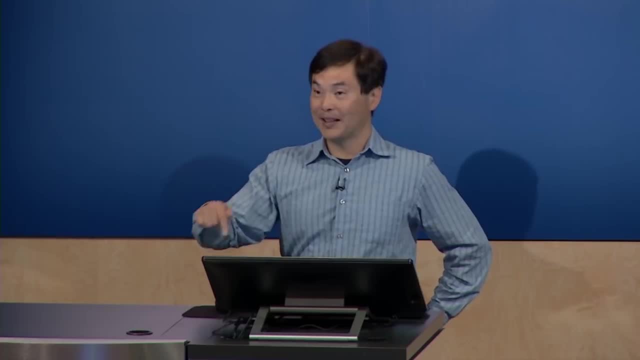 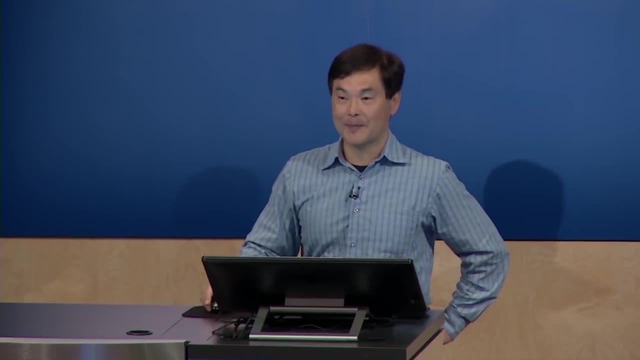 So I hope that this gives you some incentive to take a look at the data, but for us it gives us a strong incentive to push the technology to make sure the data quality is. here Bing researches ourselves. We naturally have published a paper. 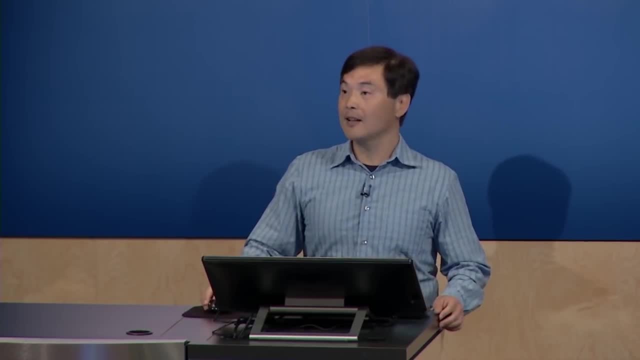 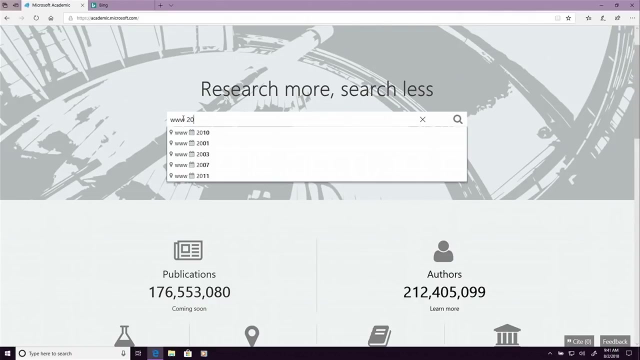 to describe how this graph is created and what we envision it can do. And the easiest way to find this paper is to remember it is published in www.2015.. And so you can just in this system, you can just type www.2015,. 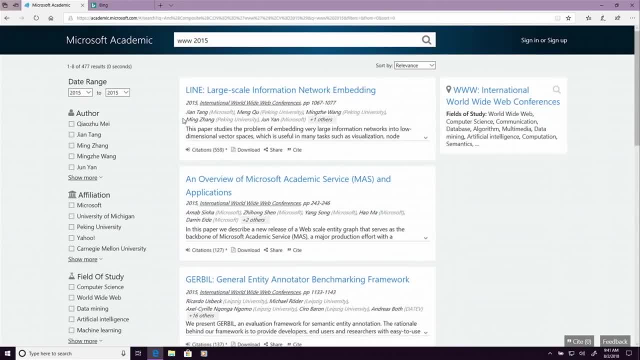 and right there you can see all the papers published in this year, and our paper is actually currently ranked number two on the search results. So there are two things immediately you can notice. The first is the query: So by recognizing the conference as a first-class citizen in the knowledge graph, 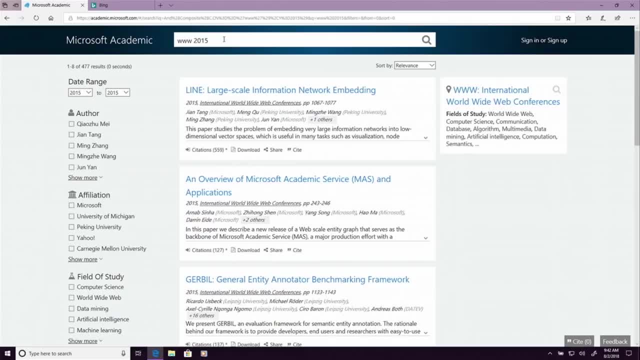 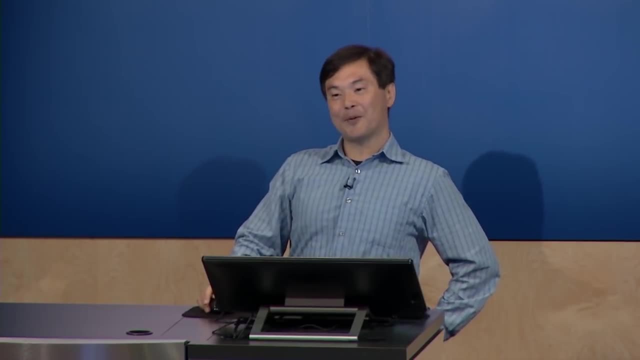 we can actually do more query, better search experience by not just keyword matching the query terms to the title, And I understand that many of my colleagues have been using this feature when they are running the test of time awards committee to find papers and their citations. 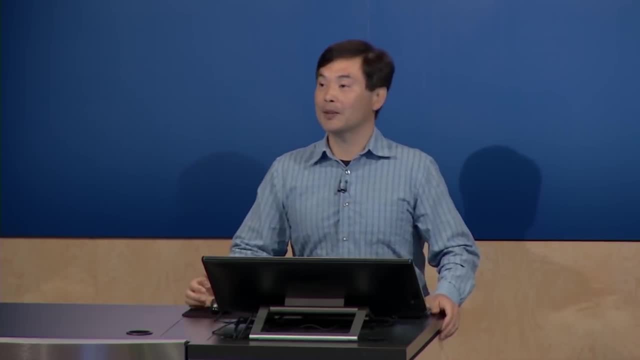 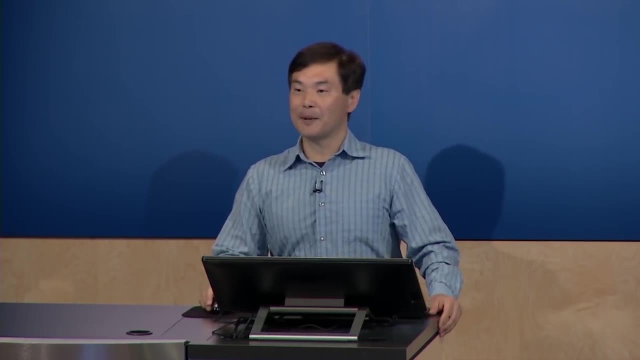 for a particular venue And this tool. you can do it with a single query in this tool And I'm also glad to report for the past two years since I discovered this new usage, I've been watching it and our ranking system. 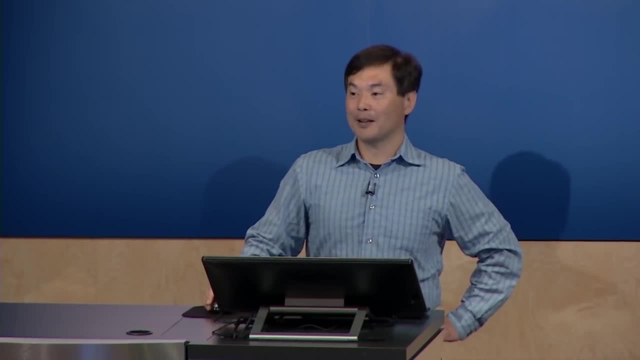 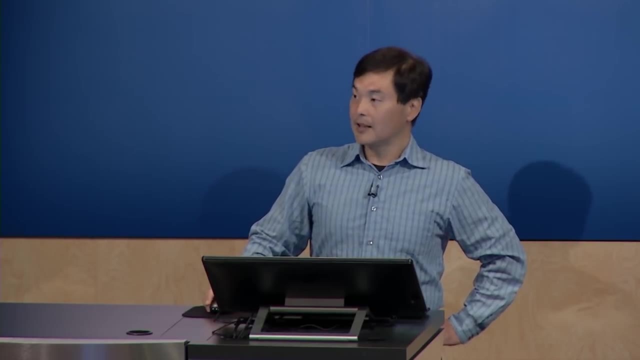 has been able to predict the test of time awards winner quite accurately, And that's actually the second thing that I would like to talk about. The ranking here is actually the full-blown search ranking, and it's not just based on citation counts. 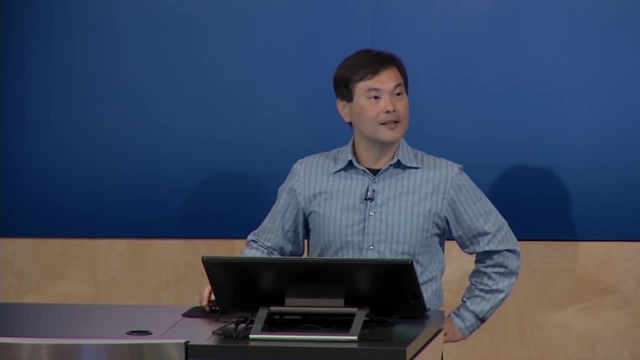 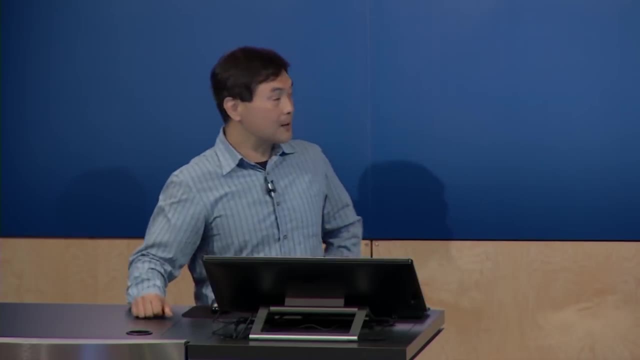 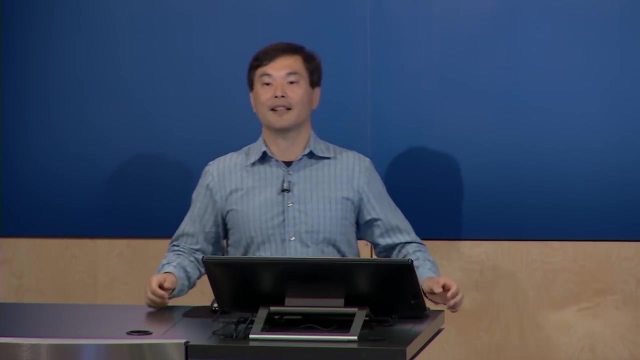 As you can see, the third search result has actually received more citations, More citations than us, And so. but the ranking algorithm here is actually also estimating the reputation of the citing parties and not just blindly count the citations. So I'll be more than happy. 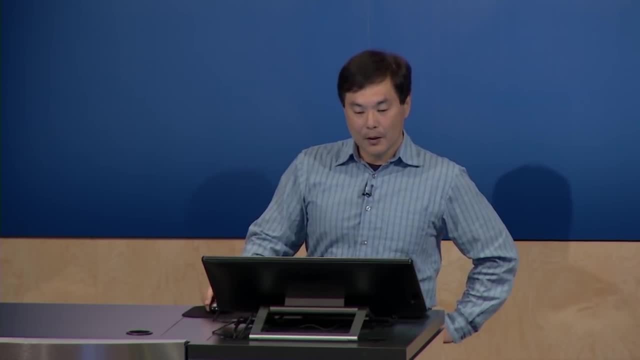 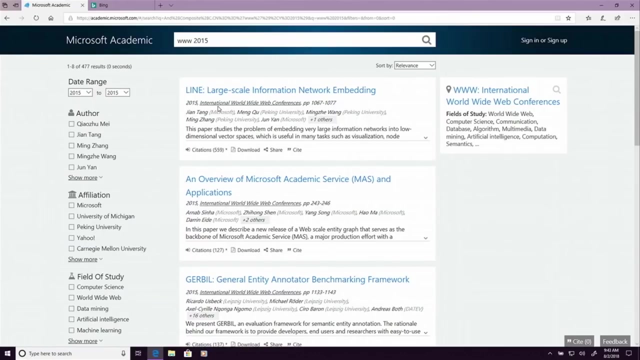 to talk more about it with you afterwards, Right? so if this trend continues, I'm predicting that in WWW 2025, this paper about a neural representation of a knowledge system is likely the winner of the test of time awards. And this paper, coincidentally- 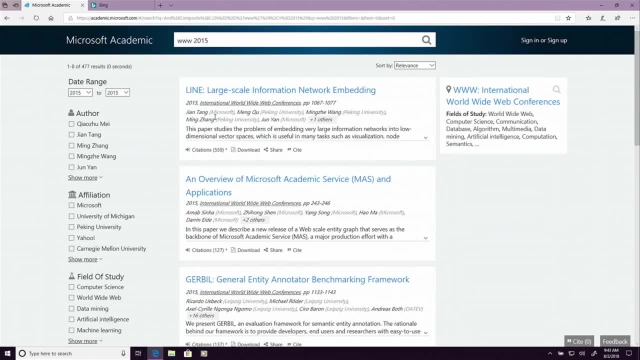 is from my colleague in MSRA, Jian Tang. Now, for many of you, speaking of Jian, who unfortunately has a very common name, and many of you who have a common name, to get your research results aggregated correctly on the search engine has been a challenge, isn't it? 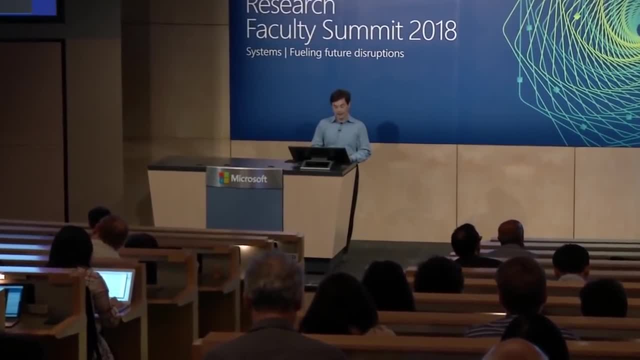 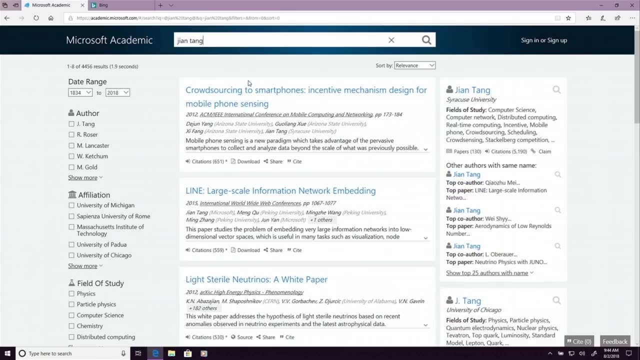 Right, so let's try it for my colleague Jian. If you try this with your favorite search engine- keyword-based search engine- you will see. well, yes, there are quite a few Jian Tang in the system and the results are actually intertwined together. 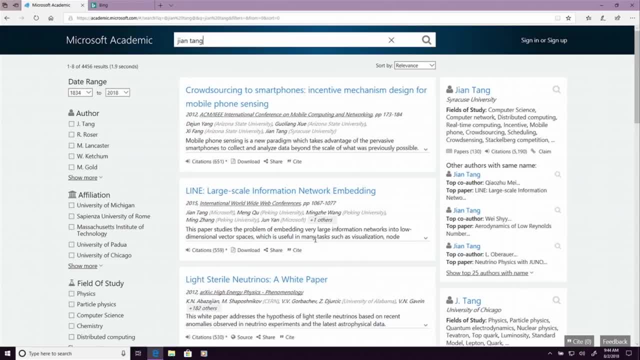 But because this system is sitting on top of a bin, we were able to use all sorts of knowledge, including your CVs and resumes published on the web, and to actually learn how to describe and disambiguate different authors. So, for example, in this system, 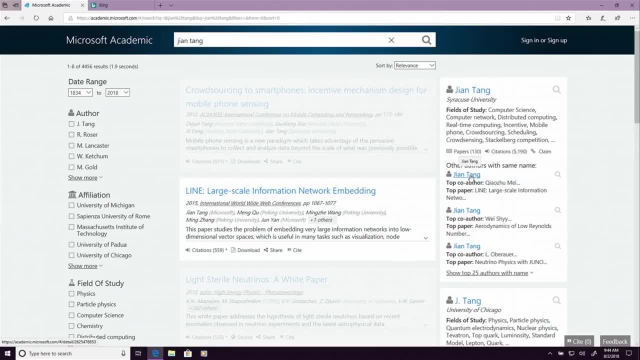 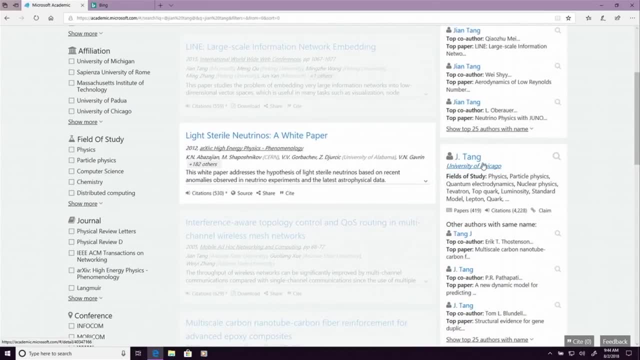 when you hover over different names internally, at the back end we actually understand which Jian Tang is which, and not to mention all sorts of other variations. Our physics colleagues like to publish their paper with only first, initial and last name, and in many publications. 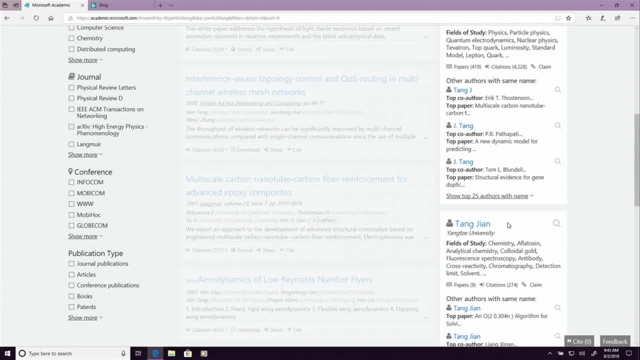 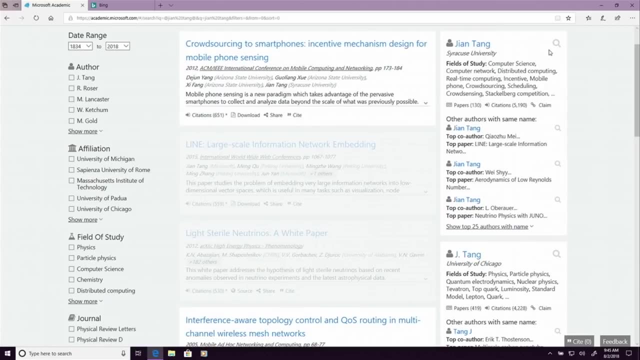 they actually observe the Asian convention by putting family first Rather than last, And so these are all different hypotheses we put in here, As I alluded. as you've already seen, you can just hover over it In this case. this is our colleague Jian. 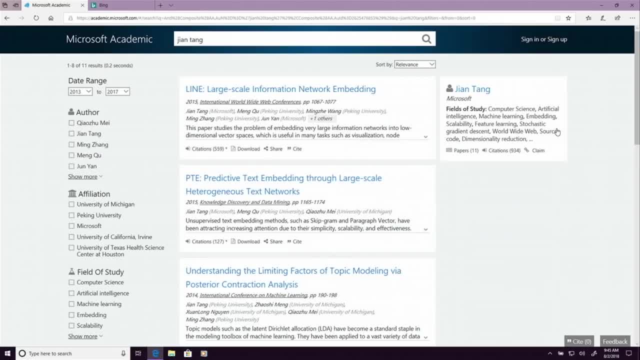 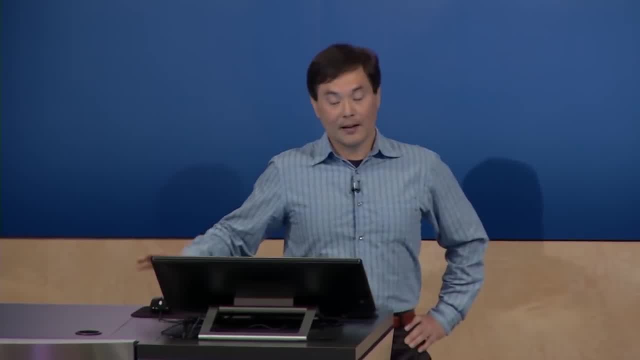 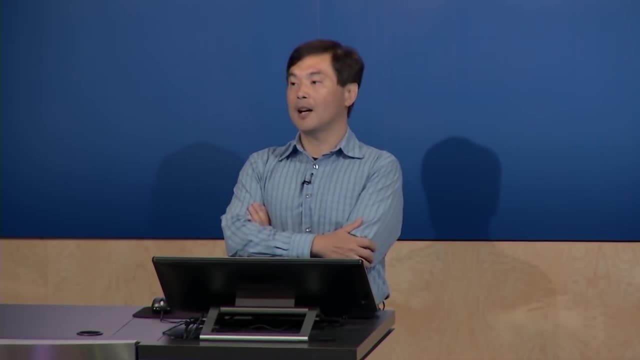 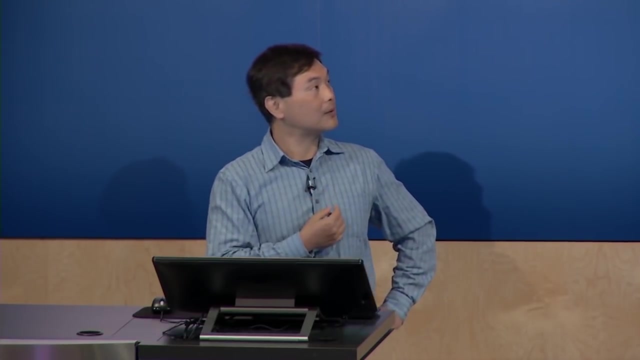 what I want, and just one additional click, Voila. All his work is aggregated correctly and showing here, So I hope this gives you a quick understanding about what the knowledge system can help us and how you can enrich the experience we have. And so let's now switch back to the PowerPoint. 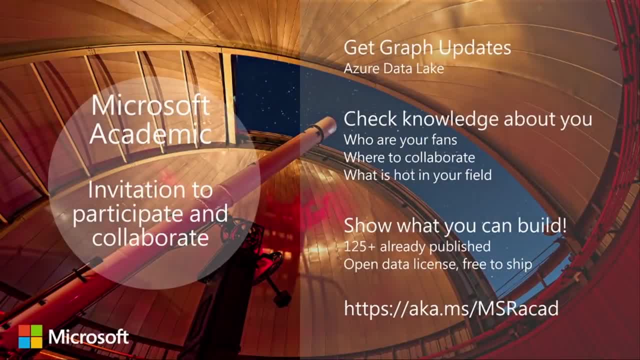 So, if you are interested, find this useful and interested, these are the resources we are making freely available to everyone. The first one is the graph, the data set. It's available through Azure, Again freely available to everyone. And then there's a. 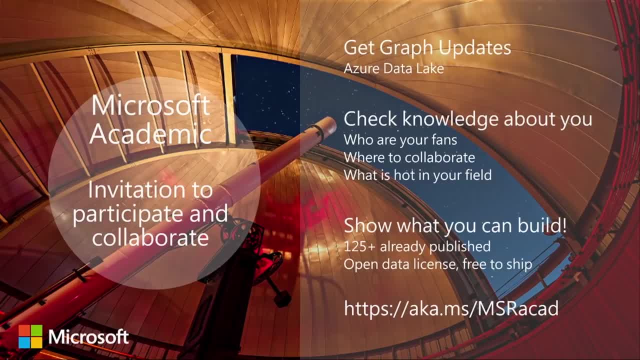 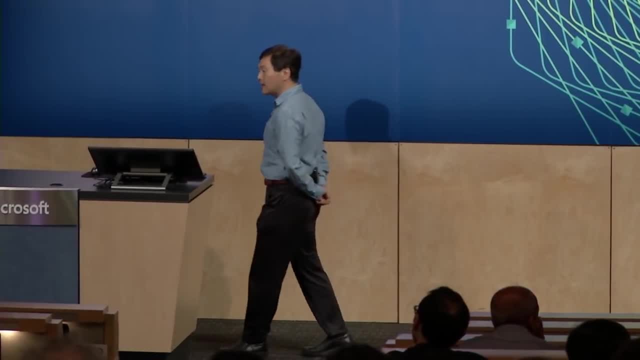 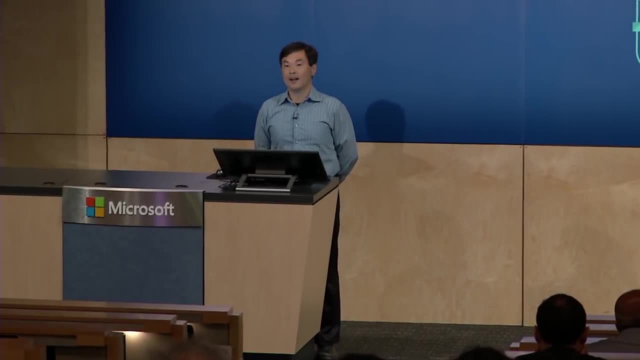 so in the same folder you will find a lot of open source tools that hopefully can actually jumpstart all these operations to deal with large data set and create knowledge systems. We encourage you to take a look and, as you see, we have already more than 100 systems. 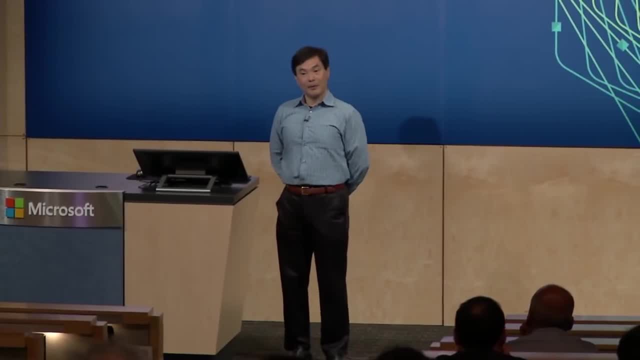 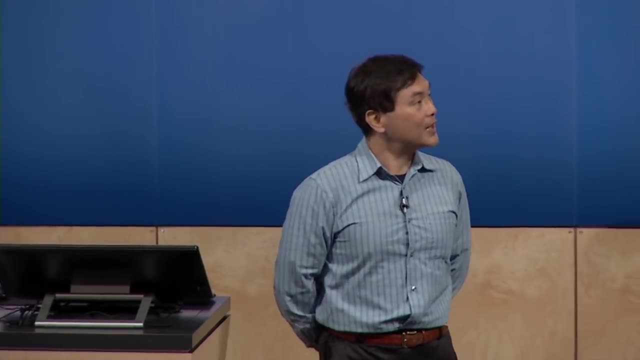 127 systems that are already published based on this data set. I invite you to take a look and tell us what you can build. More information is the URL: akams msrcat. With that. thank you for your attention and let me welcome David back. 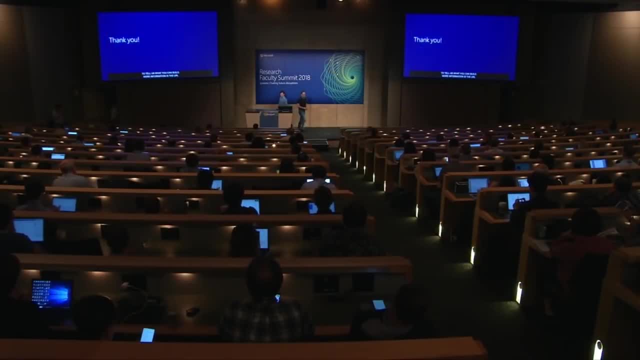 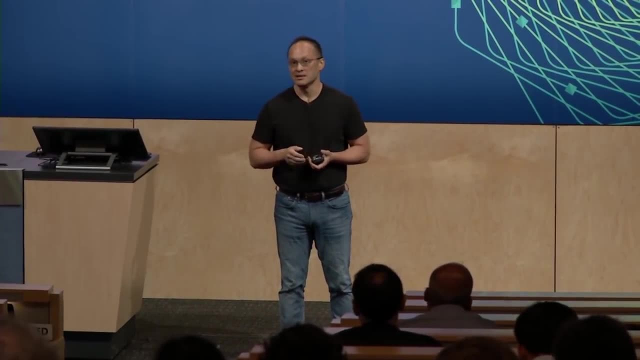 All right, thank you, Phonsen. Okay, let me wrap it up. If you roll back at the beginning, what we're seeing is this emergence of an appreciation for knowledge. Knowledge is going to push the limits of systems and AI. 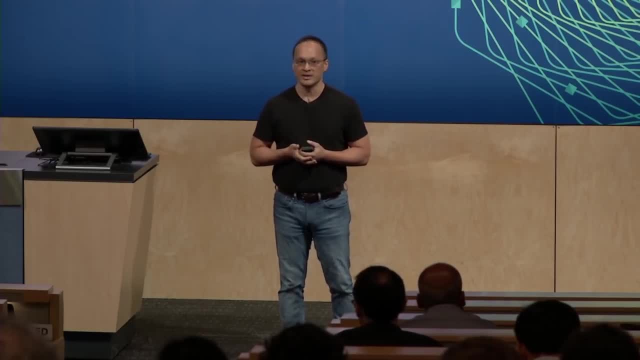 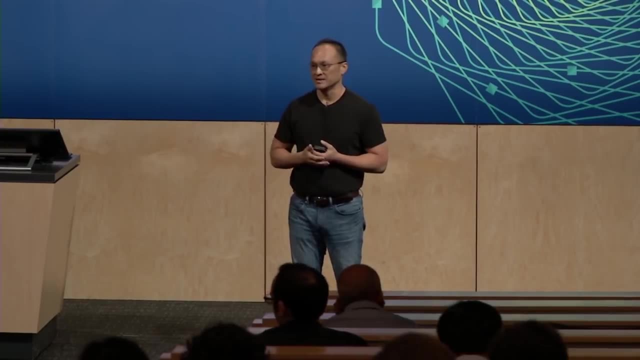 but it has a transformative effect in the way we think about products and we think about companies. And this is also a rich area where we're still at the forefront of that technology race and that technology push. And with that I want to really thank all of you. 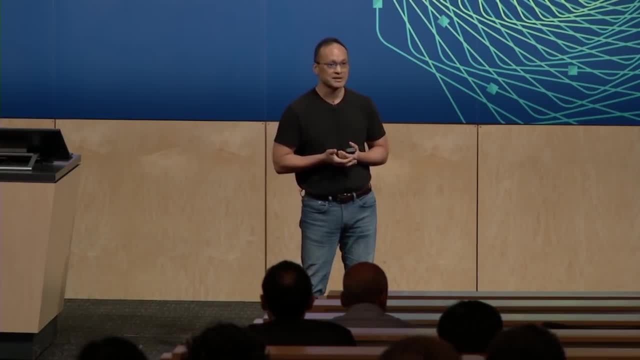 for your attention, your participation in the Faculty Summit. I'm excited that Microsoft is such a strong advocate for academia and for research, and we are looking forward to seeing amazing things from all of you and from our collaboration. So thank you, Thanks, David.